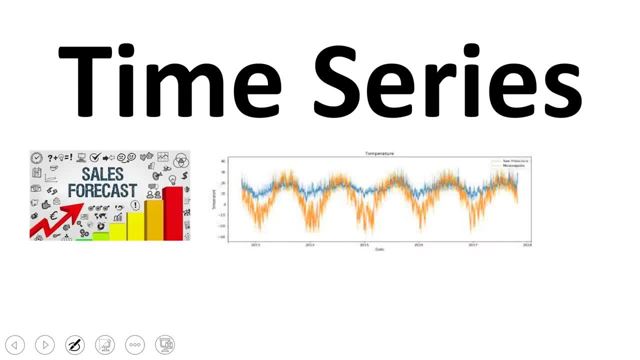 other applications for time, says: if you ask me, then we can say that we can use this for sales forecasting. we can use. ask me, then we can say that we can use this for sales forecasting. we can use. ask me, then we can say that we can use this to predict the temperature, weather. 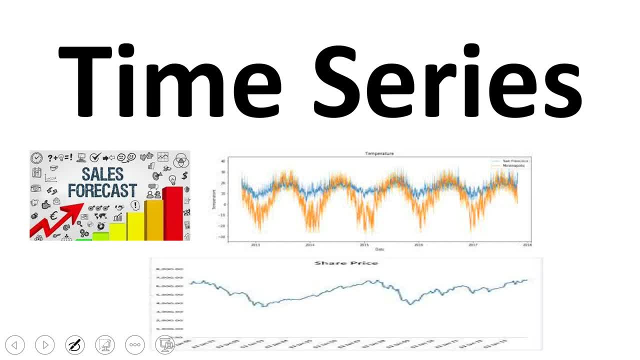 this to predict the temperature weather, this to predict the temperature weather, or whatever. it is okay. we can use this or whatever it is okay. we can use this or whatever it is okay. we can use this. to you know, predict the price of our. to you know, predict the price of our. 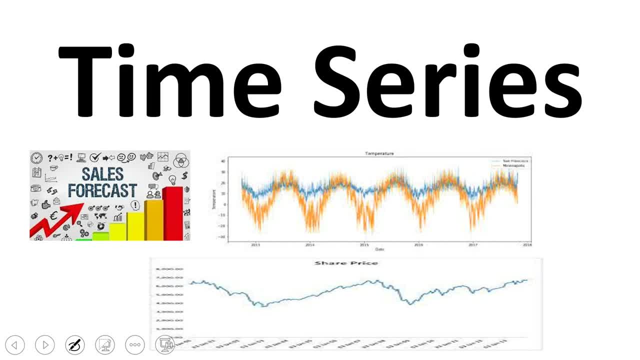 to. you know, predict the price of our favorite to stock, and so on. right, these favorite to stock, and so on. right, these favorite to stock, and so on. right, these are the images which I have taken from. are the images which I have taken from. are the images which I have taken from google? all right, so these are the these. 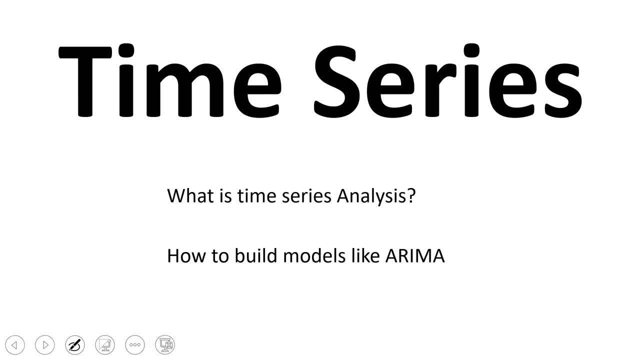 google. all right, so these are the. these. These are some of the applications or uses of time series analysis. In this series of video, we will be understanding what exactly the time series analysis is, what are the models that we can build on time series analysis, in time series analysis and. 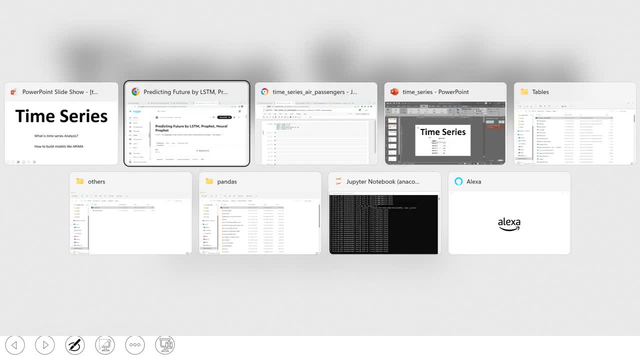 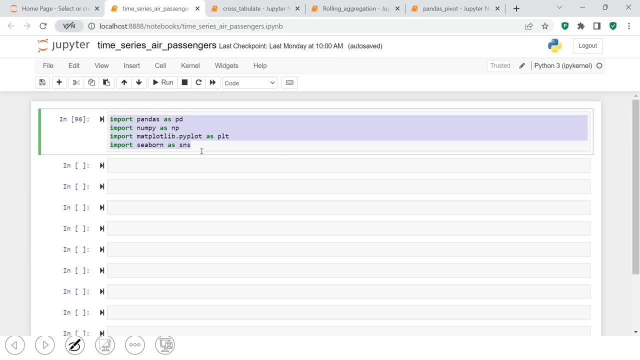 many more. Let me take you to the Jupyter notebook and try to help you understand with practical examples. So here, before we start, these are the prerequisites which I have already imported. I expect, or I believe, that you are already familiar with all these libraries. 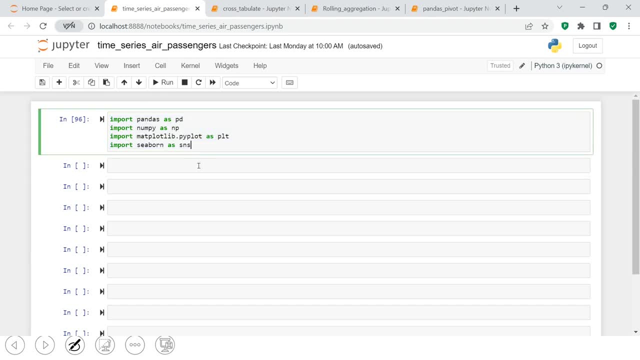 If not, let me know in the comment section. I'll help you with each of these libraries and or, if you want, you can find the videos tutorials for each of these libraries which are available on this channel. Now, moving forward, let's try to have a look on the data. 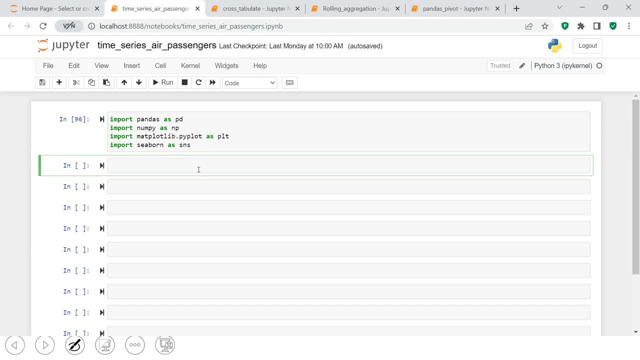 How to get the data In Seaborn library. Seaborn library also provide list of data sets. So how can we see What are the lists, Lists of data sets. for that what you can do is you can say set sorry, snskit data. 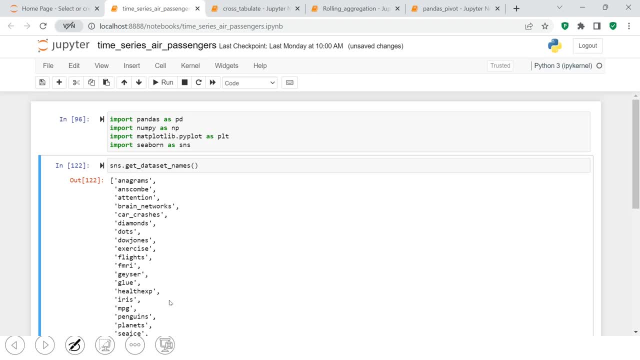 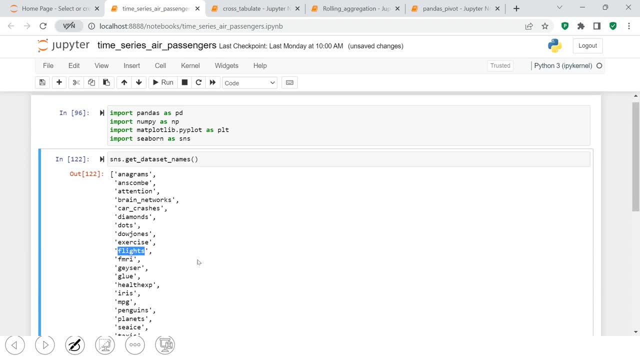 set names and call this okay. So this is what you get. This all are the data sets which are available into this Seaborn. okay, Now we will be taking this flights data. This is the air passenger data which I was showing you in the very first. 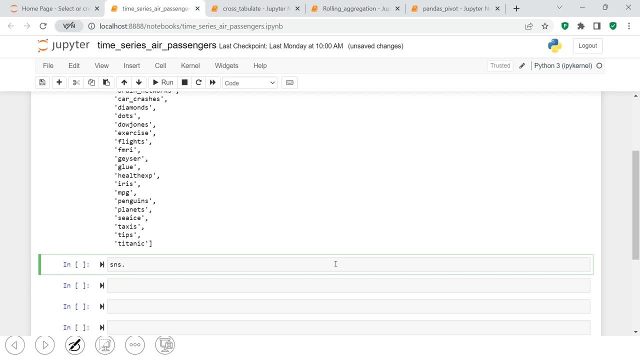 Now let's just try to import this. How would you import this? For that you're going to say: don't worry, you don't have to use pandas, because you're not going to import pandas. You're going to import that from Excel. 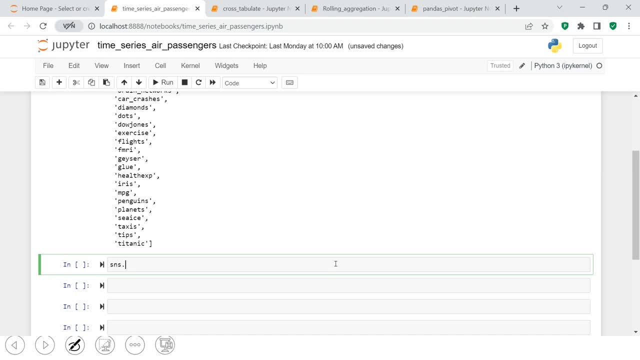 It is already available in Seaborn, We just need to load that. So here we're going to say: snsload data frame- sorry, data set- And in that you just put the data frame name and let's just see, we will put it in a data. 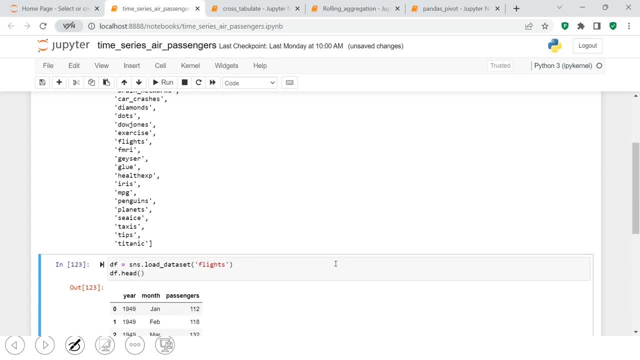 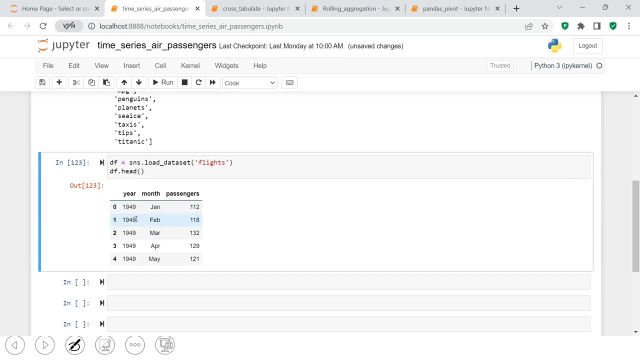 frame, and let's try to see a sample of this data frame. Okay, Like you can see, this is how our data set looks like. Here we have year column, month column and passenger column, So we need to convert it into one complete. 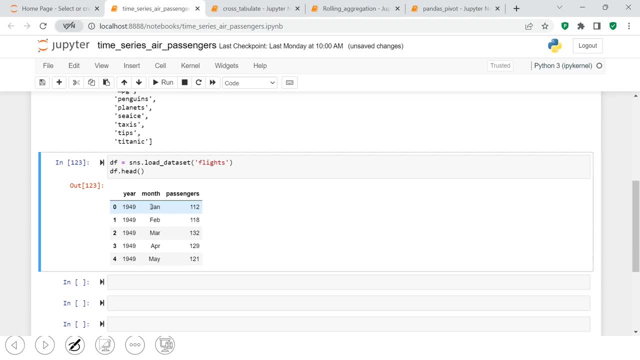 But the problem is here we have only year and month, so we require our day part also. So here what we will do is we will take one common date. For example, we will take first day of each of the month, because last day for each of 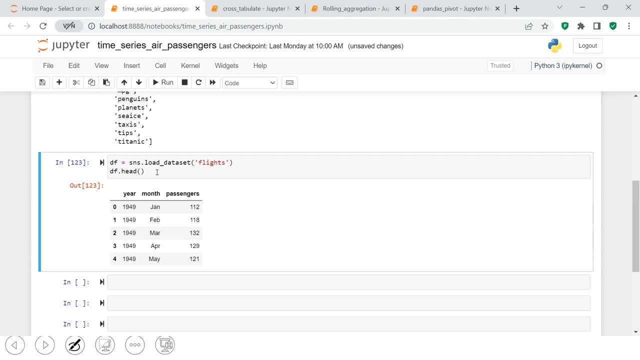 the month will be different. So we here, we will take first day of each of the month and we will try to combine them all together, all these three together, And then we will have one date column. So let me give a name to that. 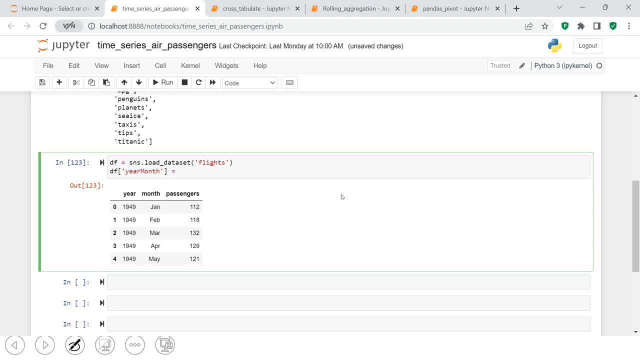 Let me create a variable. I will call it year, month, and into that I'm going to concatenate or combine all these three things. So first thing which I need is day, part dash plus. here I want to use year column. But the problem over here is: this is integer variable. 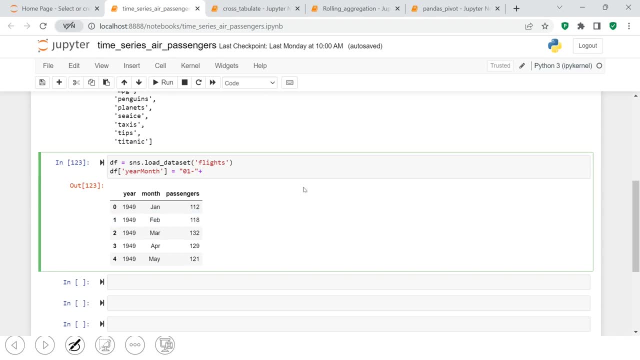 Okay, So we need to convert that into string and then concatenate. How can we do that? So, for that simple, you just need to put the variable name and then just say as type into that. You can just call, you can just say SDR. 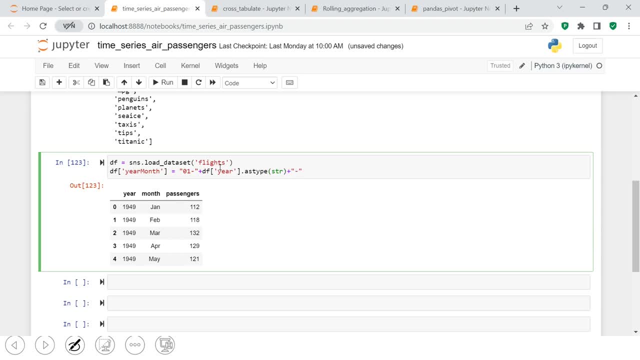 Okay, This is it. Then after that, you need to put a dash. I will be putting a dash and then the next thing, I will again repeat this same thing for month column. Now you might have a question. that month column looks like you know text, but this is not. 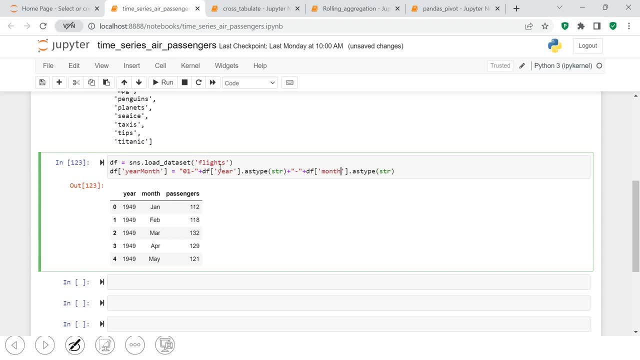 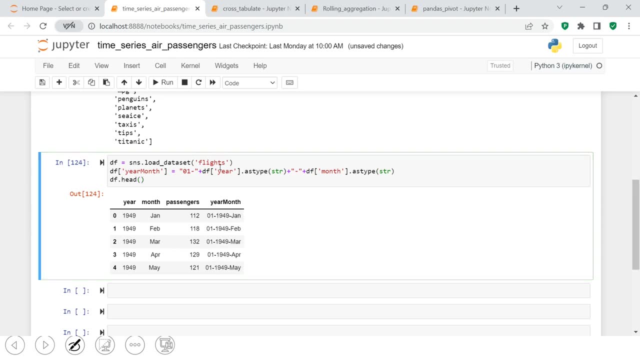 true, That's the categorical variable. Okay, That we also need to convert into the string and then we need to, sorry, use that, Okay, So that's it. Okay Now, if you see, this is what we get now, like you can see over here. 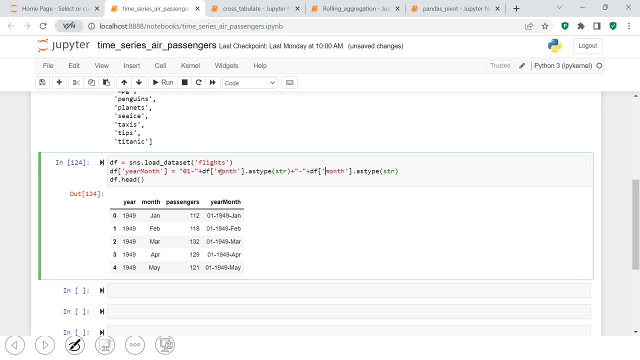 Okay, Let me do it differently, And over here I will call it here. Now this looks much better, All right, So this is how, um, but the problem over here is this particular column which we have just created is not the date time column. 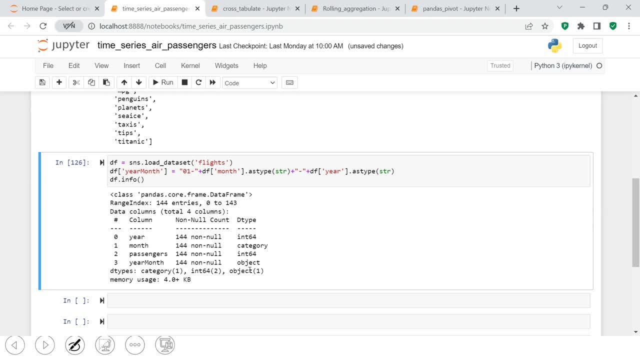 Okay, It's not the date variable. So in that, in that scenario, we might have trouble, We might struggle handling Or, uh, handling this variable or doing the analysis. So what I'll do is I'll just use one function. 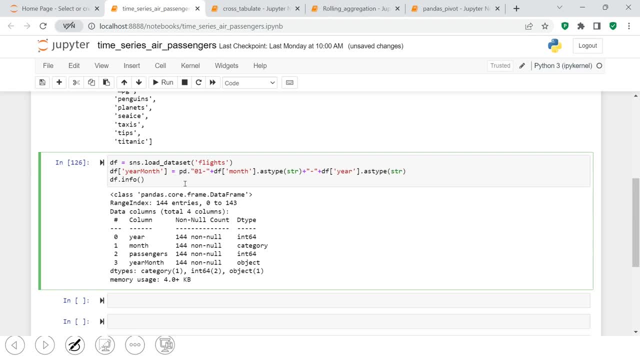 Let me call that, you know, BD dot two date time And let me just put all these things inside that Now we have this intake time format And, if you want to have a few on this sample data, this is how this looks like. 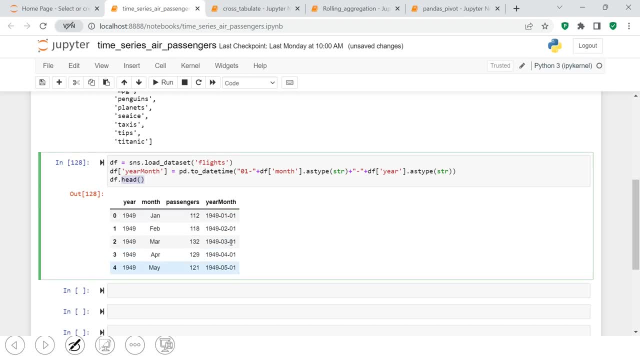 Okay, Now what I need to do is I'll be converting this particular column into Index. Okay, I'll make it index so that it will be easy for us to handle this. Okay, If you want, you can continue. uh, in the same way, but here for the convenience I'm. 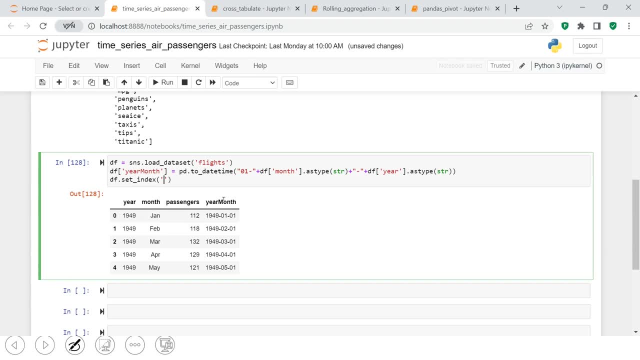 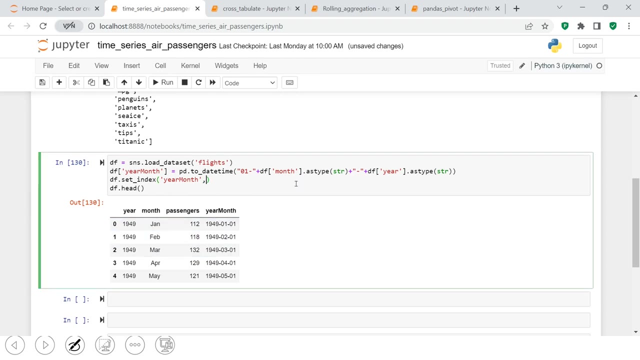 just doing this DF dot set index and you just supply the column which you want to use as index. Now let's just see. this is how our data looks like. Let me just call it DF dot head. Oops, Here You need to say in place. 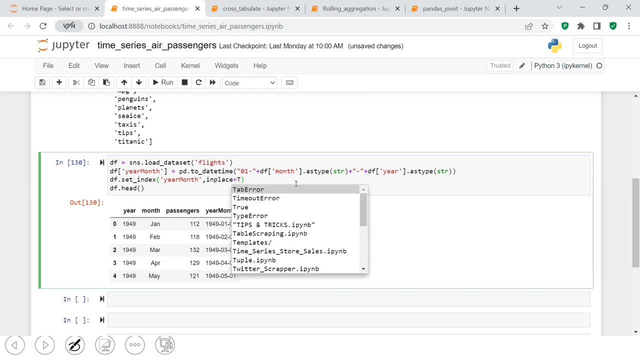 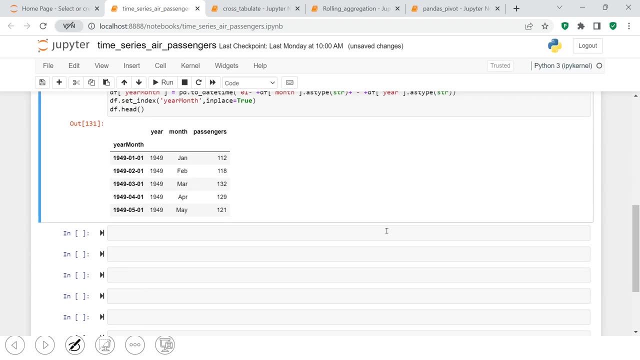 True. True In place Equals to True. All right, Now, here you see. we got this data. Now let's try to plot this data on a line chart. Okay, How can we do that? Let's say: SNS dot line plot. 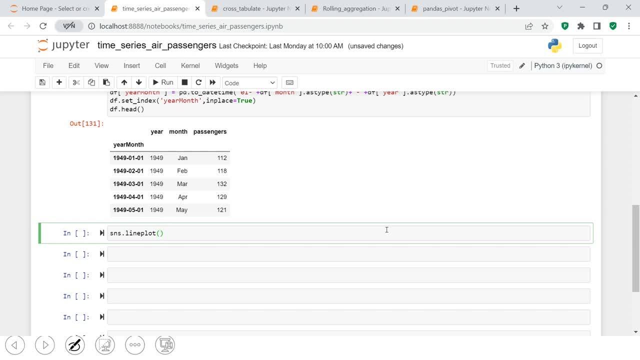 I've created a separate series for on seaborne and matplot also, So if if you're someone who is new to visualization in Python, I highly recommend you to check that out. Okay, So SNS dot line plot. Okay. 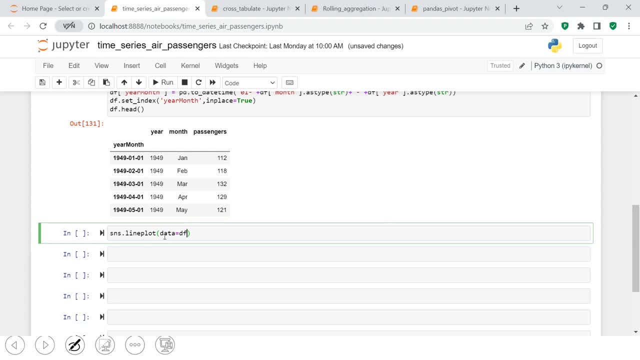 So what I'm going to do is I'm going to- I'm going to apply this data frame name here in the data frame. Okay, Uh, in data argument or parameter I'll just apply the data frame name, And then, on X axis, I won't be use DF dot index. 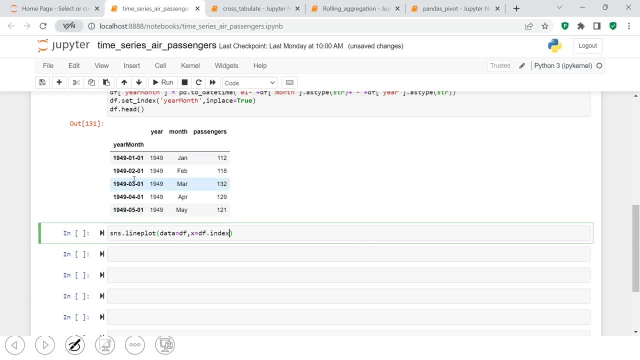 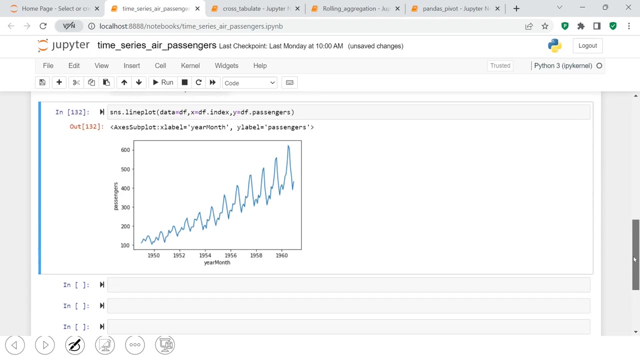 Okay, DF dot index. I will use this particular column. Okay, See how simple it is. now What next? on Y column, I will be using DF dot passengers. All right, Now let's just plot this So you see this kind of graph we are getting. 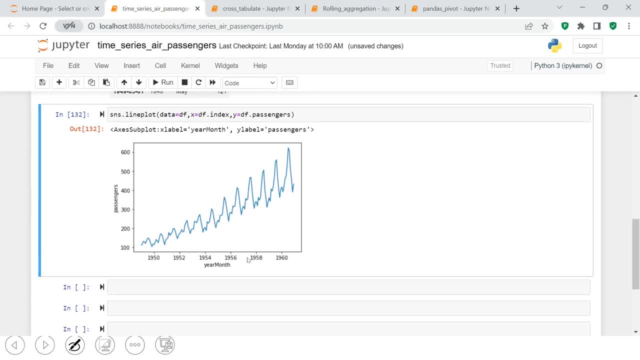 When you observe this particular graph, what we see is it shows us are trained. Uh, why it is called trained? because if you, um, I mean, there is one word which you got, okay, Which is trained, What does that exactly mean? 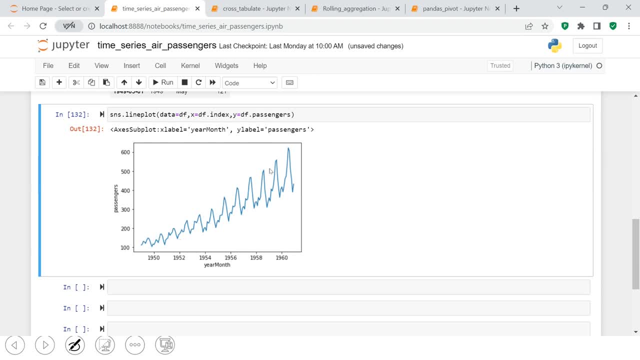 Other than trained. you also see up, down, up, down, up down, by a specific time, That is. that's something which we call, as you know, seasonality. We can say seasonality, right, What all these key terms are. 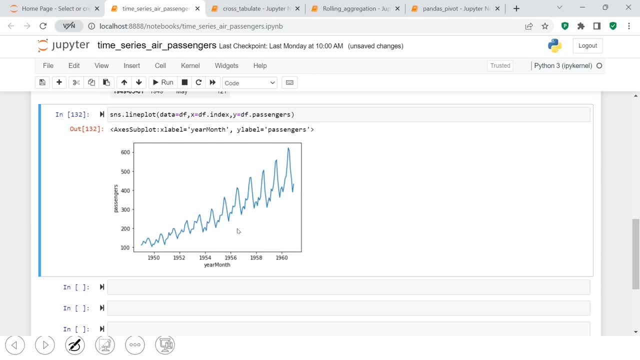 These are nothing but the patterns. So, in time series, in time series, usually whatever patterns that we get, usually those are classified in four categories. Okay, What are those four categories? Let me take you over here and try to help you understand. 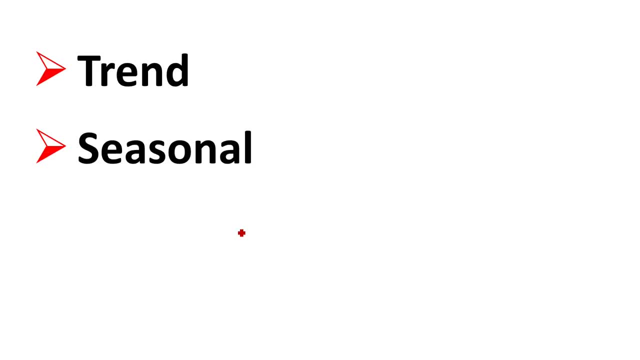 So those four categories are trained, which we just saw, then seasonal- This was also combined with the trend, then cyclic and then irregularities. Okay, Let's try to understand one by one trend: It's something in the data. When you plot the data, you will see either the dependent variable is growing or it is. 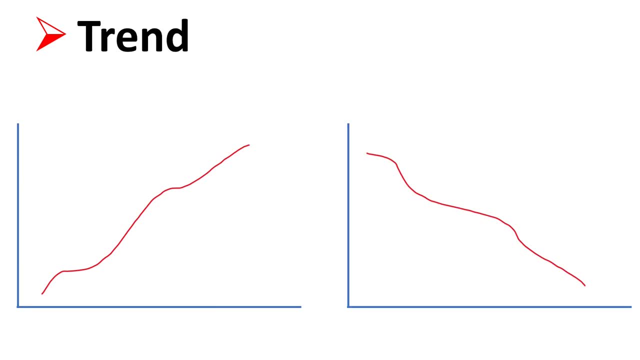 decreasing by the time. So you see over here, this, uh, this variable is growing. It's, it's increasing by the time, in accordance with as you grow by the X axis. it is growing upward here, It is downward. 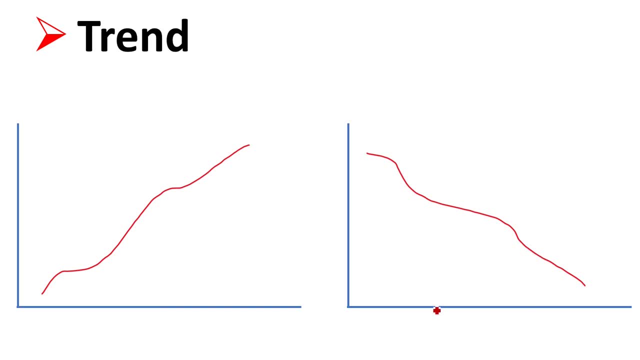 Okay, It is decreasing by X axis as, uh, as the time grows, this particular dependent variable is decreasing, Okay, So this is kind of trained pattern. We also called it component of time series analysis. Okay, This is the trend one. 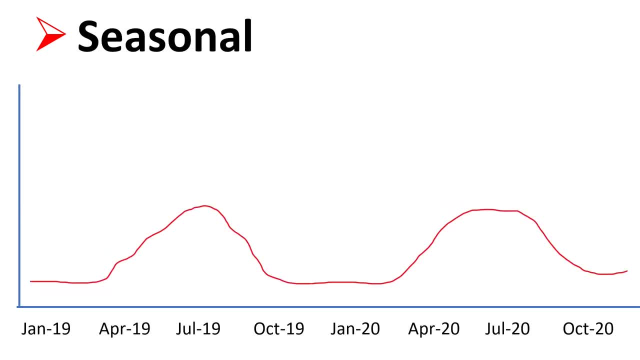 Next comes the seasonal one, For example. have a look on this particular chart. What you observe is this: before I explain you, let me tell you. this is: let's consider- this is a completely hypothetical data for ice cream. So if you observe over here, the sales of ice cream is starts to increase by the beginning. 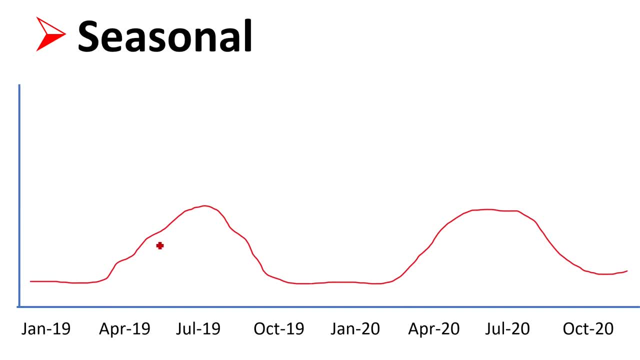 or before beginning of April month, and it keeps on growing, and then it starts falling near to October and then it keeps- uh, you know, on the lower label till again at the beginning of April. Then again it is coming down. Um, it goes up and then comes down at the start of October, and so on. 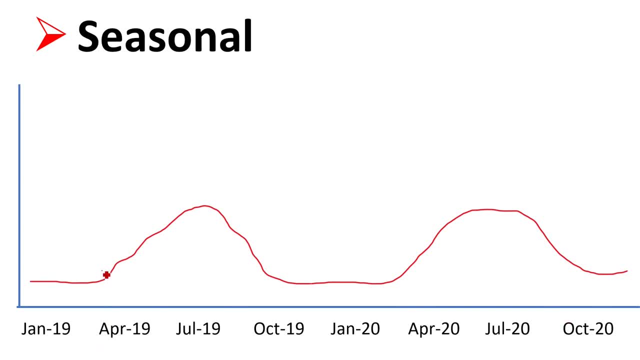 Right, Okay, So what do you observe is, from April till October, beginning of, from starting from beginning of the April till starting of October, this is growing. Okay, This is growing. So what do you see is, by the time, if you see, there is a fixed pattern, 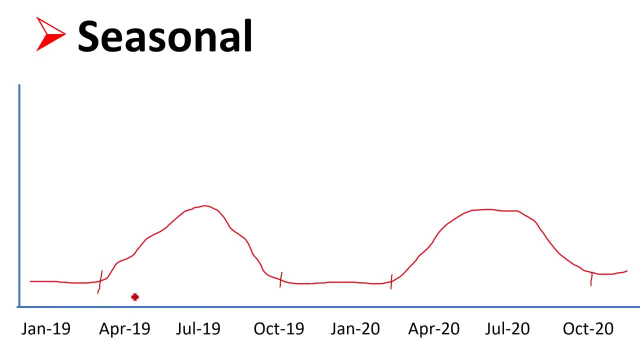 So in India, usually we have summer season during this time. So what we observe is during the summer the sales of ice cream is increasing and you see there is season, So during this time, this timeframe, the sales is increasing. So whenever dependent variable either increase or goes down for a specific time period, right, 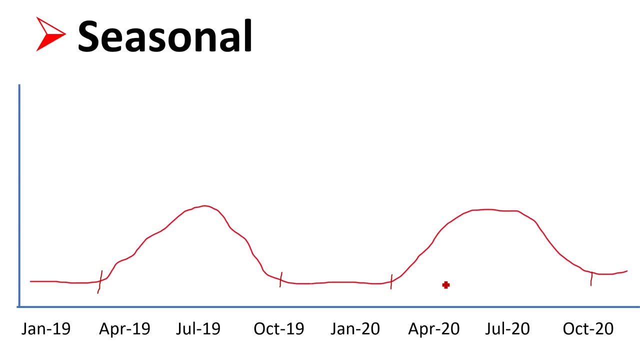 And that repeats and that gets repeated on a fixed frequency. That's where we call it seasonality. So every year in the month of April to October the sales of ice cream is increasing and then it's falling. That's why we call it seasonal. 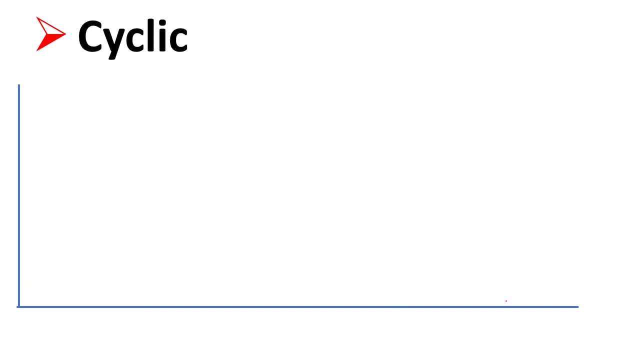 I hope that it is clear to you. Next comes cyclic. Cyclic is something which starts and then continued for some time, keeps continue for some time and then it goes away, And then there is no fixed time when it will come again. Right? 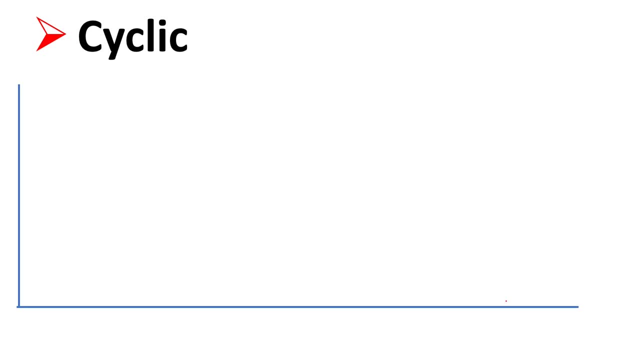 It could be positive or it could be negative, also In terms of negative, if you take example of recession, COVID. So what happens is you get this kind of trend right, This kind of trend, For example, if you take a recession. so there have been multiple times when there was a. 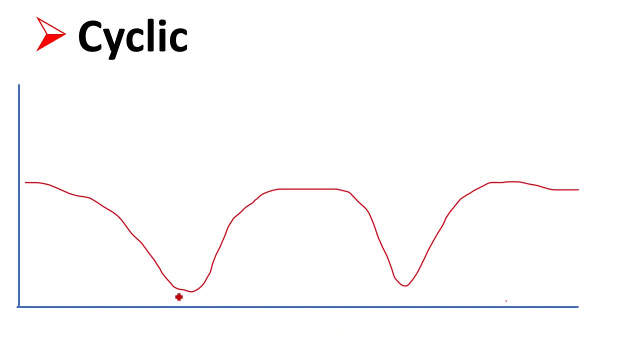 recession came right, So it will come, and then it will remain for some time and then it will go away. Then everything will remain smooth Then again at certain point. I hope that it never comes, but it may come right. 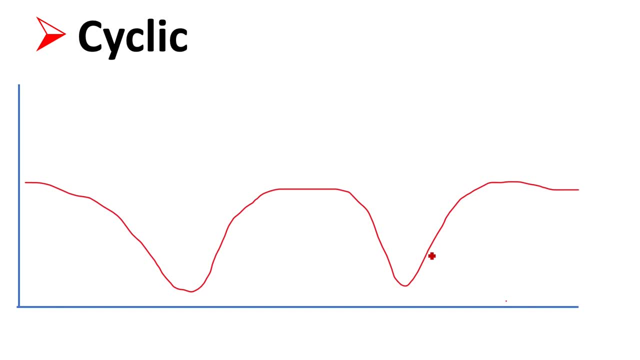 Again. then that will go and it will remain for some time And then again the things will come up right. Same thing happened in the COVID also, So those kinds of things called cyclic. usually this happens, you know, in case of depression. 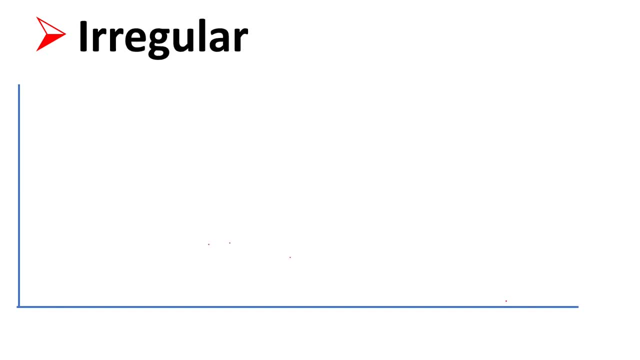 recession and all those things. Okay. Then comes irregularities. So, in case of irregularities, you don't find any kind of pattern into it, right, You don't? you don't see any pattern in the data. We we also call it noise in the data. 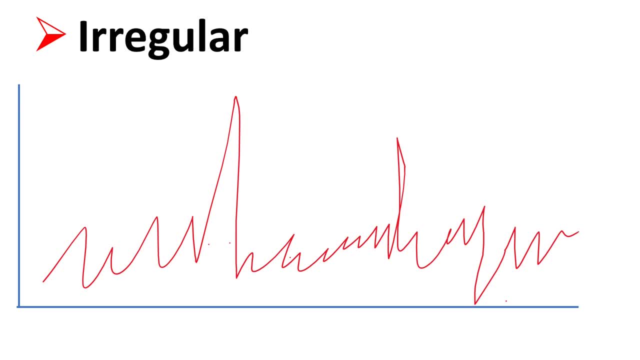 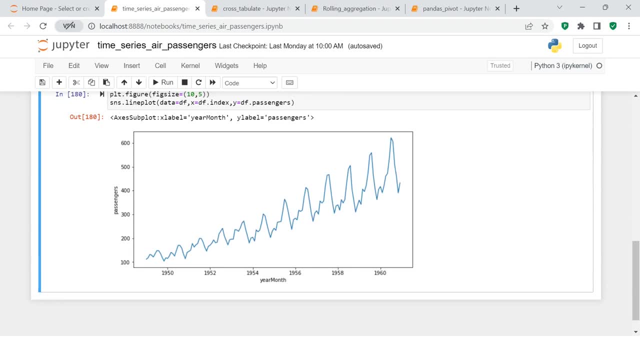 And we try to avoid this in this scene. In this case it becomes really difficult to you know, do the analysis. By now we have understood the component or patterns which we generally find in time series And over here on this graph. 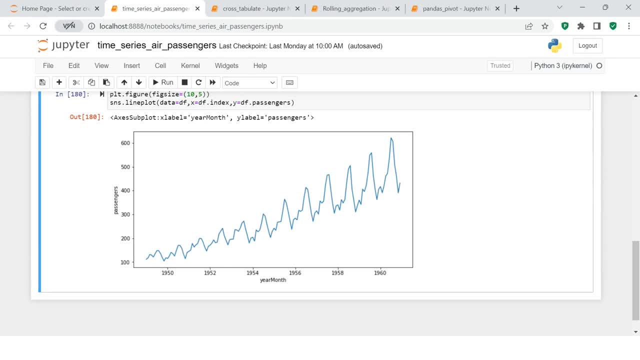 We can clearly see that there are two patterns into it. One is seasonality And then the other one is straight. Okay, So if you just start building model on this particular data, that might turn out to be biased or maybe some sort of overfitting and something like that. 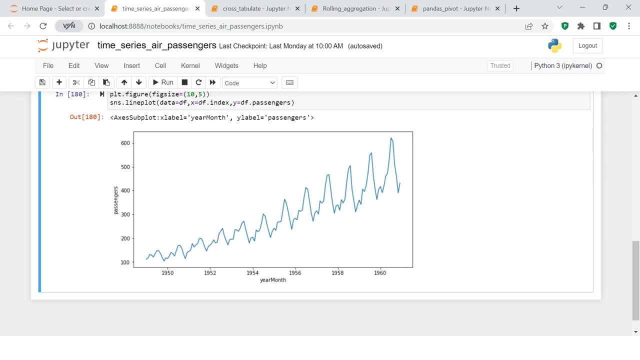 Okay Means the model may not turn out to be accurate. because? why Here, Here? Because, if the data is clearly showing, as the time passes, the number of passengers will increase no matter what Right. So the model will not give the correct output, may not give the correct output. 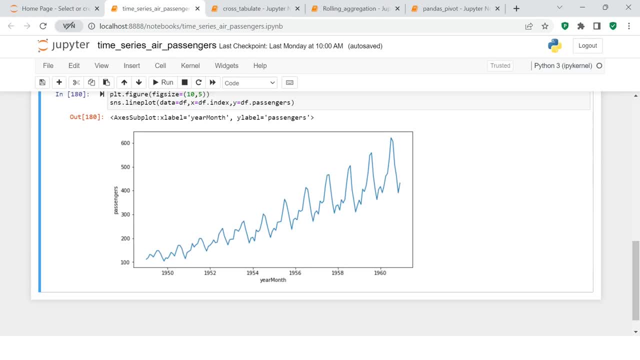 Okay, So how to fix this kind of thing? So before start to build the time series model, we check out the suitability of the data. How do we check the suitability of the data? So for that, We figure out stationarity, Right. 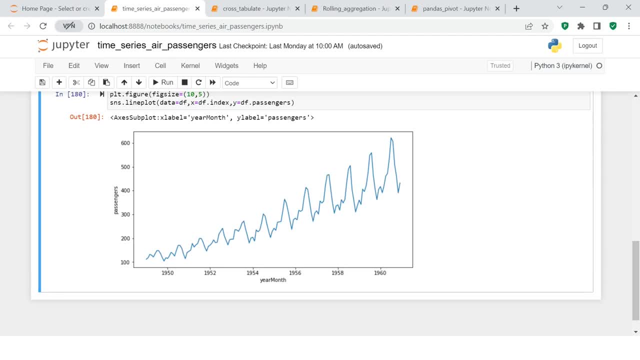 How stationary, whether the data is stationary or not. Now you got a new keyword, which is stationarity. What does the stationarity mean? Let's understand that And then we will understand how to figure out whether the data is stationary or not. 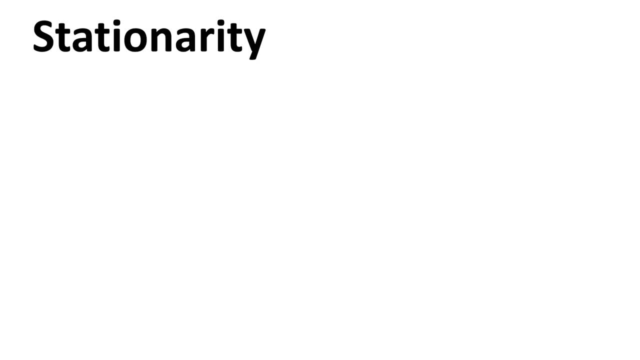 So stationarity means simply, if I put it in very simple layman term, then it clearly. it simply says- I wouldn't say clearly or what It clearly says, sorry- It simply says that mean and variance or covariance or standard deviation of the dependent variable. 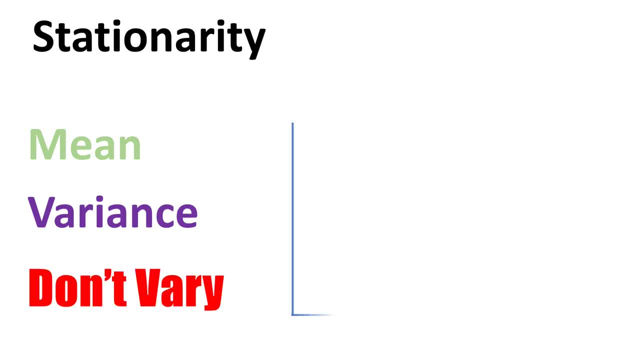 don't vary by the time. What does that mean? Let's say that if we plot our data on this X and Y axis and if we are getting this, the data is completely hypothetical. If we get this kind of data, this is a stationary. 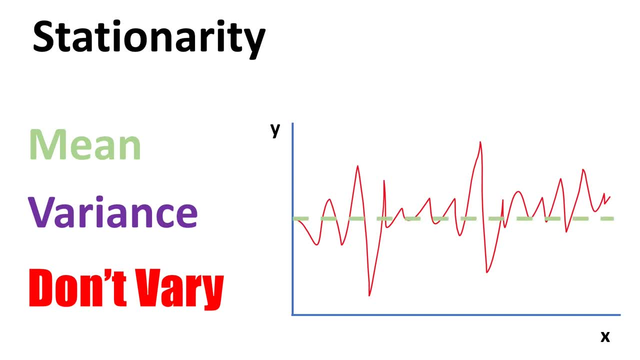 Why? Because you see this mean It is traveling alongside the X axis, which remains. it's a straight line. you are getting for the mean. So that means the mean is remaining constant by the time. X axis represents the time and Y is representing the dependent variable, whatever it is. 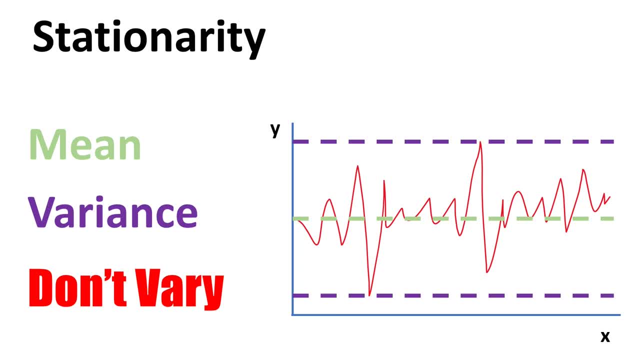 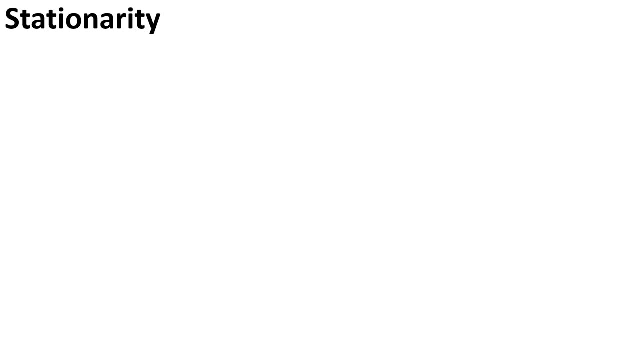 And now, if you see the variance, that is also traveling alongside the mean or X axis. So here we clearly see that the data is stationary. Now let me show you some more examples Here. So I have taken some of the images, which I have directly taken from the Google. 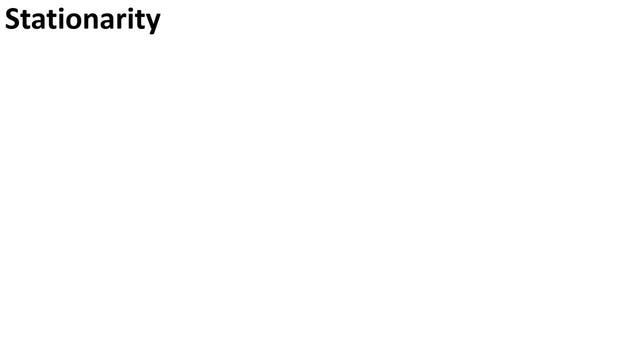 This was very much suitable to explain it, So the credit goes to Google itself. Now, here you see. this is same as what we just saw. Here you see, stationary mean and stationary variance Means here: mean and variance. both are stationary Means. both of these two things are constant. 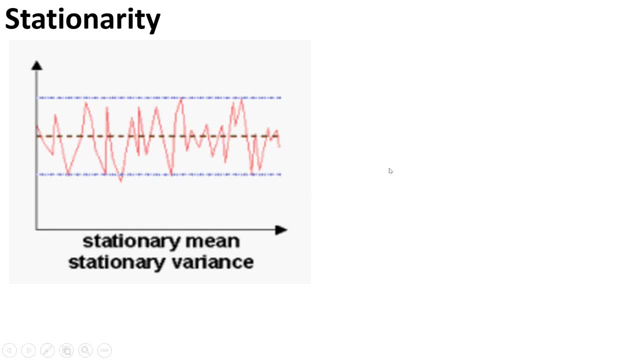 That is not changing by the time. Okay, If you see, the line is straight. So mean of this dependent variable remains approximately same and variance also remains same. Now let's have a look on the different image. What do you see over here is the line in the center represents to mean, and these two blue 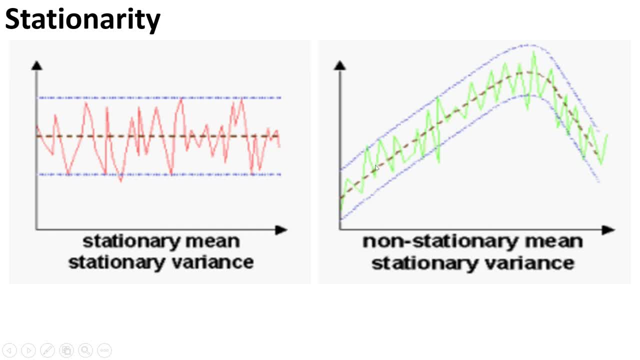 line represents to the variance. So mean is not constant. If you see it is, first it is trending. It is showing you a trending pattern. First it is increasing and then it is falling. Okay, You can also consider it as a cyclical. 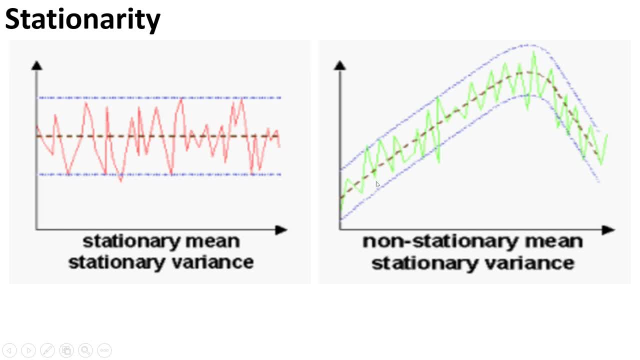 Okay, But what do you see is variance that remains constant. This increasing and falling line doesn't show that variance is not constant. This is alongside the mean, where you see the variance is constant. Okay, Variance is constant, but the mean is not. 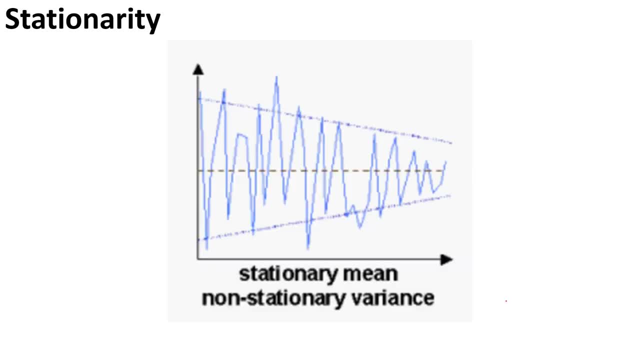 Now let's have a. if it is confusing, let's have a look on another image here. What do you see? This means mean is constant. That means mean is stationary, but the variance, the top and bottom line, are not constant. 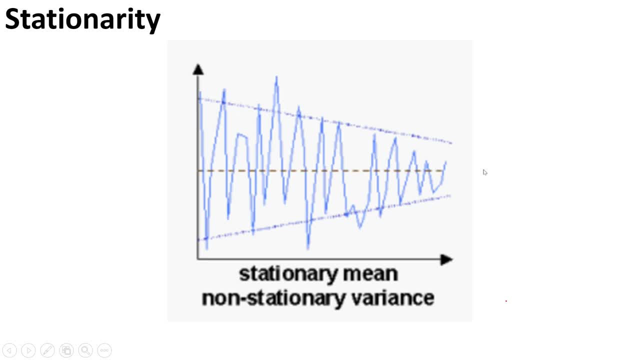 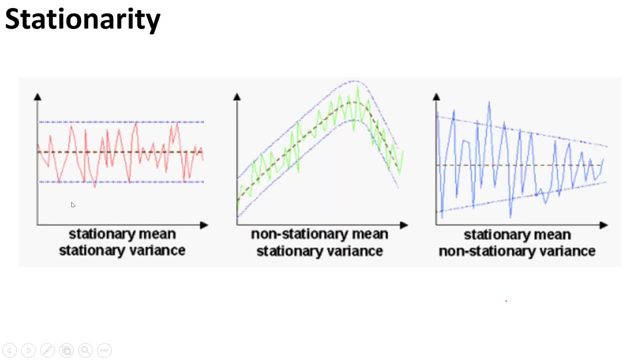 You see, initially it is more than it is reducing. Okay, So that means the variance is not stationary. If we put all these three image together, this is what we see. The first one is stationary, where mean and variance, all both of these two things are. 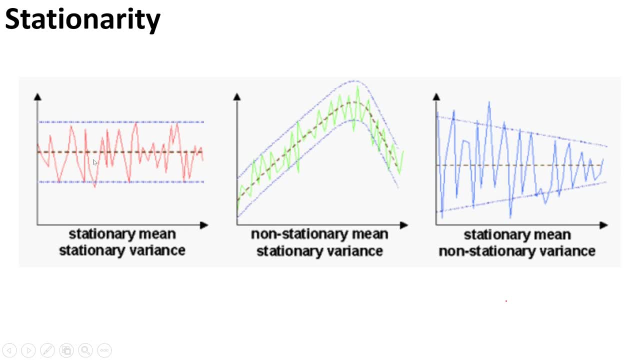 traveling alongside the x-axis. That means both of these two things remain constant by the time. Okay, In the second one, what we see is the mean is non-constant constant, but the variance remains constant, So that means this is also not a stationary. 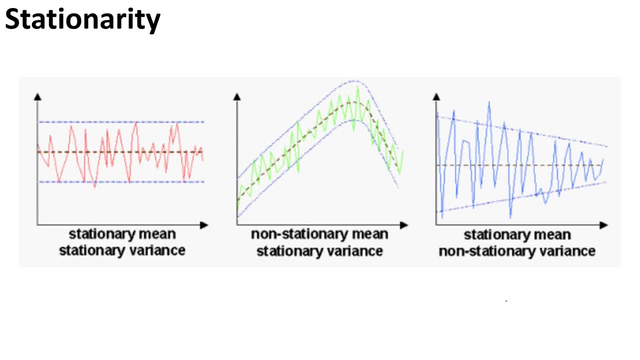 This one is also not a stationary By now. I hope that it is clear to you what stationarity is. In case, if you have confusion, put that into the comment section. I'll explain it in a separate video Moving forward. how to check the stationarity of data. 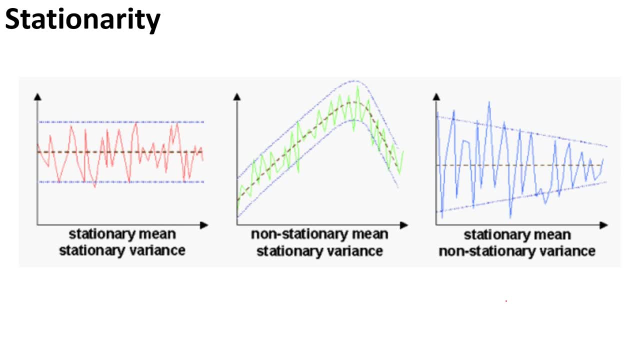 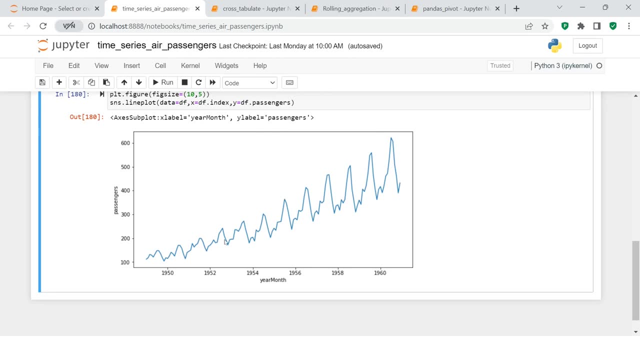 How to specify, how to you know, validate whether our data is stationary or not, though, by simply looking at the graph. when you plot the graph, and if you are able to, there are four patterns which we learned in the previous video. those four patterns we find in the 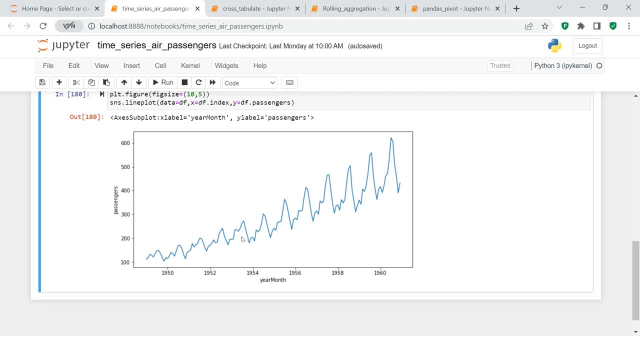 time series, right? So if you see I'm trending and cyclical, trained or cyclical work to train cyclical and seasonality. these were the components, The pattern in time series. So if you see, if the plot is either trending or it's seasonal, then that means it's stationary. 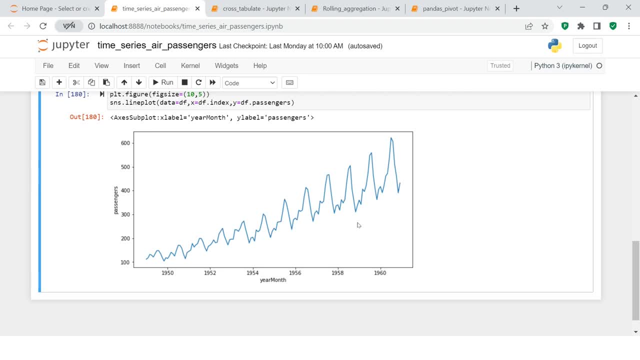 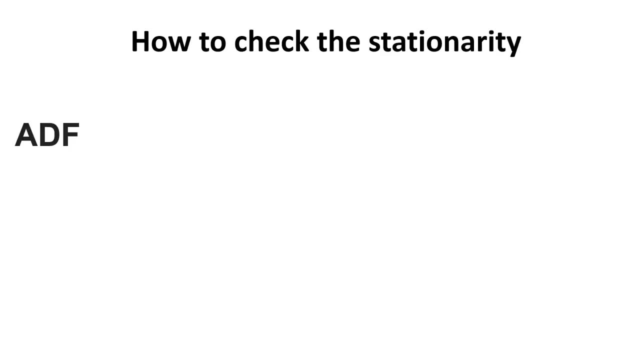 But still, if you want to specify that more particularly, how do you do that? So for that, there are two. mostly these two ways are used. Number one is ADF. What is ADF? Sometimes it is also called ADCF. 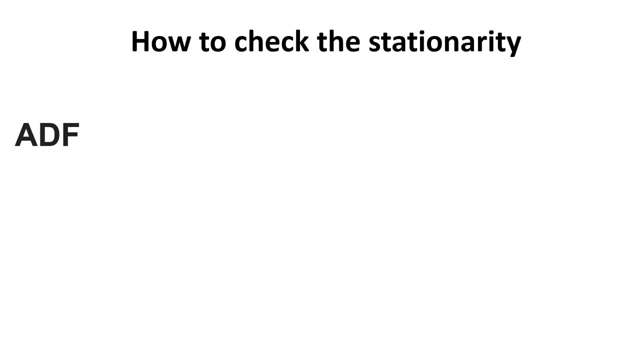 Not, sometimes somewhere it is where you would find that it is also used as ADCF, but the meaning remains same, which is augmented Dickey-Fuller test. Now there is a Wikipedia page for this. You can check that out to have the detailed understanding. 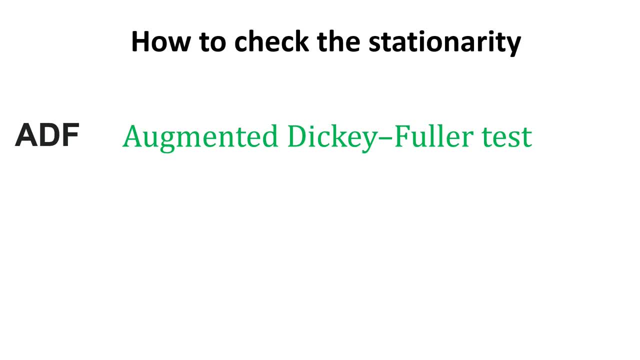 I'll provide the link in the description section And this augmented Dickey-Fuller test in this. what we do is we completely deny that, whatever the data is, we completely say that the data is not stationary. That's the null hypothesis we will take. 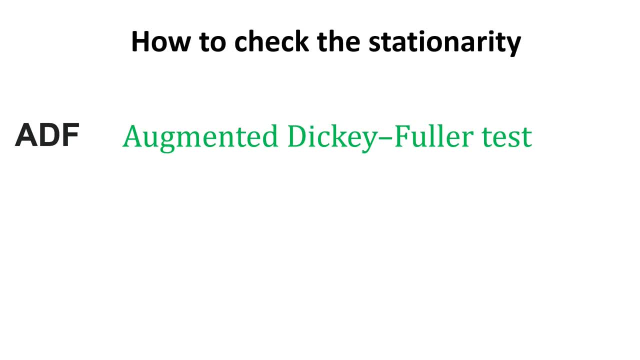 And then we will do this test, Which is Which will specify, or I mean this ADF or ADCF test either will reject or accept the null hypothesis, right. So in beginning we will set our mind that the data is not stationary. 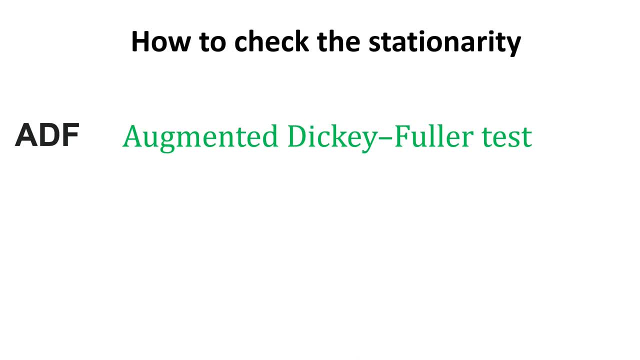 And then we will do this test to specify whether the null hypothesis can be rejected or accepted. Then what is the output? How do we specify this? So out of this test we get these two values: test statistics and critical values. So if you get- there are other values also which we get, but primarily if you see test. 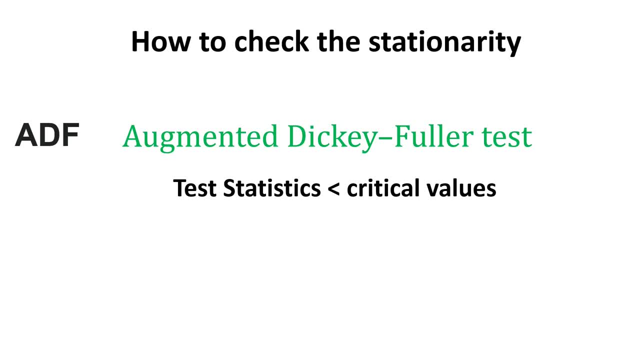 if test statistics is less than critical values, you can clearly see that the data is not stationary. Okay, I'm sorry. here I made a mistake. I should have to say: if test statistics is less than critical values, then we can say the data is stationary. 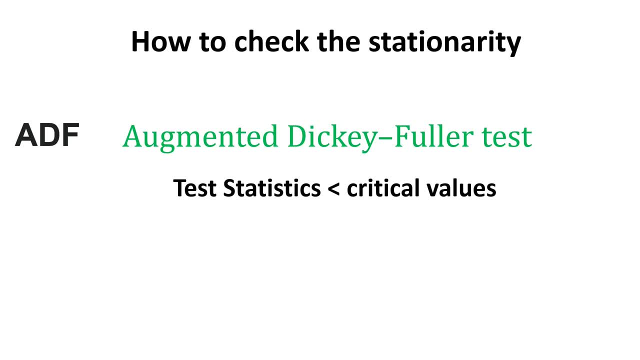 Okay, If it is not, then the data is not stationary. So, basis on this, we can either accept or reject the null hypothesis. Okay. The second test is which we can perform is rolling statistics. In this we simply take the rolling mean or rolling variance or standard deviation, and 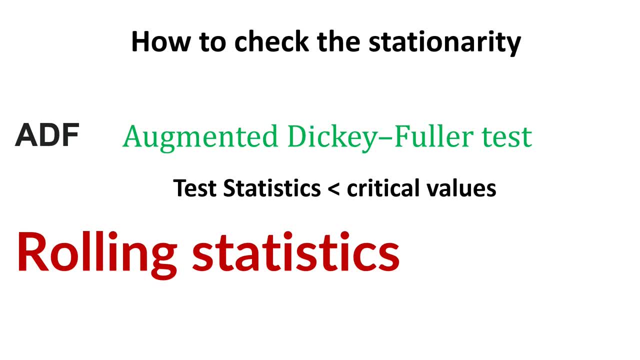 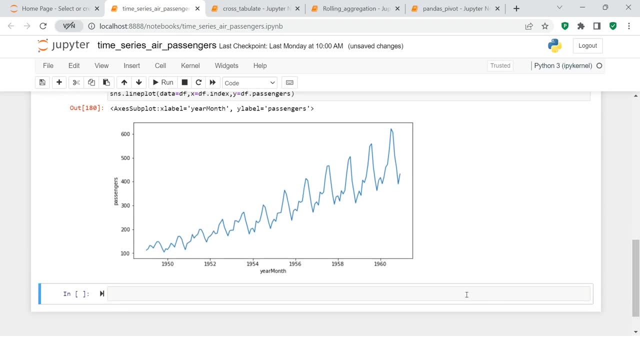 we will plot that, And this is the simplest one and provides the best clarity. okay, By visualization. All right, So now lots of talk, let's go to the Jupyter notebook and try to do this. Okay, So first let's start with the performing: the rolling statistics. 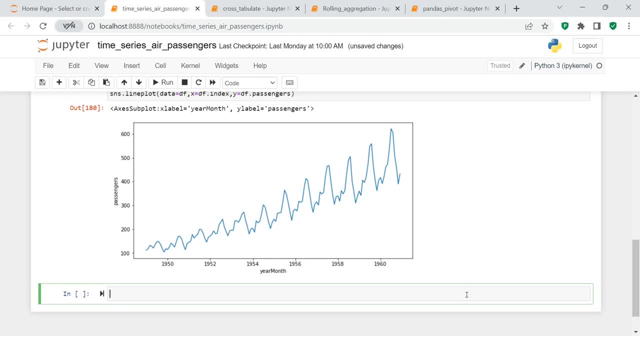 What we can do is: let's try to create a variable in our data frame. Let's call it roll, mean, And into that, what we're going to say is dfpassengersrolling, And here you need to specify a window. And what does window means? 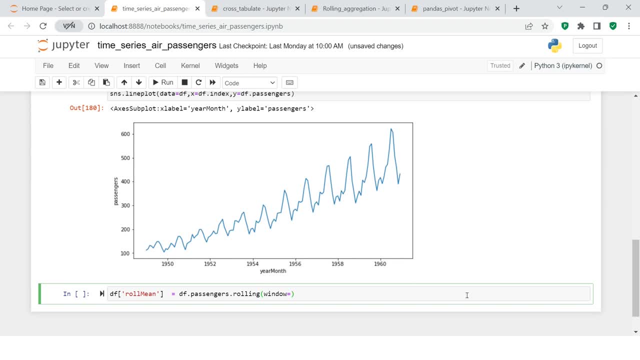 Window means by how many months or by what timeframe you want to roll the average. Now, if you want to understand rolling mean or rolling statistics, there is a separate video which I have created, link I'm giving in the description section. You can just check that out. 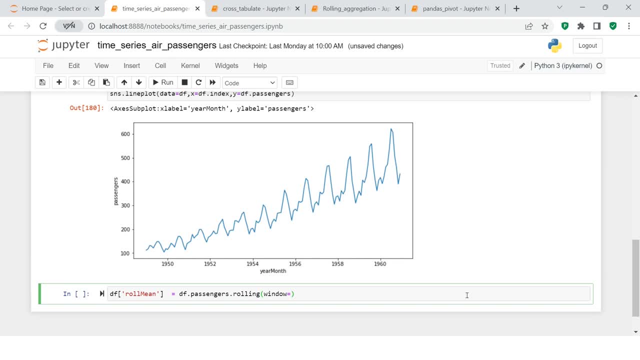 If that clarifies it, is okay. If not, let me know into the comment section. I'll make a separate video. So here I want to roll the average by 12.1.. Okay, So I'll simply say 12, and because here I'm going to create the mean, 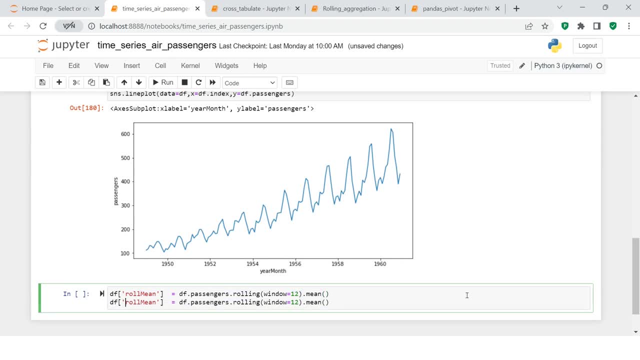 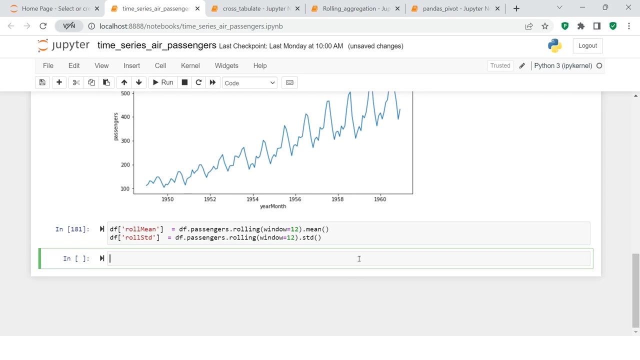 So I'll just say mean, this is the simplest way of doing this. Now there is another variable for standard deviation that I will create and I will say std, and here I will just change it to std. All right, We are done. Simple. 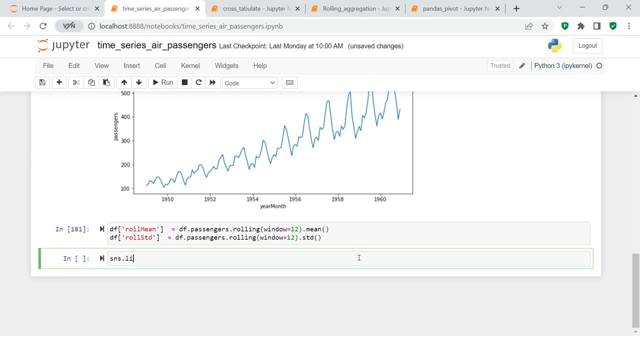 Now let's try to plot this. Okay, So the first data set which we are going to plot is line plot And into this data It goes to tf, where on x axis I'm going to plot the, on x axis I will plot index, because 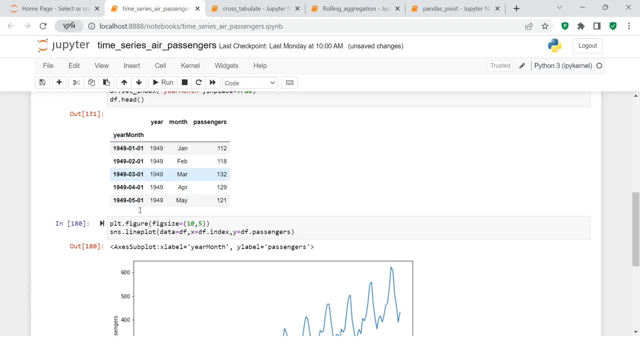 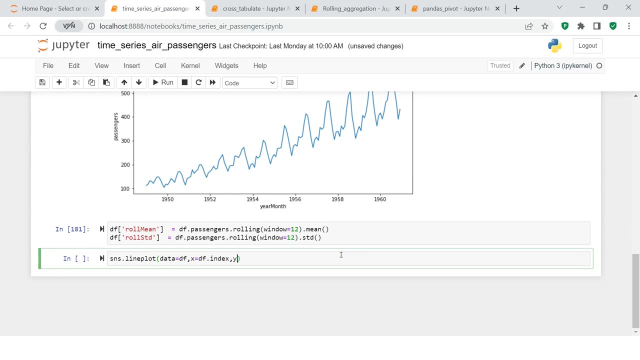 index is the column which has time, right, You see over here. then the second one on y axis. I'm going to plot passengers on y axis. I will just say tfpassengers. All right, we're done. So here it is exactly same. 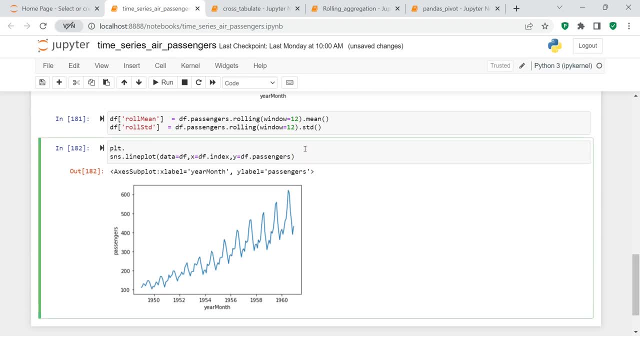 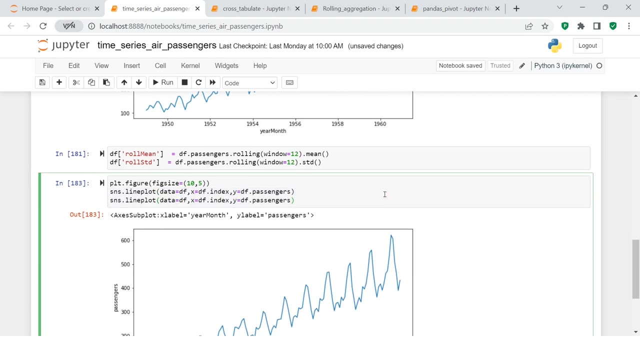 What we got previously. Let me specify the image size also pltfigure, and into that you can just say figure, fix size and just let's just give the dimension so that it will look a little better. Now let's plot the mean also here. 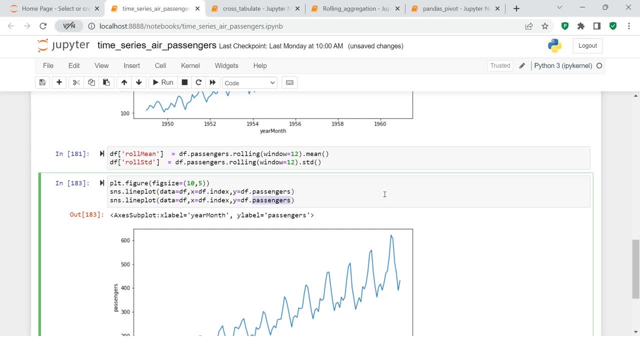 I will just say sorry, here I would say role mean this variable. Okay, Now The next one. This is standard deviation Std. Sorry, This should be std. No, it should be role std. This is All right. 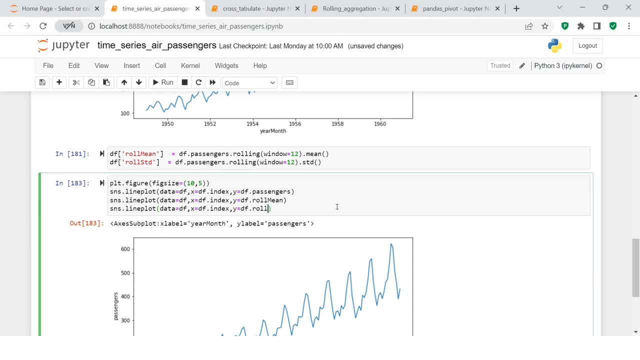 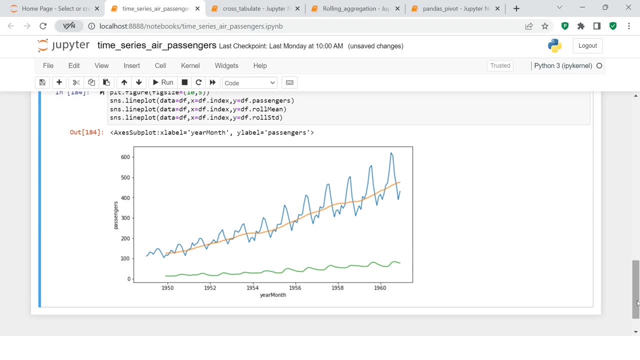 So we are done over here. Now here what you see, if you remember from the previous example here you see, this line represents to the rolling mean. This orange line represents to the rolling mean, This green line represents to the standard deviation. 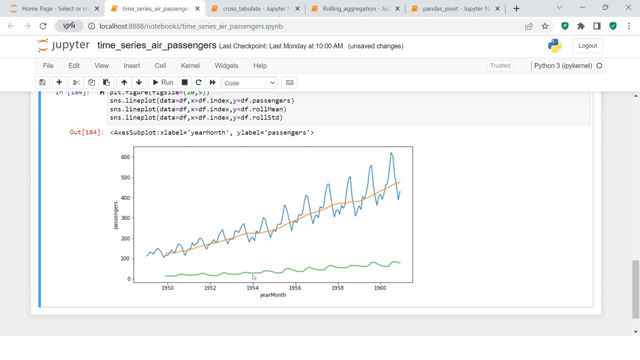 Okay, Rolling is standard deviation. So what we see is standard deviation is approximately. you know, stationary, That means it is approximately constant to the timeline, right? But if you see the mean, that is not stationary, that means it is not constant. 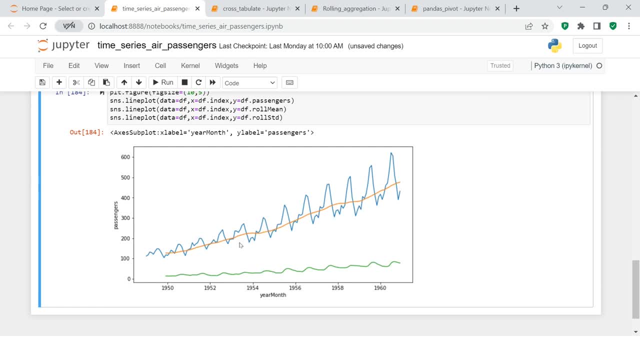 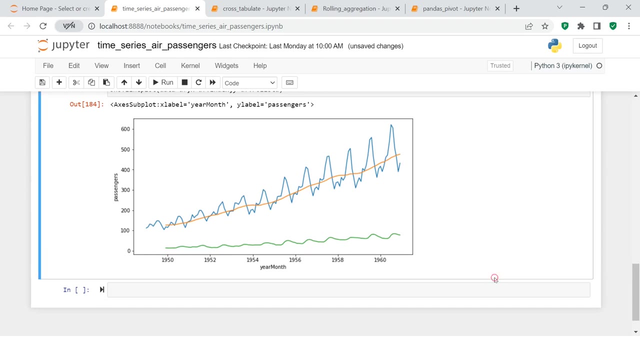 It is trending. rolling mean is also showing the trending pattern. trend pattern. Okay, It is increasing by the time, which means our data is not stationary. Now let's try to perform the second test, which is nothing but the ADF test. 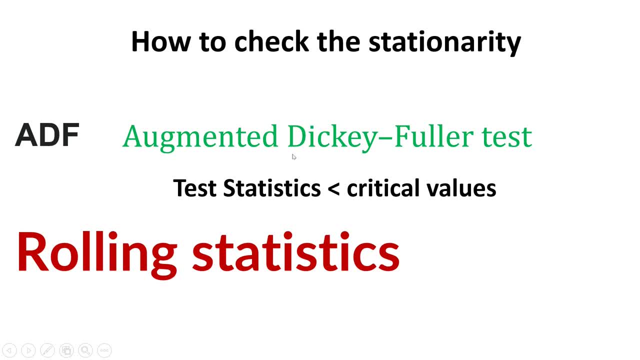 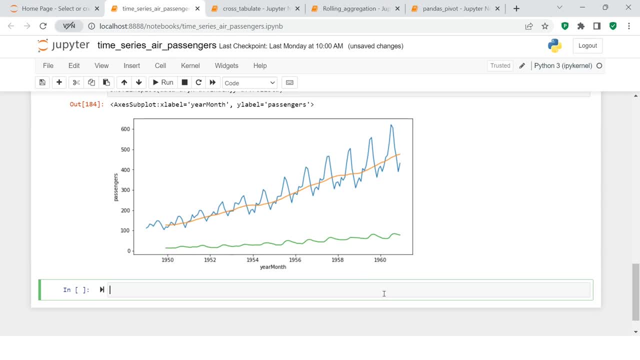 Okay, Which is which I just explained over here. Augmented Dickey-Fuller test. Okay, Augmented Dickey-Fuller test. Now let's see how can we do that. So for that you need to import a module from statistical, I would say statsmodelsdsacom. 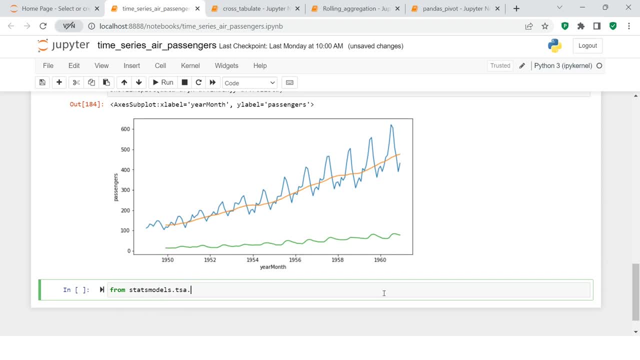 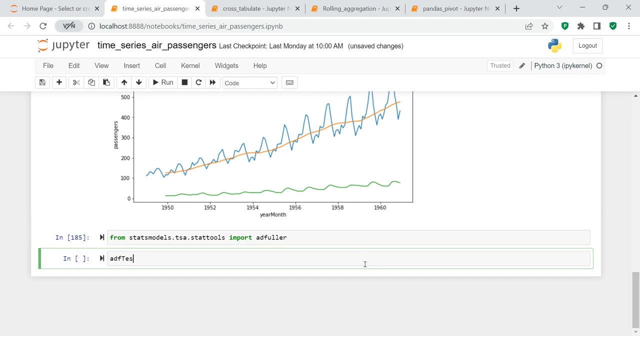 Okay, DSA dot stat tools: import ADF- ADF filler. Okay, Now we got it. Now let's create a data frame called ADF test, And over here I'm just going to put ADF filler and inside that I will take the variable. 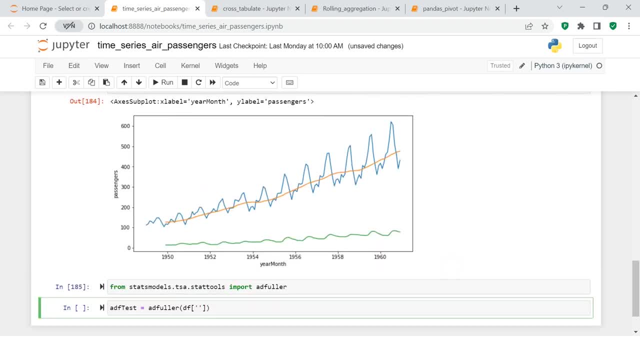 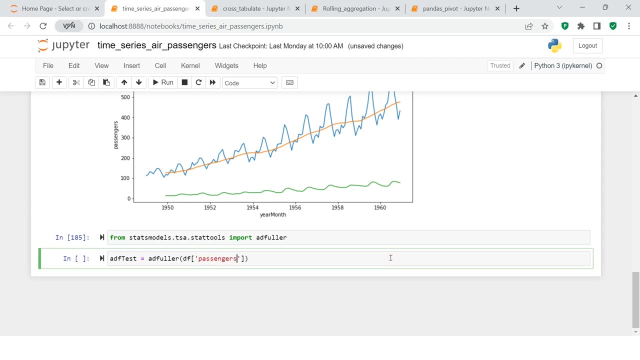 which is nothing but passengers. Okay, Uh, if I can copy this, yes, it will be quick. So here I put this. and there is one more parameter which you need to pass on, And that is this: this one auto lag equals to AIC. 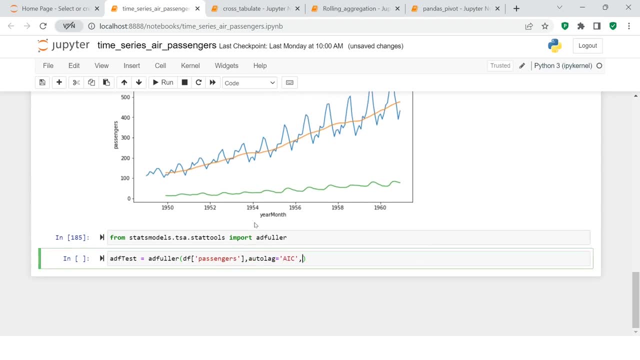 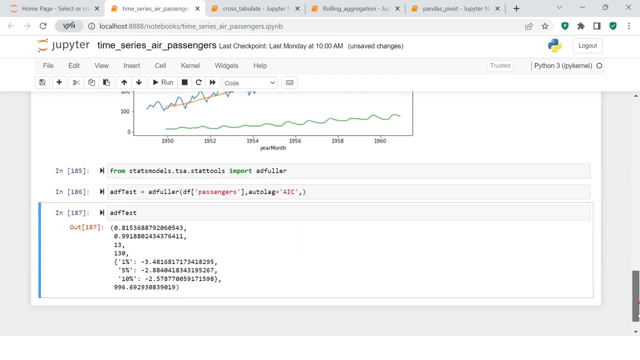 This is default, one which you need to pass away and no need to put much mind into it. Now this is done, Let's try to see what is the value that we are getting. All right, So we got this value, but it is not clear what. what does it represents too. 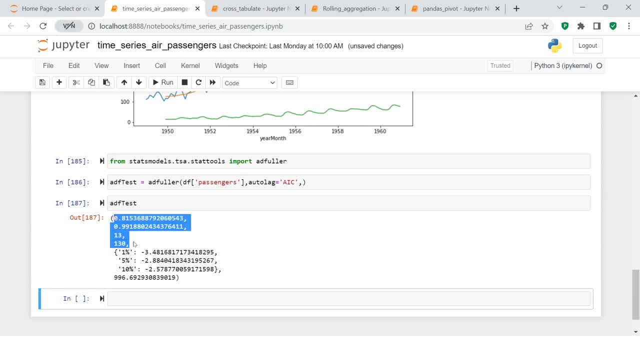 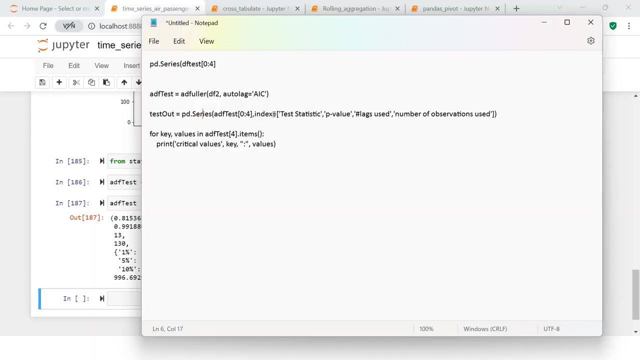 Let me make it clear, Right? So there are two segments. You can see this one and this one. So this is criticality and this is the statistics, like test statistics, P value and all those things. So here I have noted it all down, which will just put it: I'll, I'll just take it. 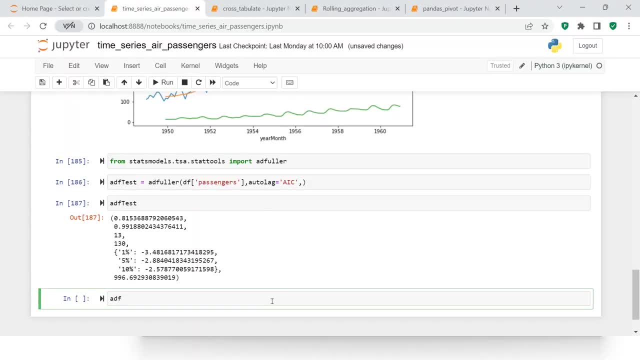 I'll just take this. Okay. So for first exam, Let me show you something. Okay, So if you say this and if you slice this zero to four, so this is what you are getting right, The first segment, Okay. 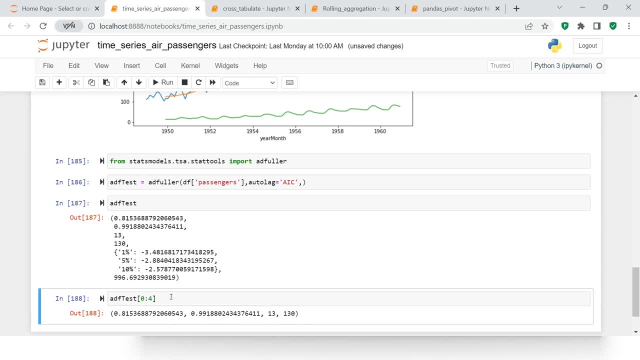 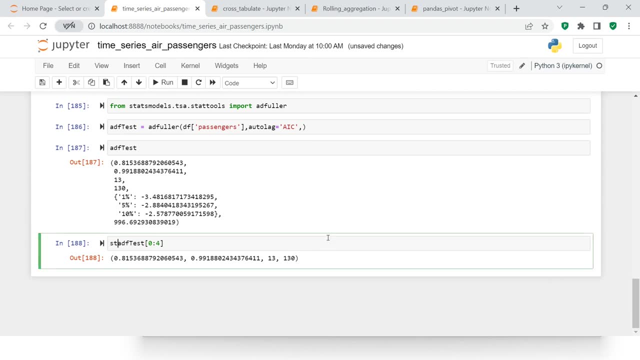 Now, what are these values? How would you know what are these values? Okay, So for that, I'm just going to convert it into a series, so that it will be easy for us. Okay, So let's just say stats. stats equals to this: 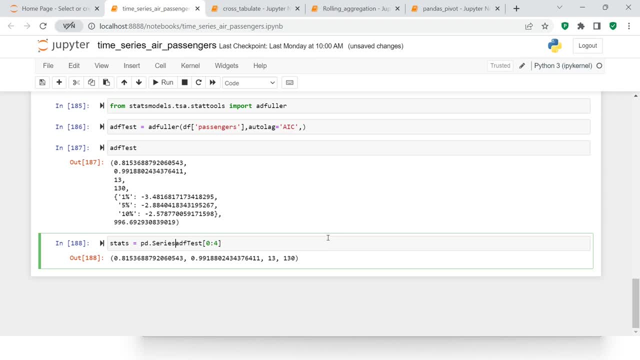 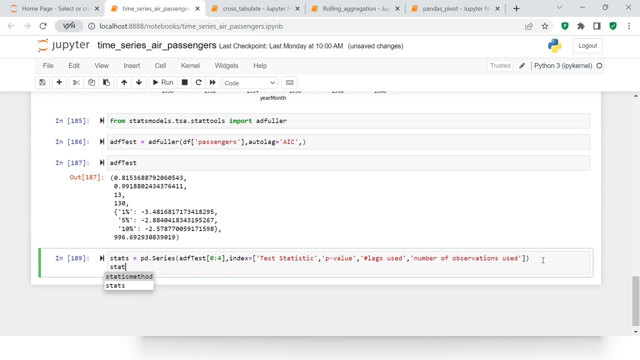 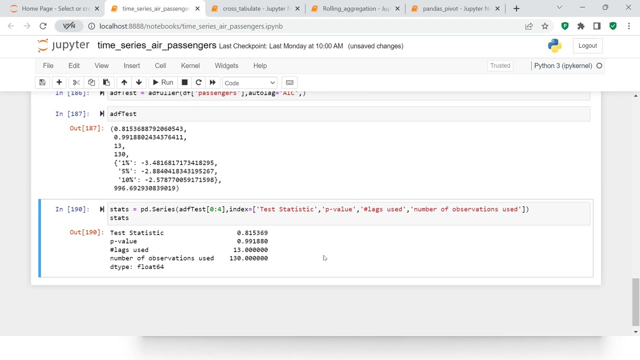 And here I would say PD, dot series, Okay, Okay, And inside that I'm just going to say index, whatever I have copied over here, right, I'll just put it and let's just print that stats. You see, over here here the test statistics which we are getting is 0.81, right. 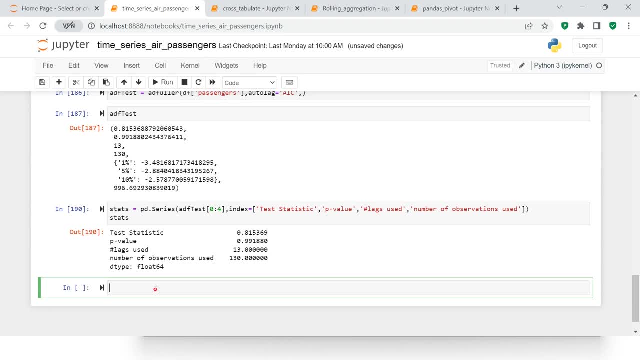 Now let's see the criticality. These are the criticalities. Okay, So we just have to print that. So for X. you see this is a dictionary. If you want to understand how to iterate through the dictionary, I have a separate video. 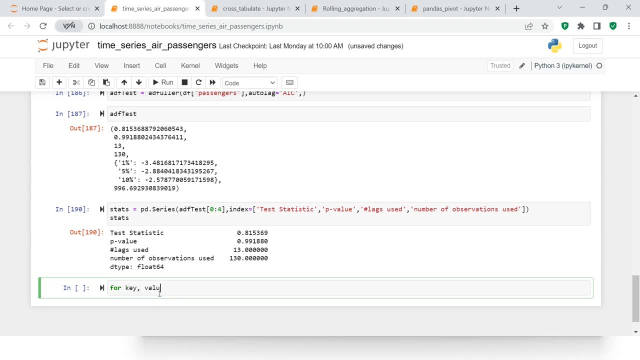 Just check that out. Okay, For key and values in. in we can say AD test filler, AD, ADF test, which we have created, and into that we want to pick the fourth element, dot items. All right, Now let's just try to print. 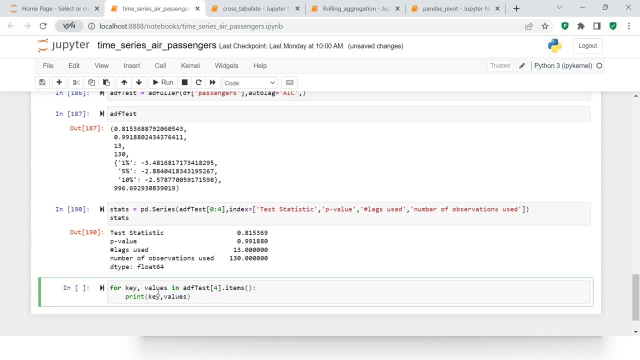 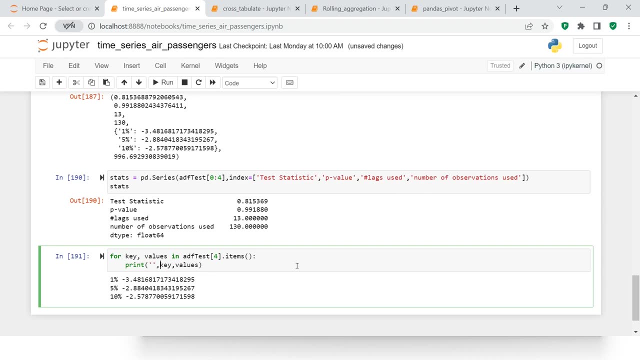 You print key and values, but this is again in this story. again remains same. So here I'm just going to say this, and here I'm just going to say this: I'm just trying to decorate it, Nothing else, Okay. So criticality. 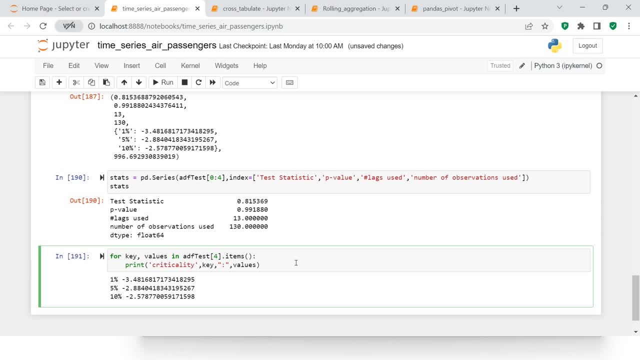 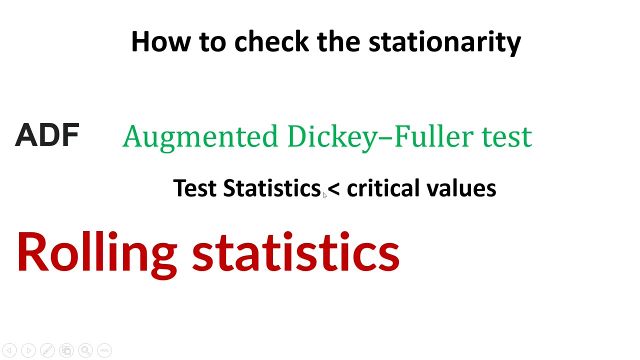 All right Now you see. So criticality: 1%, 5% and 10%. Okay, And 10%, This is the interval. So for 1% we are getting minus three, minus two and minus two. Okay, But see, the condition says over here that test statistics should be less than critical. 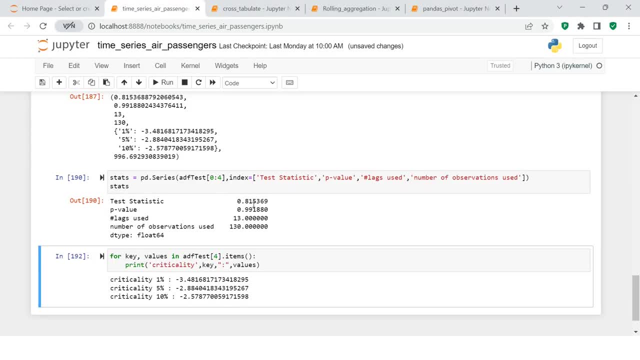 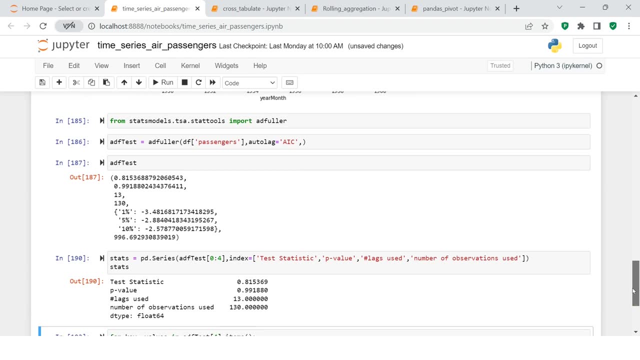 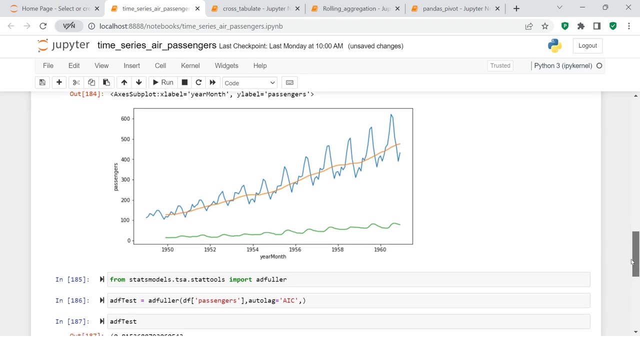 values, but the critical values which we are getting. that is less than test statistics, which means clearly our data is not stationary, right? So they hope this was clear to you Now. in the next video, we will understand how to make this data stationary. 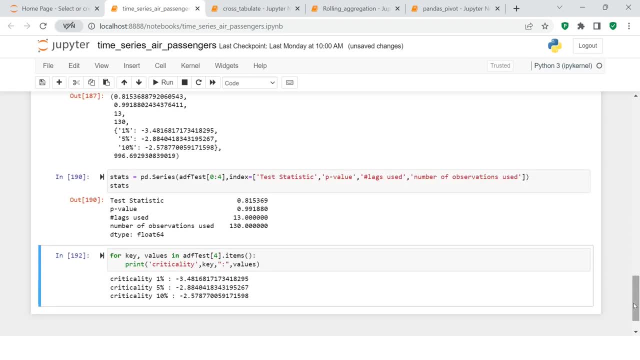 What are the ways to make it stationary? Okay, I just hope that in this video we covered what stationarity is. what are the types of the stationarity? Okay, So, types of- for types of the stationarity it is nothing, but let's say it could be seasonal. 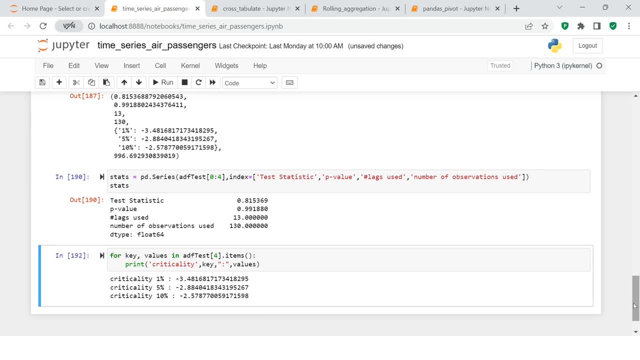 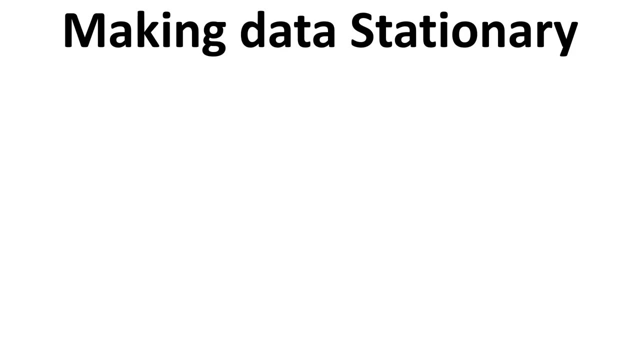 stationarity. It could be trained stationarity and all those things, And we also covered how to check the stationarity in the data. Hope it was clear to you. are going to understand how to make the data stationary if it is not Primarily. 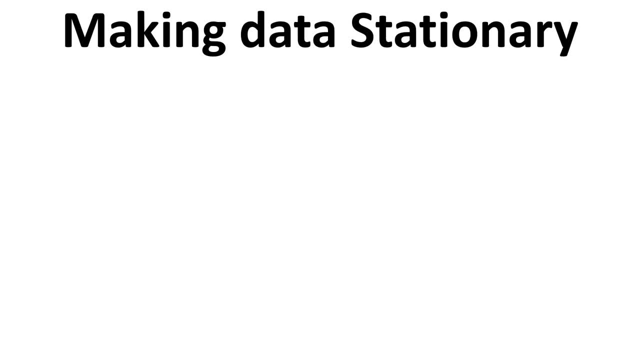 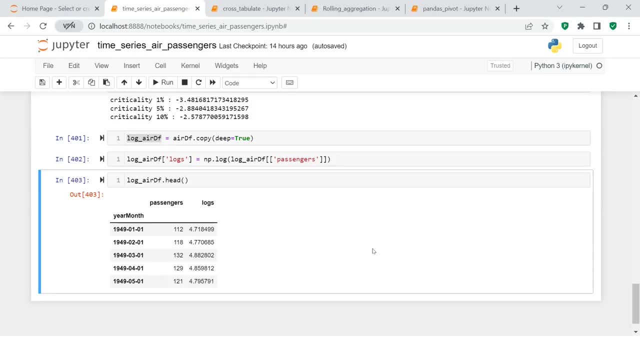 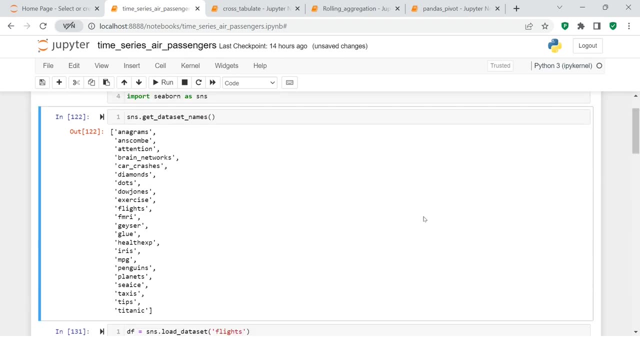 There are three ways which you can use to make your data stationary. The most simplest one. All right, Before I take you to that, one more thing. here is a quick view. So what? this is what we had understood in the previous video, where we tried to you. 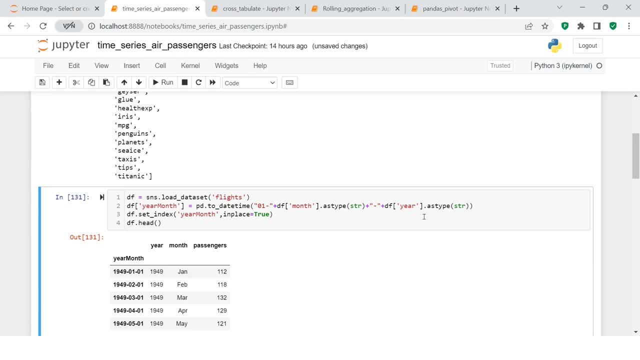 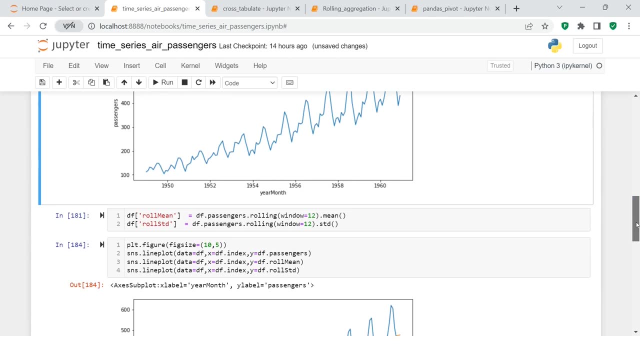 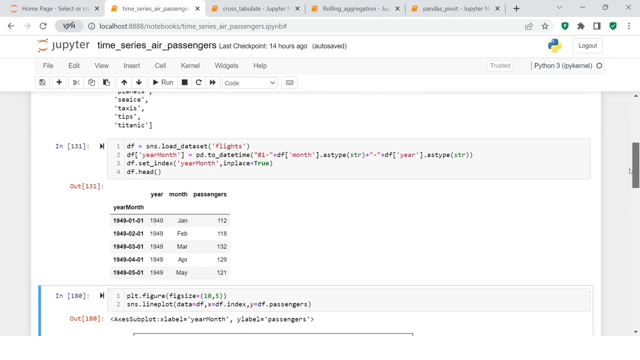 know, check the stationarity of data by two ways. One number one um this I'm just showing you because just in case we have not seen the previous video, Then you can. You will have some idea right. So we just discussed there are two ways of finding this thing um checking out the stationarity. 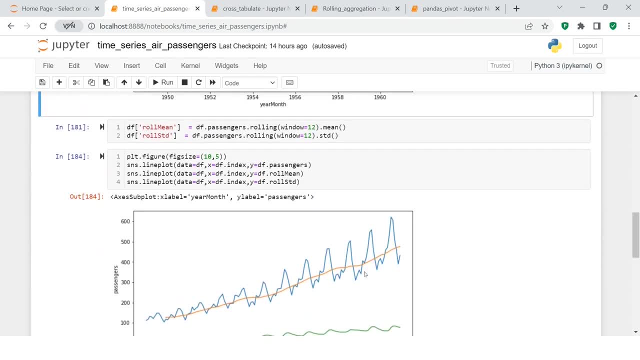 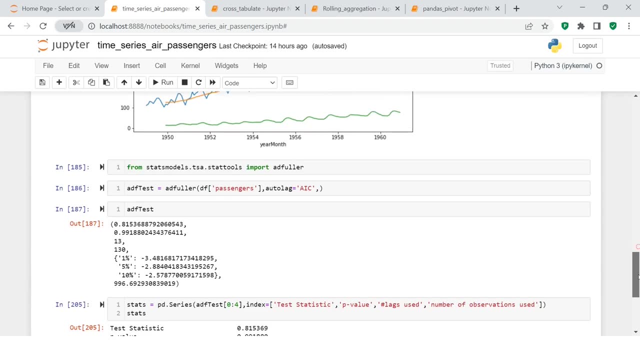 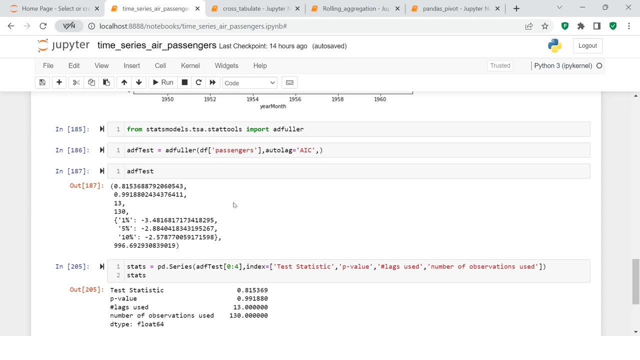 of the data Number one by rolling statistics which we did over here, where we find rolling mean and rolling standard deviation. we plotted them all over here And then we saw whether the data is stationary or not In this segment. we tried to do the ADF test, or somebody also call it, or I mean somewhere. 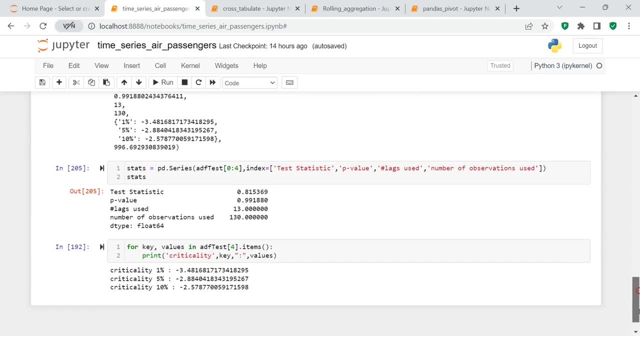 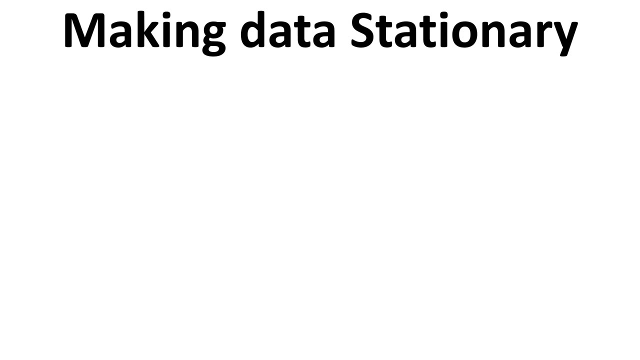 it is also called as ADF test Right. This is on that We get certain statistics and which helps us conclude whether the data is stationary or not. Now, coming back over here, there are three primary ways which you can use to make your. 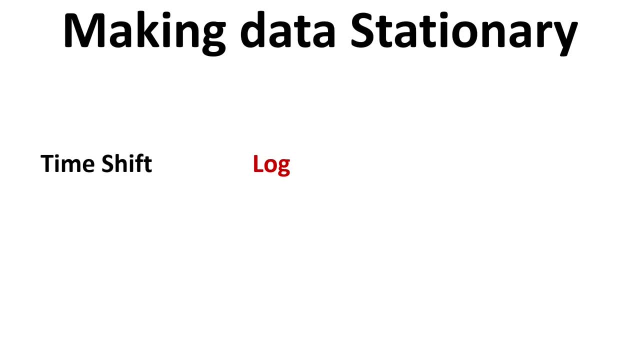 data stationary Number one timesheet- This is the simplest one- Then log, then finding a square root cube, et cetera. So these are the three ways, or rather I can say whatever the ways are there, you know. 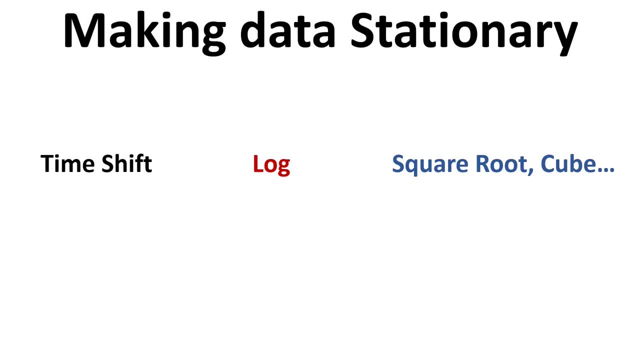 um, these are the most commonly used right And there's no fix. There isn't any fixed sequence that first you should go for timeshift, then log, then square root and cube right. You can try any of them in whatever sequence you want, but the most convenient way is to. 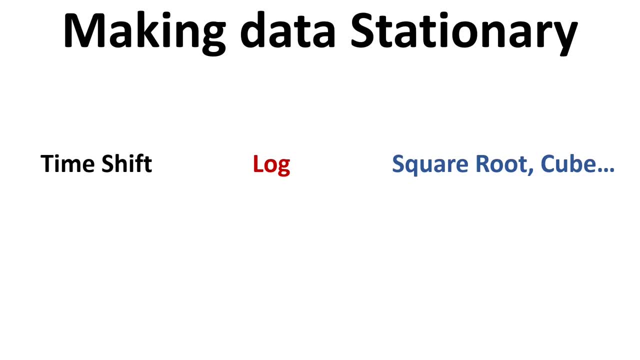 go first with timeshift, because that's the simplest one. Then there it is also not necessary that you try all these three. if you find your data stationary enough On timeshift itself, it is not necessary that you try all these three. 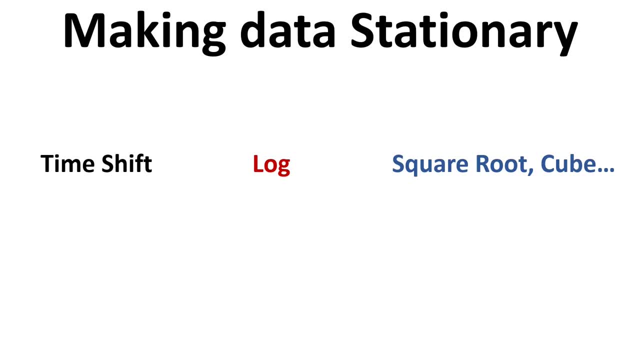 If you find your data stationary enough on timeshift itself, then you can try all these three. On timeshift itself you can go ahead and start building your model. If you find it on log, then you can start with model building. Same goes with square root and cube. 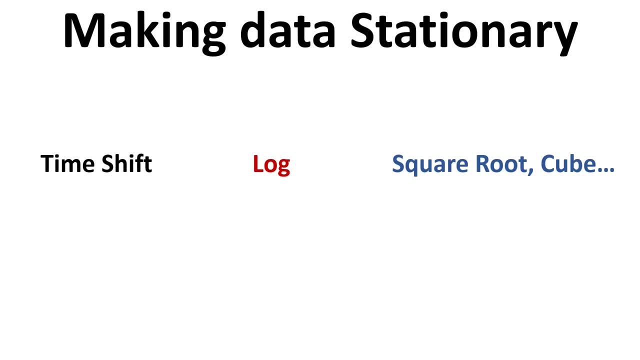 If you still don't find your data stationary enough or satisfactory enough, you can combine them also to find a satisfactory outcome. Let's have a look on timeshift what exactly happens over here? So let's say: this is your data. If you remember, in the first video we saw this: 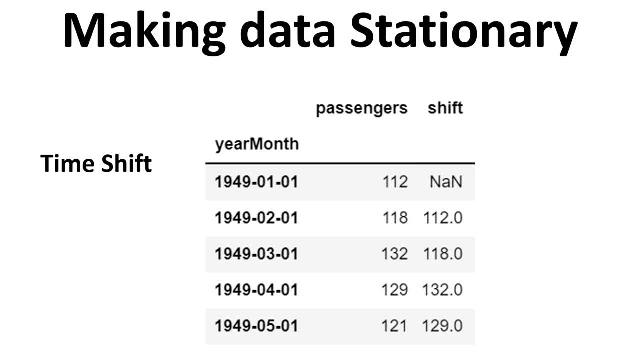 So here you exactly: shift the values By a specific interval. So if you notice over here, here we are shifting the data by one month. How, If you see the number of passengers? 112, the data has in the month of January 1949, which? 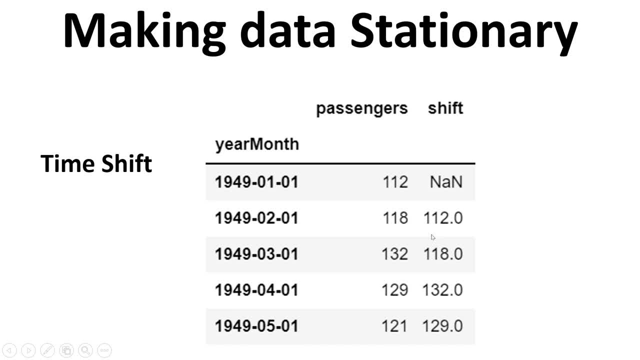 is shifted to the February 1949.. This is the shift which we have done. After doing this. same goes for 118.. It was for February, but that is shifted to March. right, In SAS we call it lag, Okay. 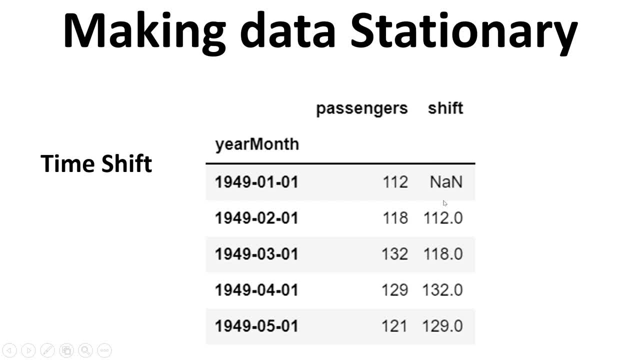 And over here We are saying it's shift. So here I'm shifting the data by one month. If you want, you can shift it by six months, 12 months, 24 months, whatever the way you want. It's not necessary that you go by 6-12 only. 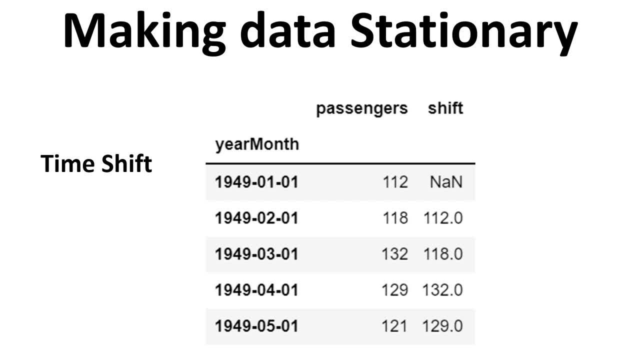 You can also shift it by seven months, eight months, whatever fits well to your data. Then, after shifting this, we find the difference of both of these two, the actual one and the shifted one, And whatever value we get. based on that, you can do your stationary test. 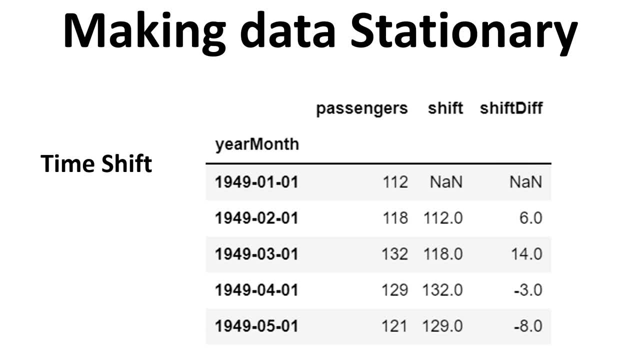 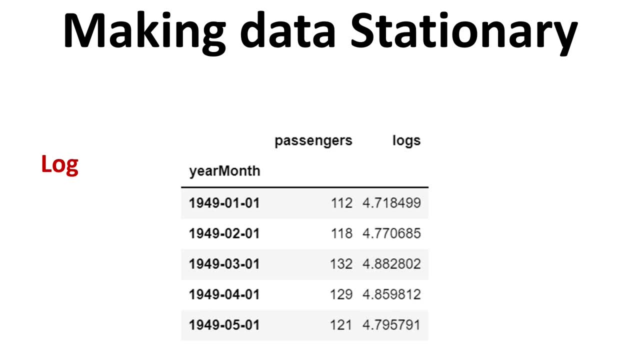 How does it look like? And then you can decide to go ahead and build the model. Same happens with log In log. what we do Is we simply find the log of dependent variable And then again we do the stationary test. 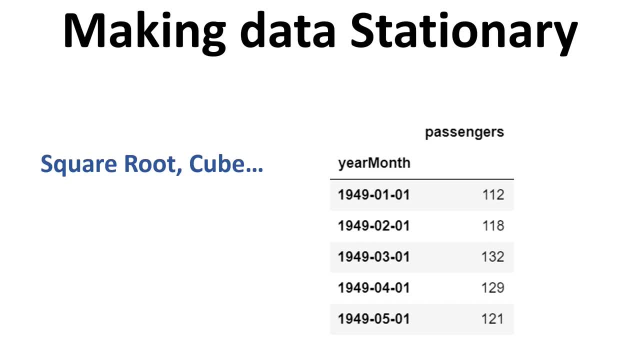 If it looks fine, we can go ahead and build. the same goes for finding the square root, cube, et cetera. You simply find the square root or similar in the similar fashion. you can also find the cube here I have just shown for square. 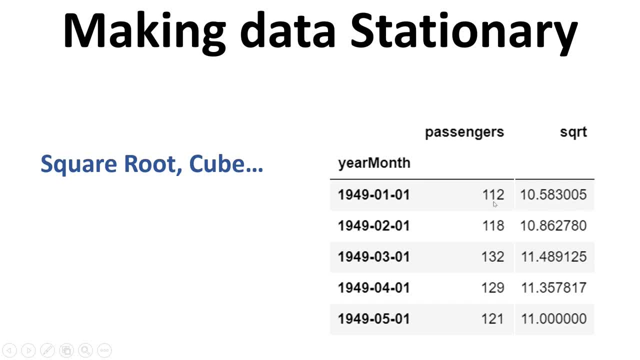 And then you can see if this does not work. see what you can do is you can also find the difference. and then you can do that. instead of using the passengers, you can try to, instead of using this actual value, you can try to use the log value of this and then square. 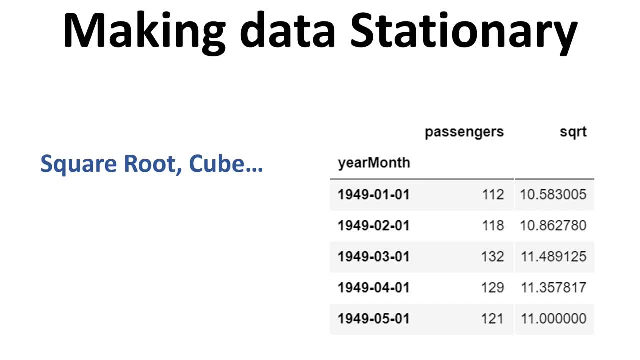 root that and then find the, find the difference and check out this stationarity. So there are multiple ways. all right, a lot of discussion. Let's jump to the Jupyter notebook and try to understand it with practical example. The moment you feel confused, just pause the video. put your doubt in the comment section. 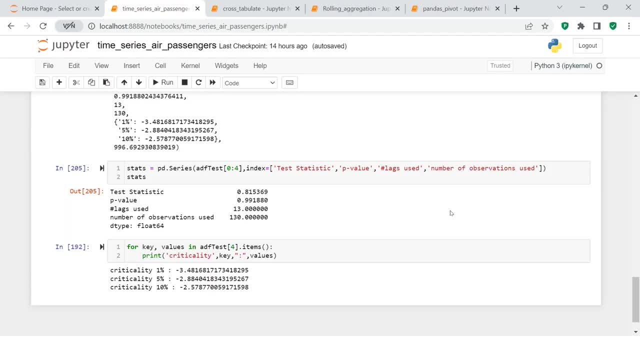 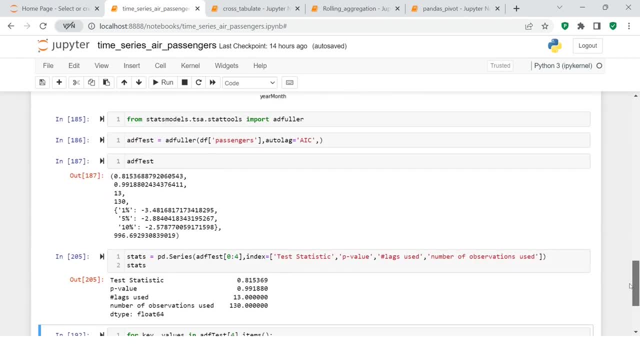 on the bell icon, click on the bell icon, click on the zebra in the bottom right corner And after we move forward, what I do is because we will have to keep on doing this test again and again. So what I do is: I'll quickly make up a. I'll quickly. 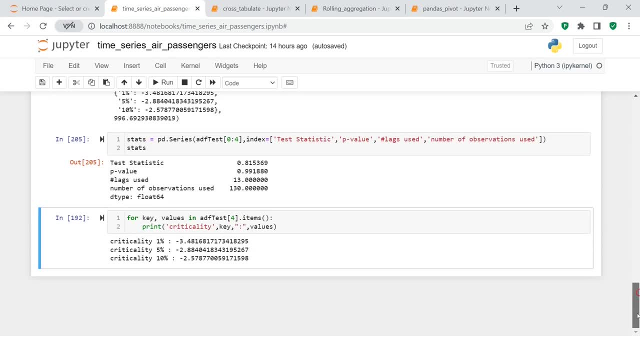 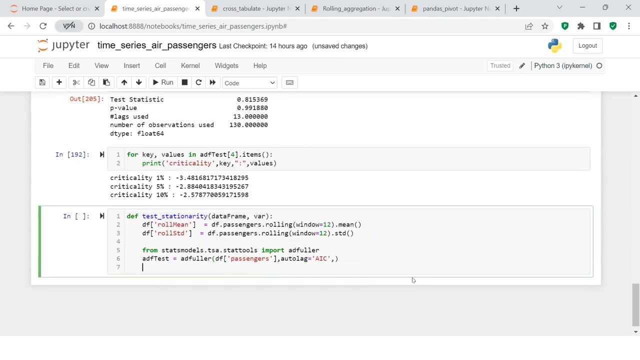 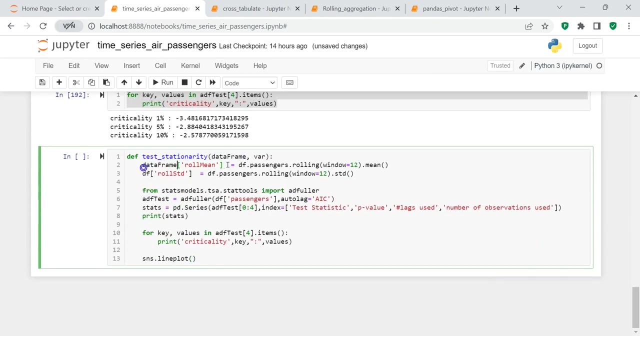 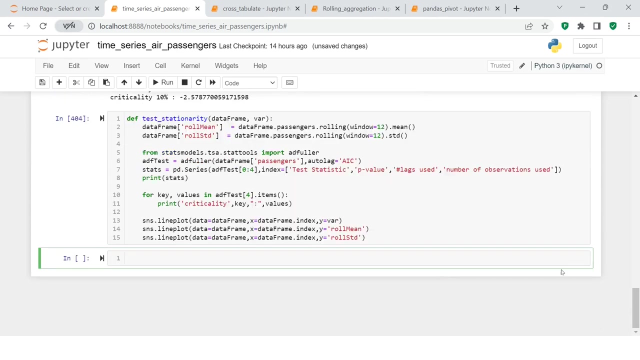 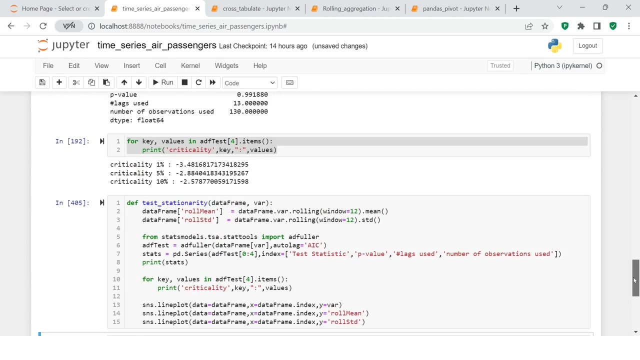 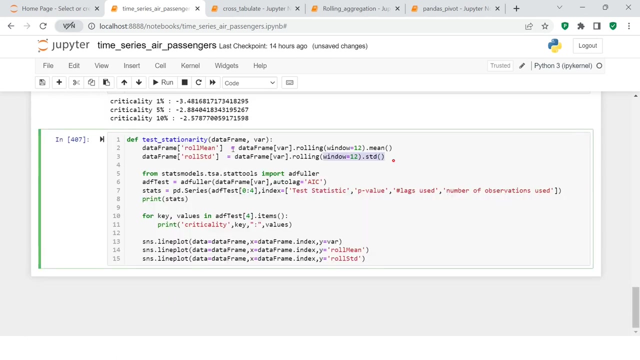 put them all together and make a function And then we will move forward with making the data stationary. That will be helpful. So while I make the function, enjoy, We'll be right back. What exactly I did is: first I'm trying to, whatever data you supply and whatever the 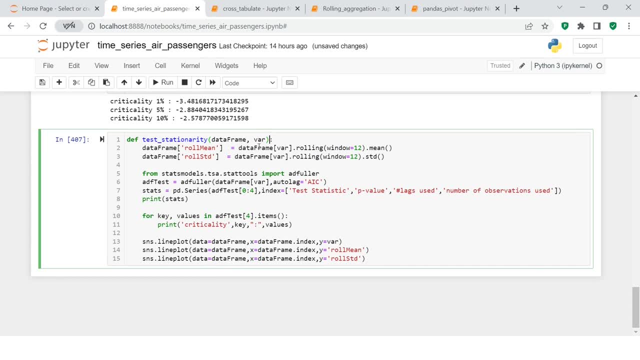 variable you supply, for which you want to, you know, check the stationarity. this function I'm creating because we'll have to keep on checking the stationarity again and again, All right, So for that reason, this video, this function, we have. 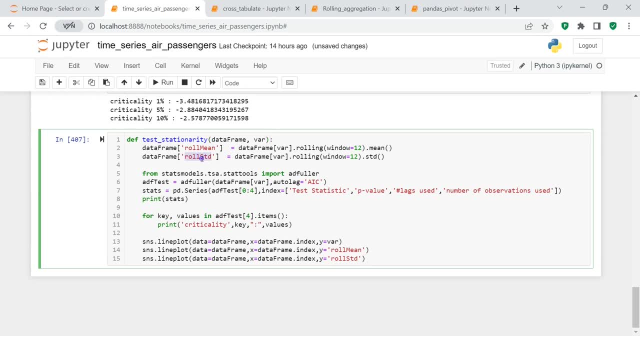 So here, first I'm trying to create the rolling mean, then rolling standard deviation Right, And once that is created, here I'm trying to do the IDF test right. And if you look at this and then whatever the test, 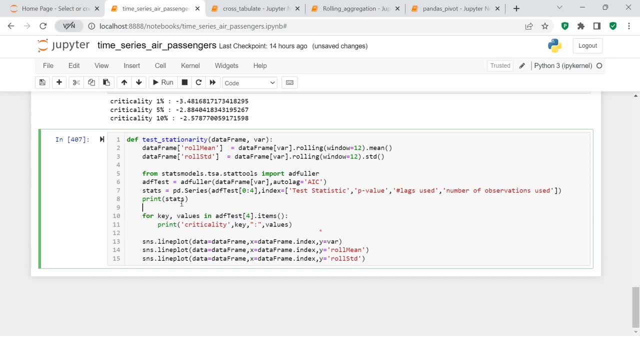 Test comes over here. I'm trying to print over here. right, One print is over here. This will do the statistics printing and the printing, And then this is going to do the criticality printing. OK, And this part is going to plot the data. 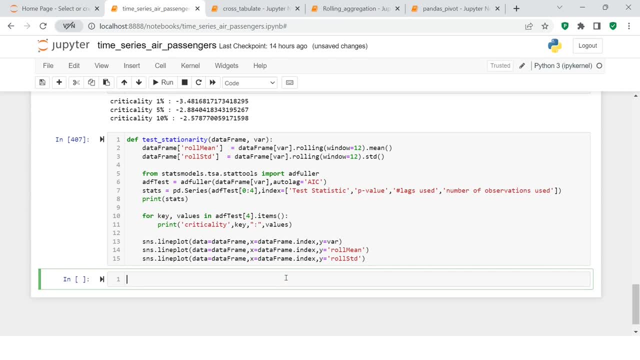 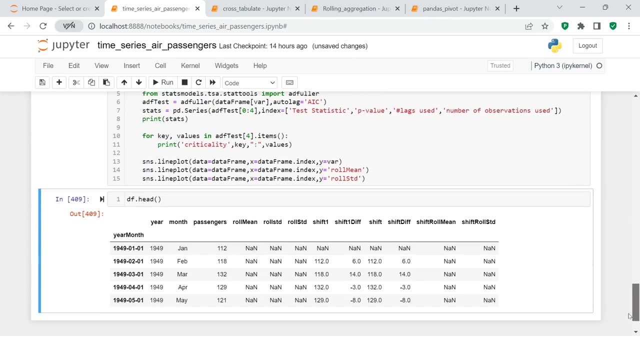 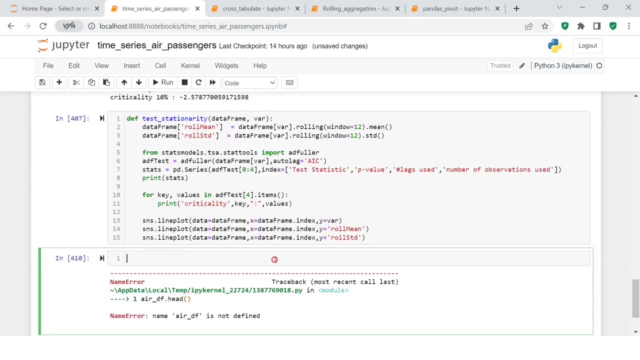 OK, Let's test this if this is working well or not. To test that: here we have our data called DF And let's see This is how our data looks like. OK, We have error DF, also error DF, which, which actually should be the same data here. 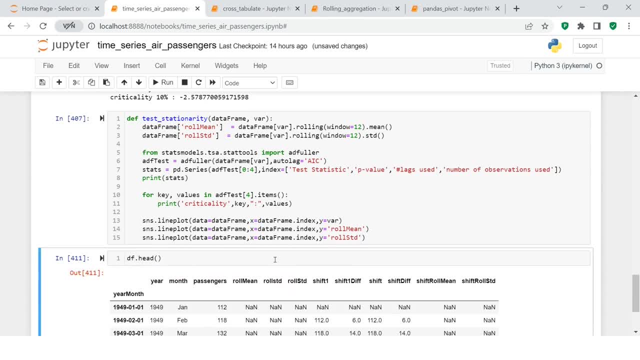 All right, No problem. So let's say DF, dot head. OK, Now we want to test this. So for that, what we can do is test the stationarity and in that supply the data frame name and then supply the variable, and variable name is passengers on which. 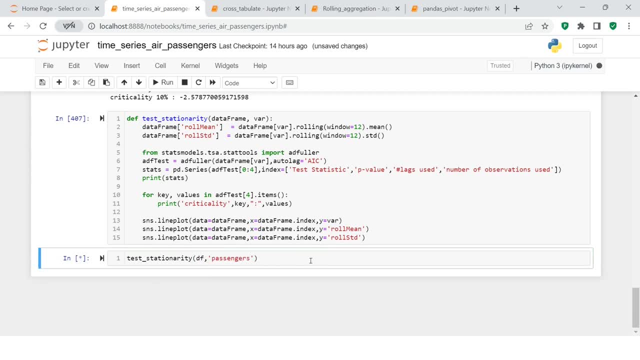 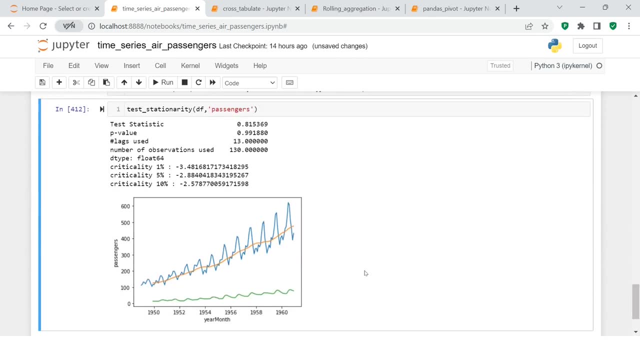 we want to do this test. Remember this has to be in quotations. Now, once you do this, this is what you get. All right, So this is how we will keep on using. So here you see, this is the actual value. 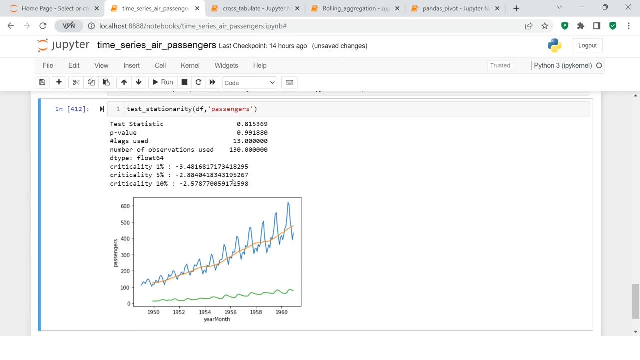 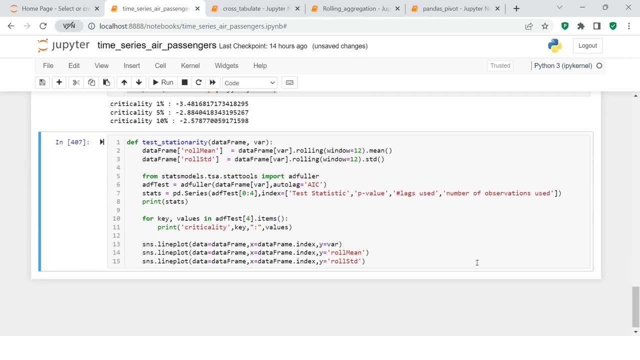 This is rolling mean and this is the standard deviation. And here you have these statistics. Well, well done. So we will we keep, we will keep on using this function again and again. OK, So now, before we move forward, let's make the data clean so that we could. 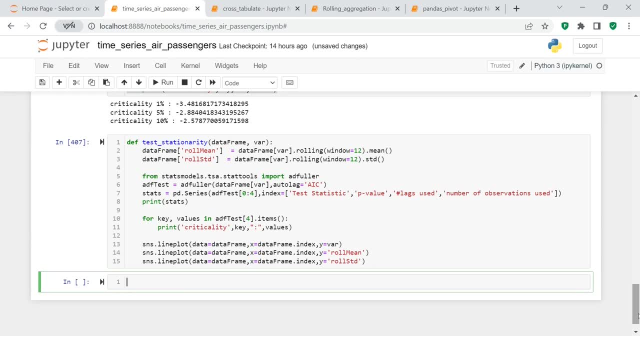 We it, it would be easy specifically for us to continue our OK. so if you see, in the data here you have a lot of variables, So we are going to let's create another data, Let's call it ADF, And in that I'm going to say DF. 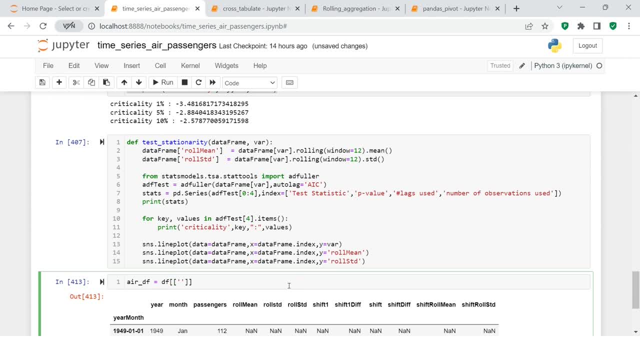 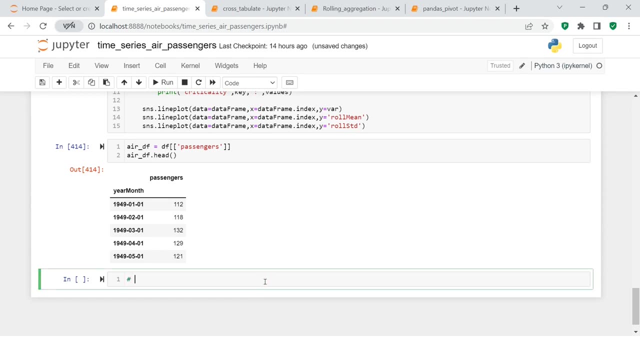 And out of that I will just take passengers. This is all that I need. OK, DF, dot it. You see now, that's, that's all that I need. OK, now let's try the first method. First method we discuss is by shifting. 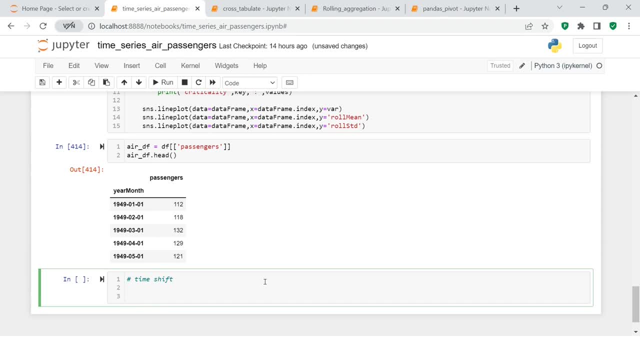 the time time shift. Now let's just try. So how can we do that? So here I have my data frame, which is called ADF, And in that I'm just going to create a variable called shift Right, And you can also say shift one. 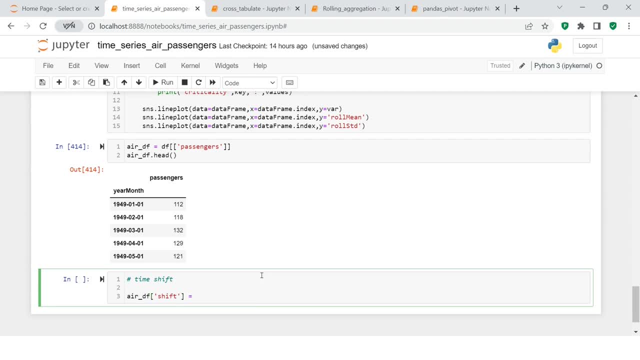 OK, or let's call it shift only because we will keep on changing this and trying this. OK, so this is what our shift is now. After that, what do you can do is use a data frame name, dot the variable name To which you want to shift and then say: 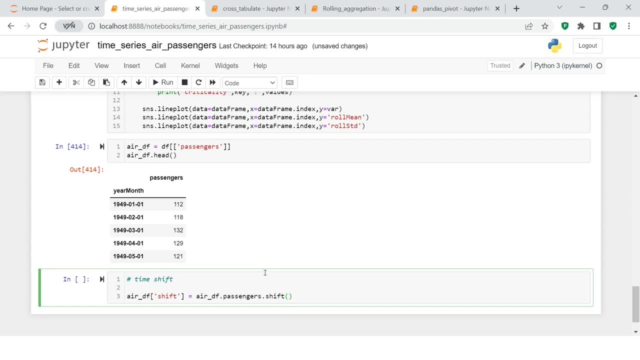 call this function, which is called shift, and by how many months, if you want to So. do you want to shift it? So, if you want to shift it by just one month, you don't need to put any value over here. OK, if you want to put. if you want to shift it by more than one month. 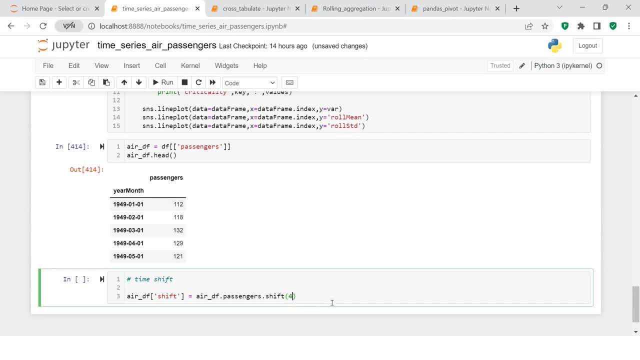 then you need to put the value. for example, if you want to shift it by four month, then just put it, for let's try with the simple one. So here we have ADF and we are going to say: you know this thing. 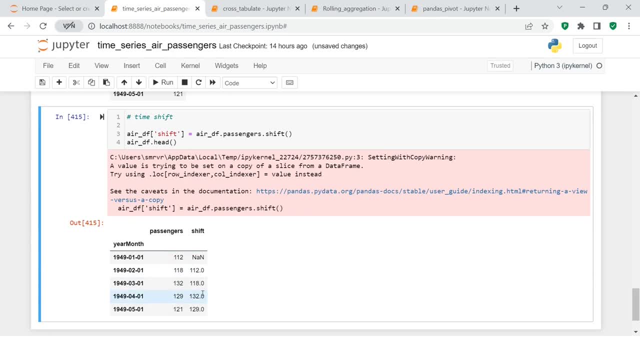 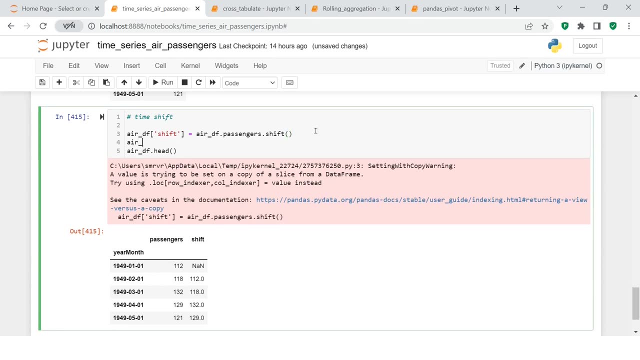 Like you can see over here Right. So here the value is shifted. Now the next step is finding the difference. So let me just create another variable which I would say: look, I'm trying to keep it to the absolute beginner level, Right. 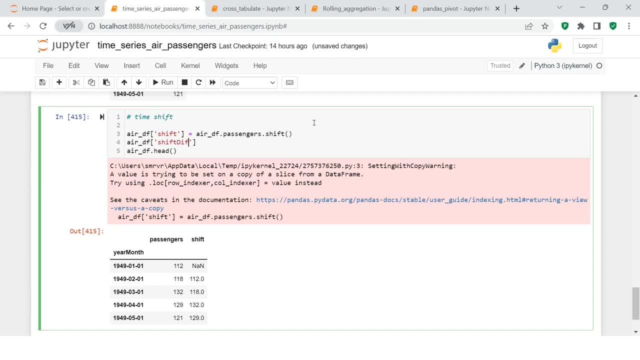 But if you find it little annoying, So just try to watch it in double speed, or maybe one point five. Now, the next thing which we're going to do over here is this: We will- We'll- subtract ADF. Sorry, ADF dot passengers. 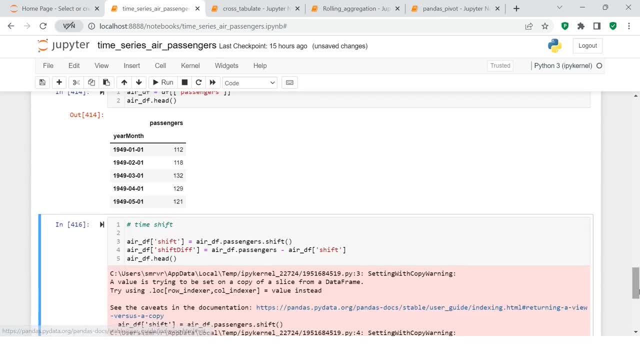 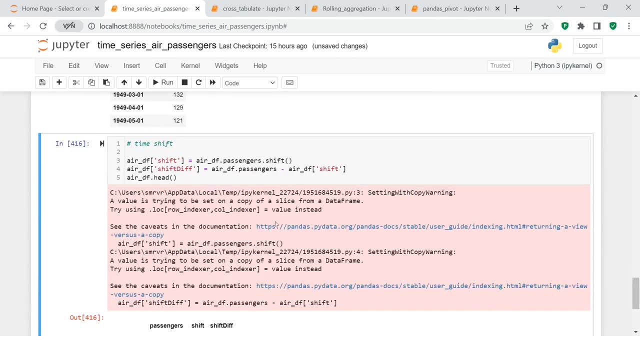 minus this thing. OK, now let's just see how the data looks like. OK, so this is done. Now the next thing is testing the data, Or let's just try if this looks much better. No, it's the same thing. 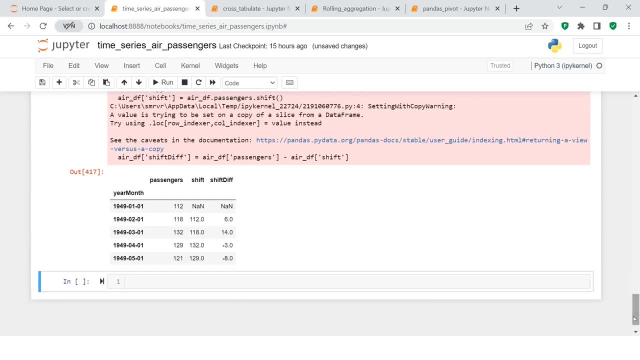 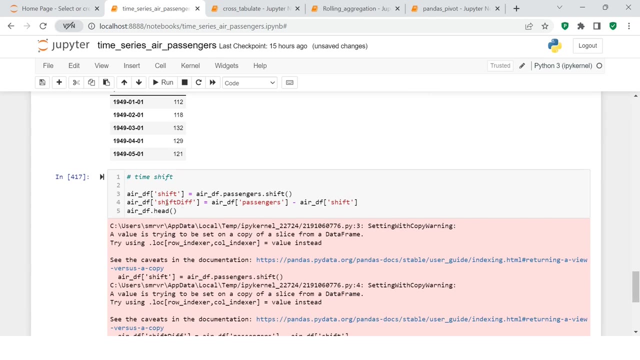 OK, so this is looking the same. Now, the next thing which we're going to do is check out the stationarity of this data. OK, so test stationarity, and the data frame which we have created is ARDF, and in that what we are going to use is shift difference. 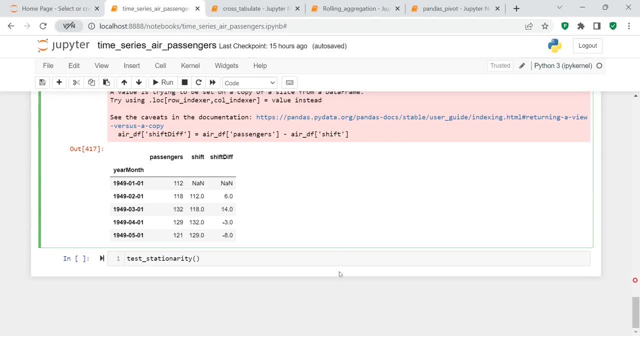 This is the variable which we will be using. OK, so let's just call it over here: ARDF. This is the data frame Name, and the variable which we want to use is this. Now just hit enter and see the magic. 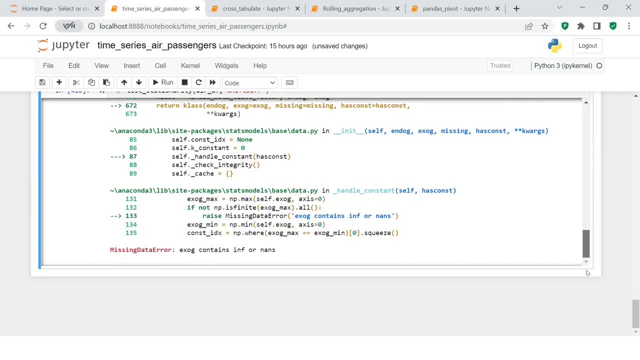 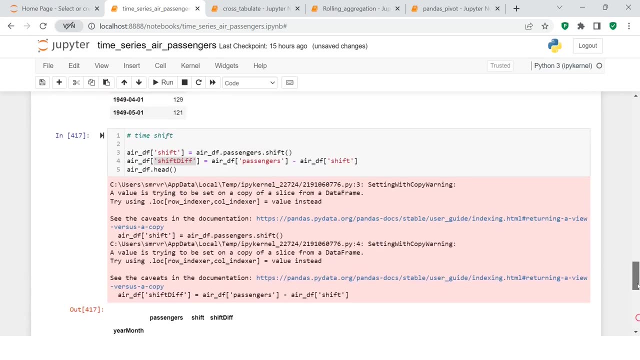 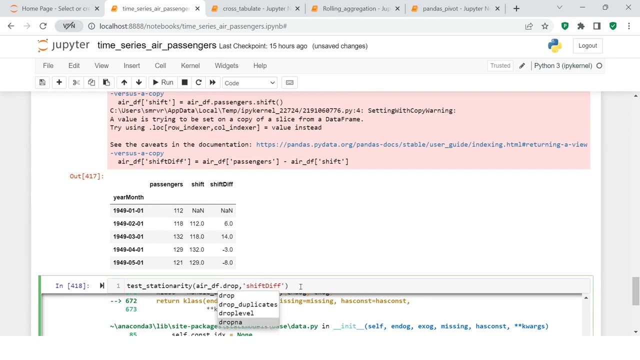 Oh, it showed the error. Let me just figure out what the error is. It all contains information, or NANs. OK, so what do you see over here? is this NAN that is creating problems? So that's not an issue, Let's call it: drop NAN and let's just do this and let's see if it worked. 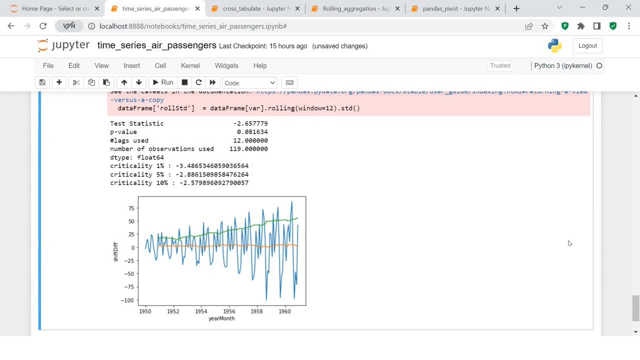 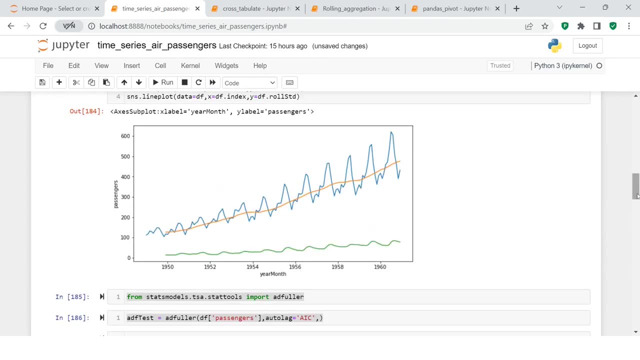 Yeah, So here is what we have now. You see, this is still much better right From, as compared to the original data, or originally we had the data like this: Right And after doing the shift transformation, this is how the data looks like. 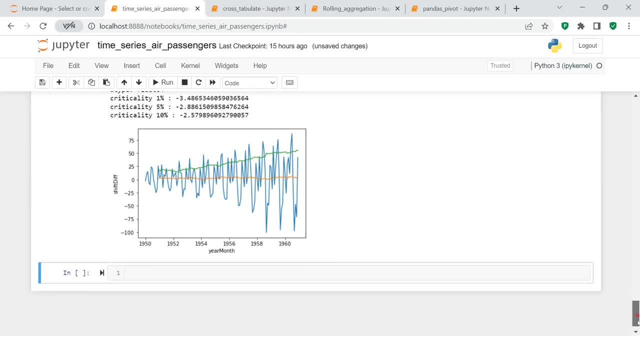 So this was the shift transformation. Next comes is log transformation, right, So let's just try to see how we can do that, So if you have not understood it pretty well. So before I move forward, let me give you a quick view. 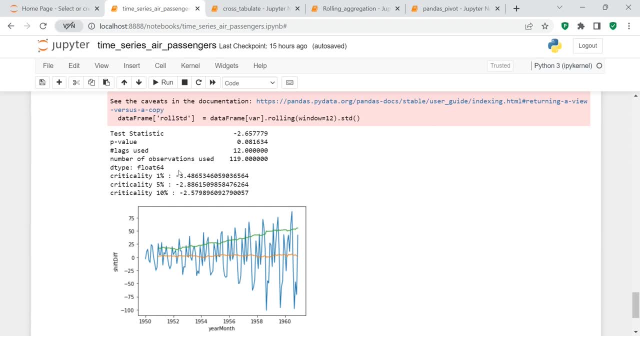 So if you see over here, test statistics is minus two point six five, while the criticality is minus three point four for first percentage interval And you see this is somewhere closer to this criticality Right And the value is zero point zero eight. 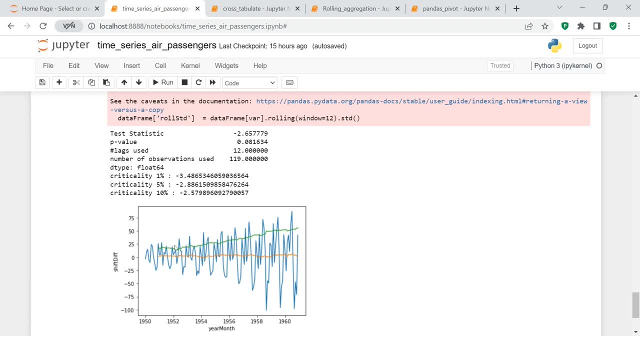 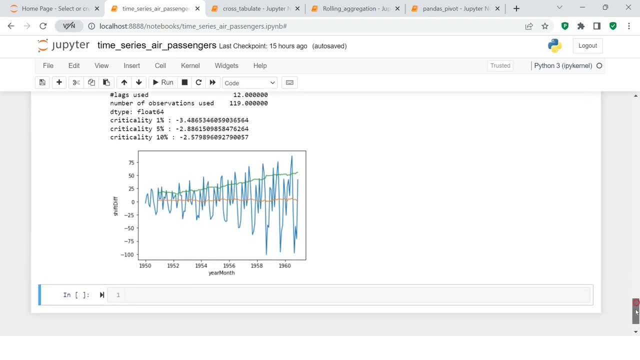 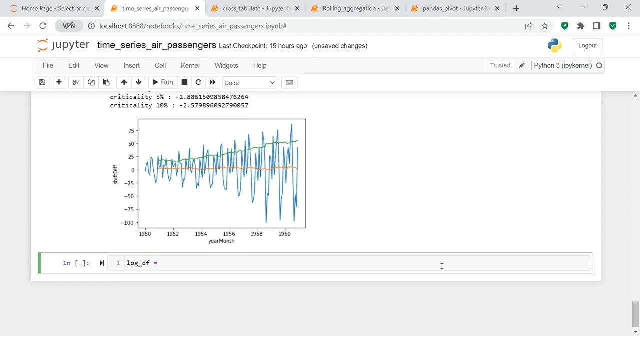 Well, here you see, mean is fairly looking constant, but the variance of standard deviation is showing a kind of trend pattern. OK, so this, this was The one test. now let's move forward and do the another test. before we move forward, Let me just create a subset of the data again. 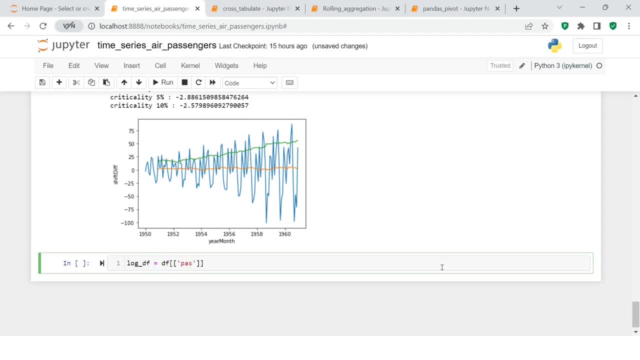 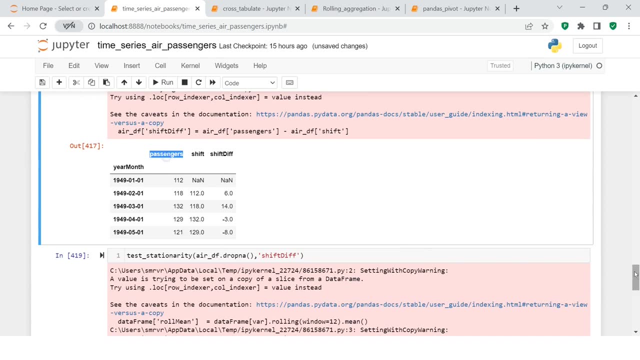 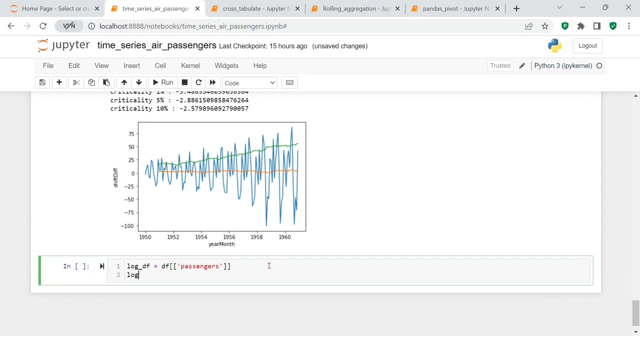 And here I would just say passengers, OK, let me just do a quick copy paste, passengers, because I just don't want to waste the time. Your time is pretty much important And let's just see if this looks good enough. Log Dot header. 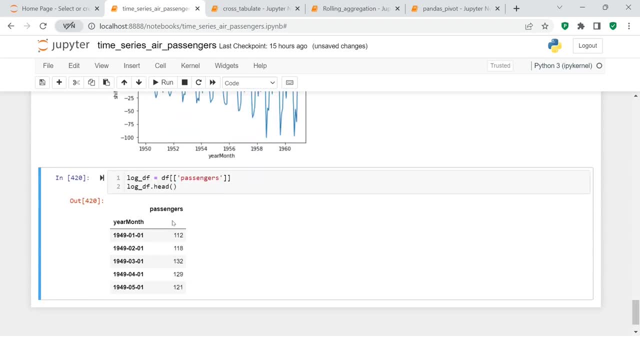 Yes, Now, here we have the data. Next step which we're going to have is find the log of this value. OK, For that, what you can do is you can just simply say log and inside that you just supply the variable which is log df. 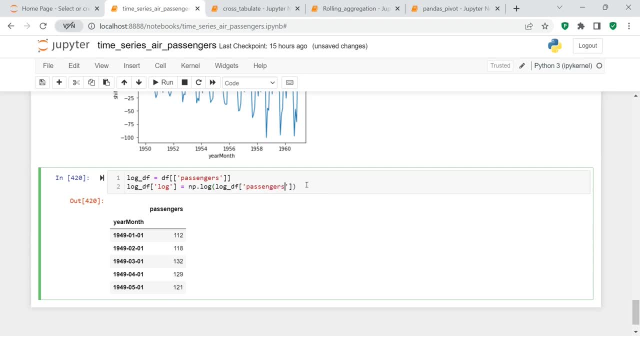 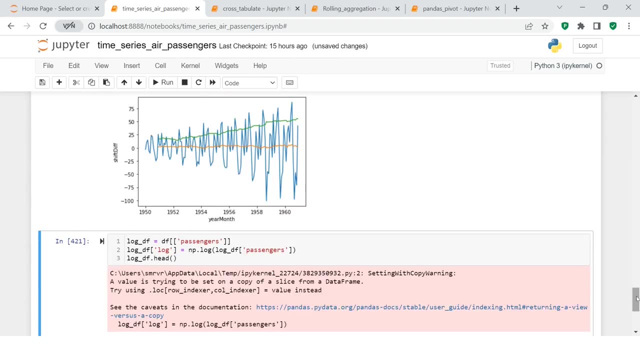 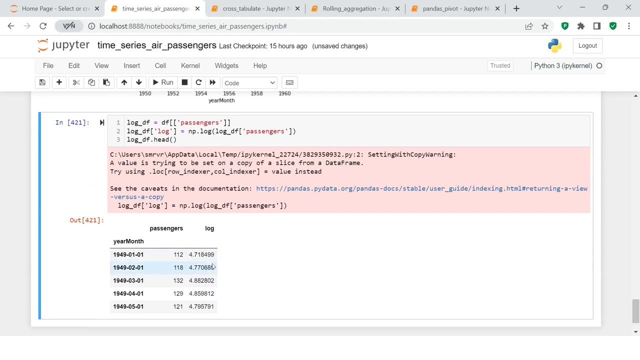 log df and out of that you can just take passengers Right And let's see log underscore df. How does it looks like? So here is what we got. OK, now there are two things. Number one: you can directly check the stationarity on this log variable. 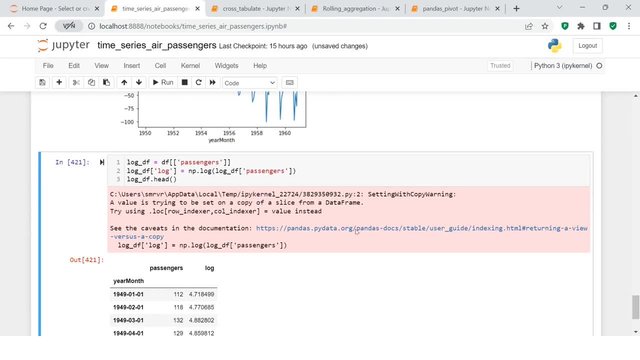 Number two: you can combine the above shifting method into this and then find the difference with log, not with passenger, And then you try to check the stationarity. I'll go ahead with the simplest one first, And then we will see What is required to combine it. 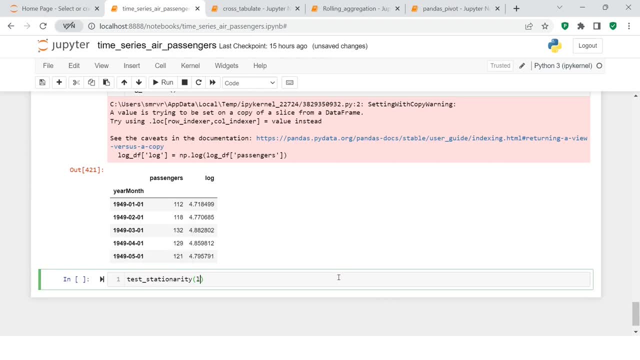 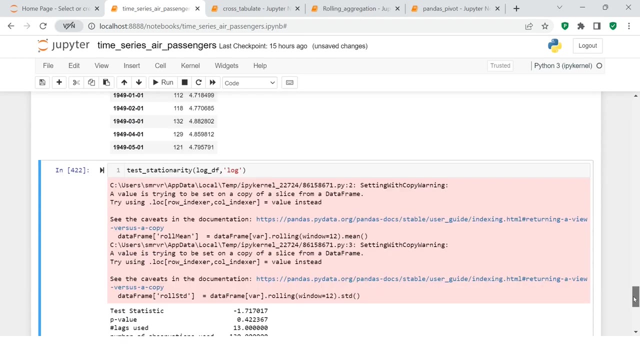 Let's check the test stationarity. OK, in this, the data frame name which I want to use is log df And the variable which I need to use is not passengers but the log. OK, do I have known? I don't get the error this time because we didn't use the shift thing. 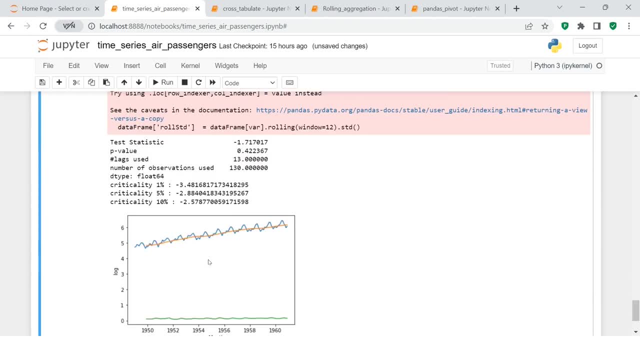 OK, All right, This looks good. The variation is: you know, the variance is pretty constant, But original data and this mean is still showing the pattern into it, Right, But just looking at the graph we cannot conclude it pretty well. 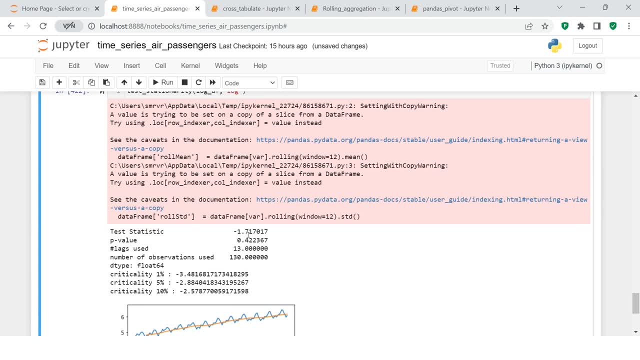 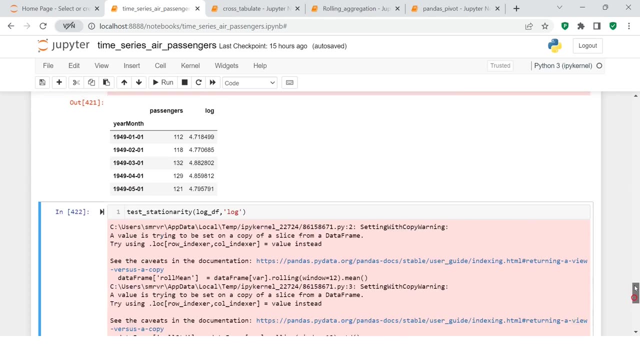 So let's have a look at the statistics. So, in statistics, if you see this minus one point seven, this is fairly, you know good, Compared to the previous one. And if you see the p value is zero point four two. 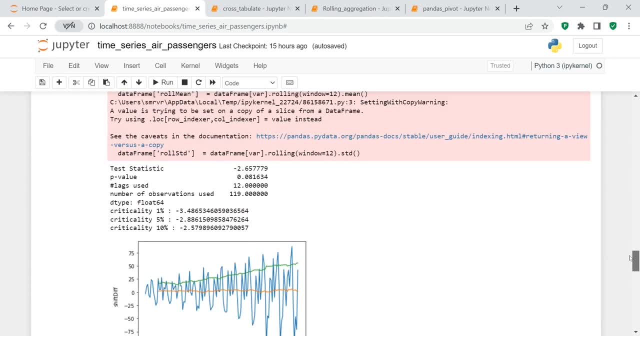 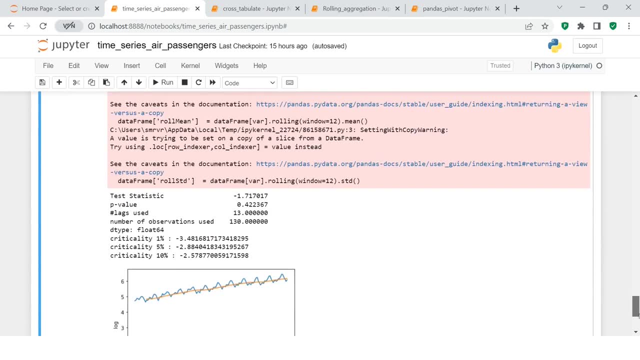 And what is the p value that we have in the previous one? Zero point zero eight. So still, this one time shift looks much better compared to this log thing, Right So? and if you see, this is the mean curve and this is the standard deviation curve. 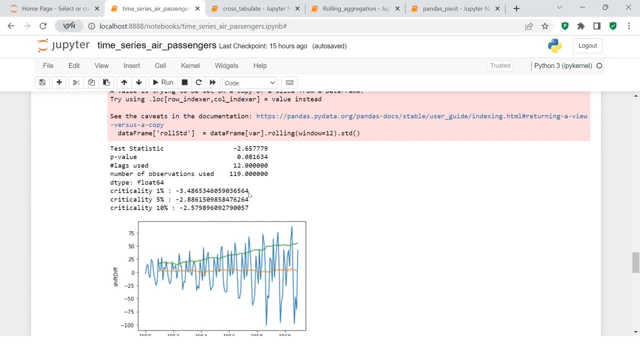 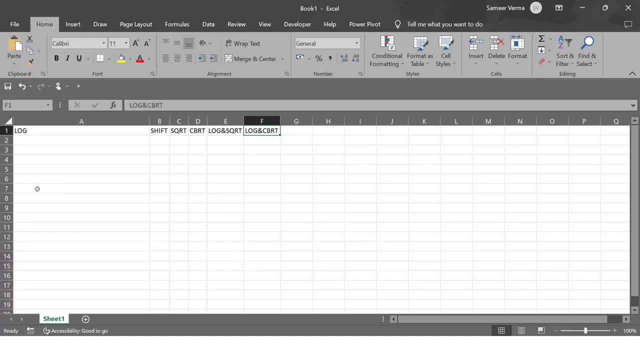 All right, So this is what we had for this one. Now let me just keep this. This one is for here. I have an Excel and I'll put all the things over here. Let me just say shift, for the part is here. 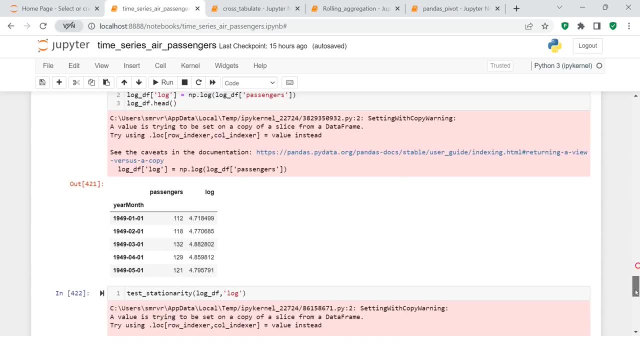 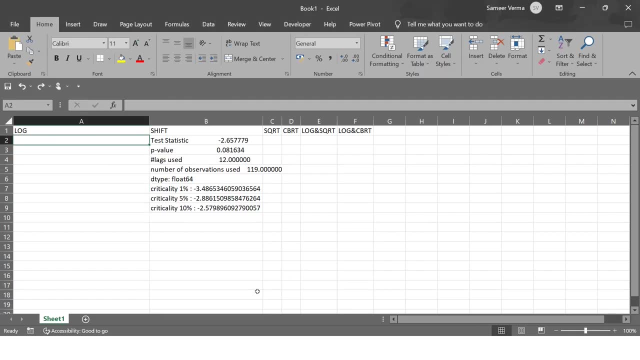 And this is going to be the log, so that it will be just simple for us to quickly have a comparative view. OK, let me just do this. OK, now, if you see, log is showing you The greater p value compared to the shift one. 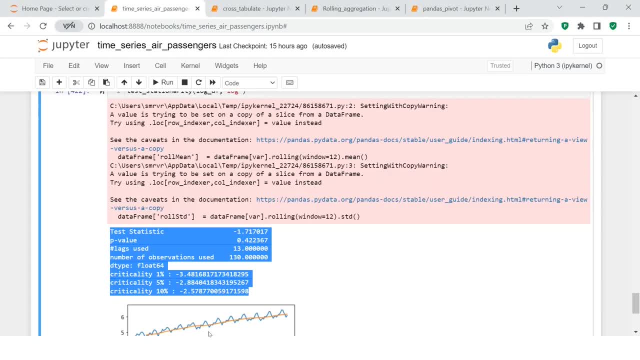 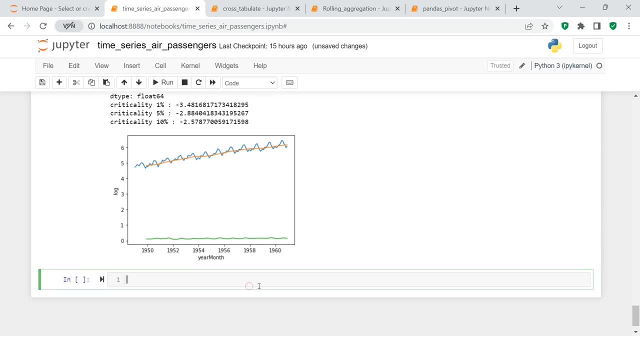 OK, now let's move forward and try to do the square root for square root Again. what I'll do is I'll create another subset of the data. If you want, you can keep. you keep on using the same data, But just for simplicity I'm going to use this over here. 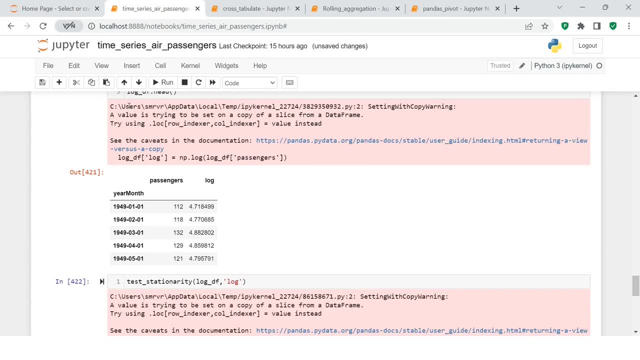 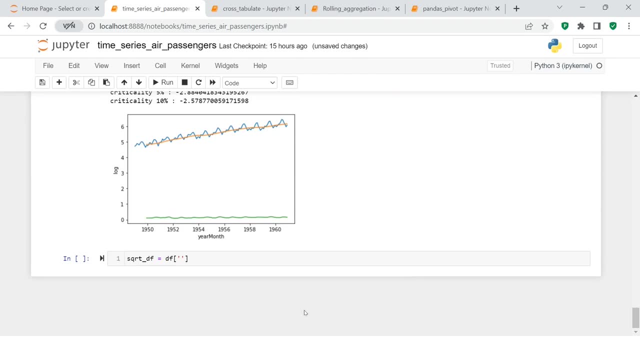 Oops, sorry, Here I have to use passenger again. I need to copy this, And here what I'll do is I'll just put it over here. All right, Let's have a quick look on this square root here, And how does this look like? 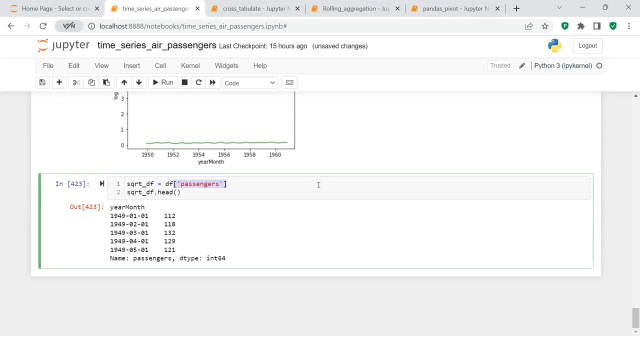 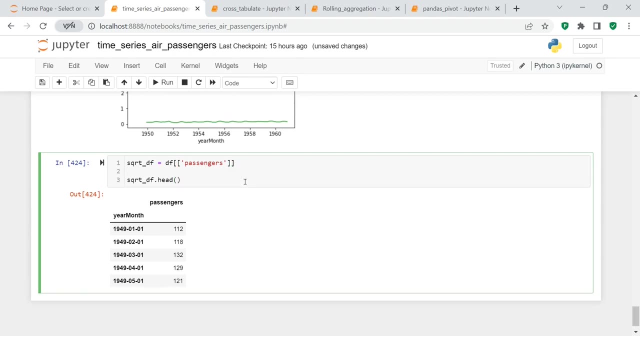 All right, So this is looking like a series. Now let me make it data. OK, now, here we have it fairly enough. Let's create another variable into it And I would say into this: This is q r t square root and n p dot s, q r t inside that. 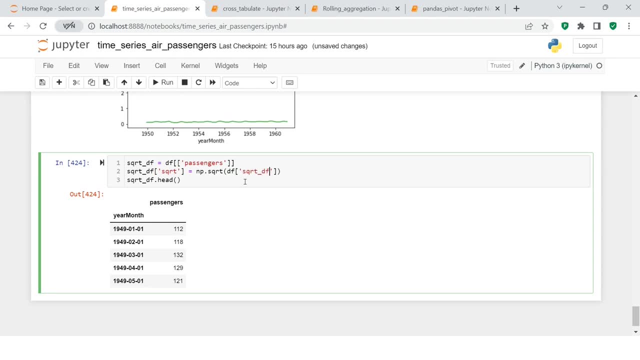 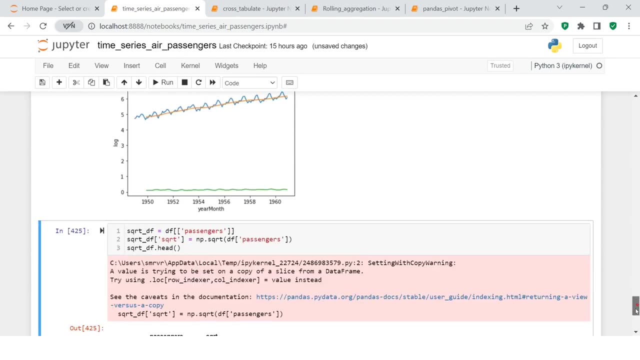 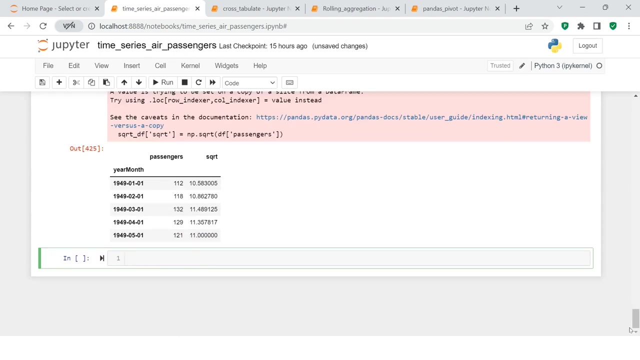 Let's just apply this variable, which is t, f, and this passengers, And now you just go ahead and have a look on this. Perfect. Now let's try to plot this. Now let's just try to check the stationarity on this data. 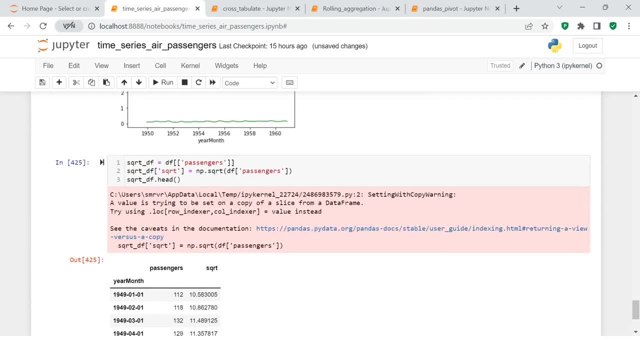 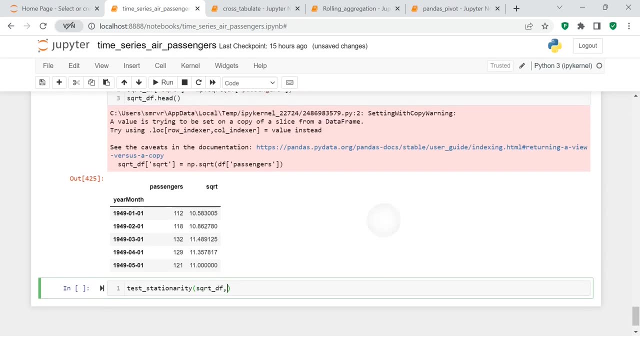 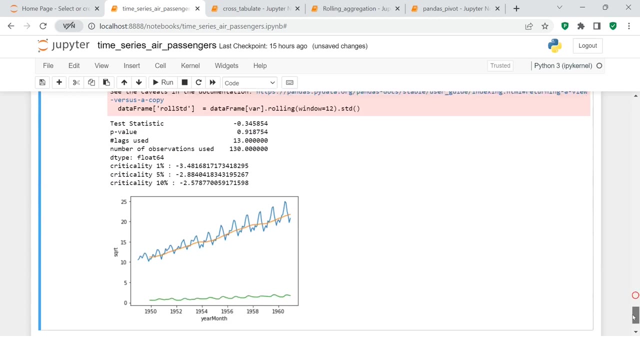 Best stationarity into this supply, this data, The data and frame name is s q r t t f. s q r t t f, And the variable which we want to use is s q r t. Let's just run this and see how does it looks like? 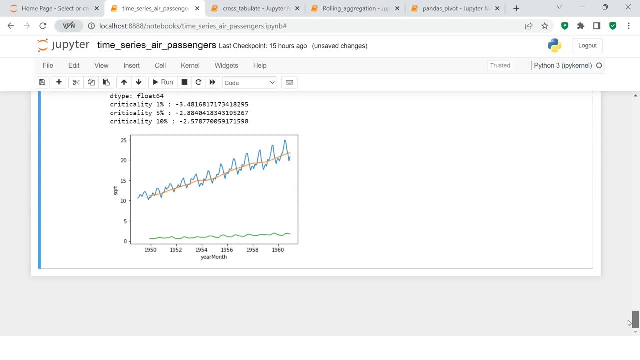 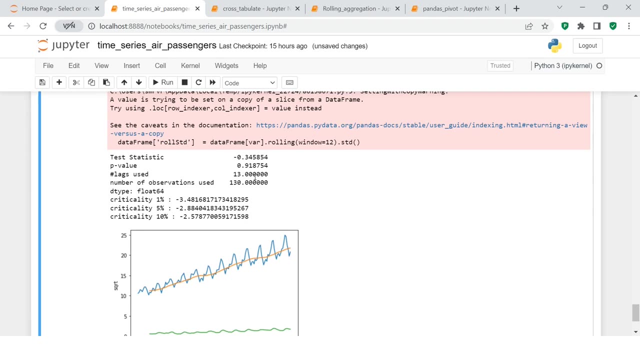 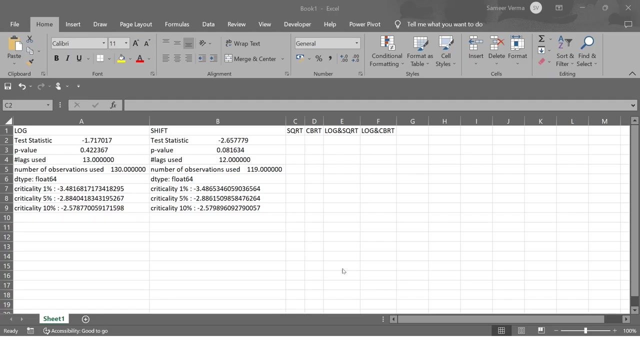 Oh, this is terrible. Not much better, huh? Let's have a look at the p value. that is zero point nine, And then this statistics is negative: zero point three, four. Let's just take this By looking at the graph. it is looking terrible. 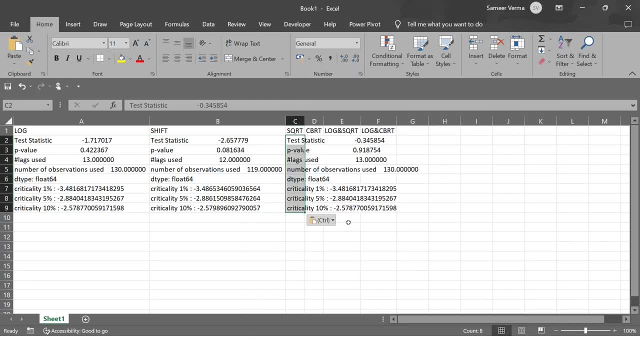 This was the square root method. Here we got that also. Now the next thing which we can try is cube root. Still, the shift thing is looking better. This is: this has the value of zero point zero eight, And here it is zero point nine. 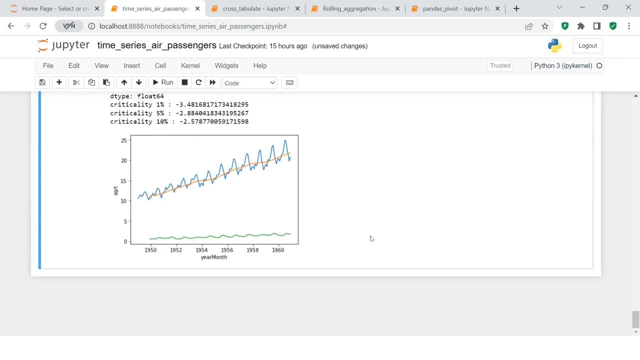 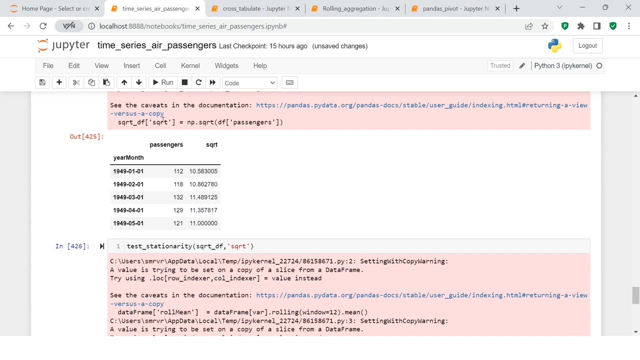 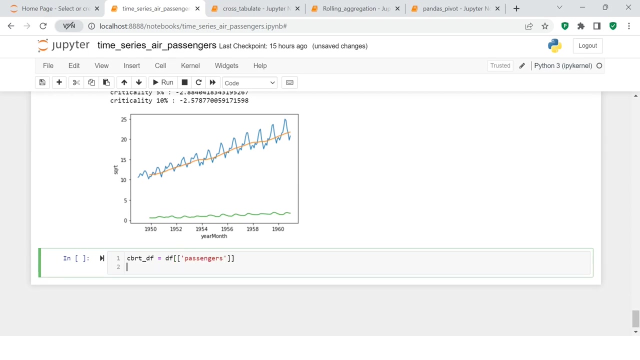 All right, Let's move ahead and try the next one. Next one we're going to have is: Let's take cube root, underscore t f, And here I will again take t f- subset passengers, T f- subset passengers, And let's just have a look at it. 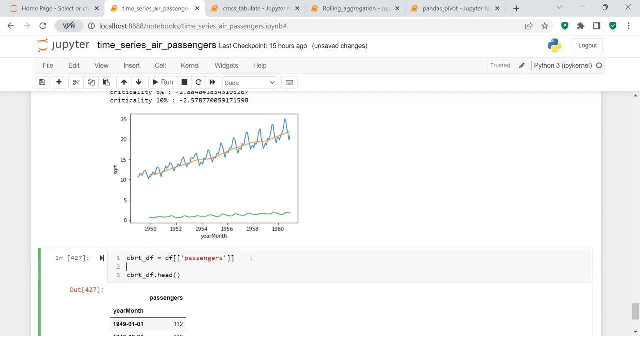 And this is how our data looks like. Now let's create the variable in this way. We will say: cube root equals to t, f And into this I just need to put this in: and p, dot, cube root And p is nothing but numpy library. 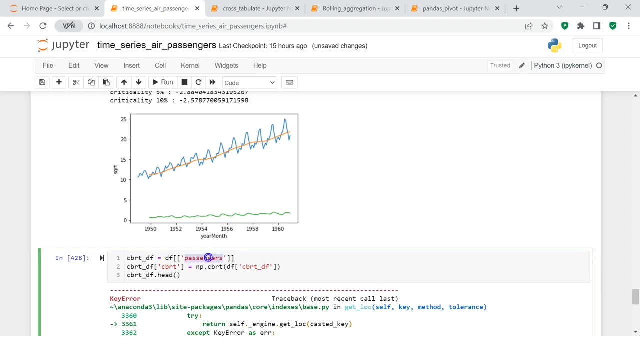 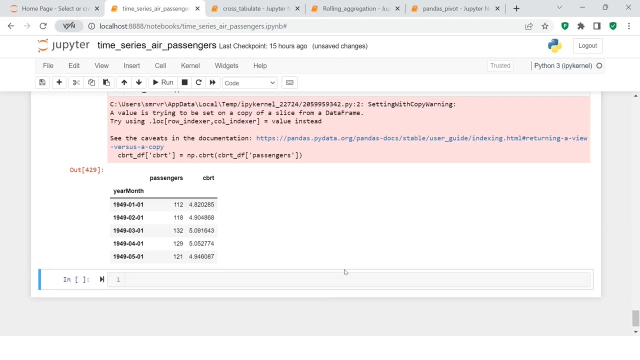 OK, All right Here. I got some problem and the problem is right here. Instead, I should use this as the data frame. Now we got it right. Here is what we have. This is cube root. OK, Now, after finding the cube root. 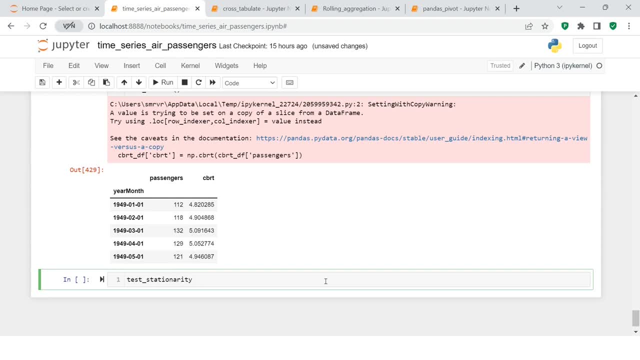 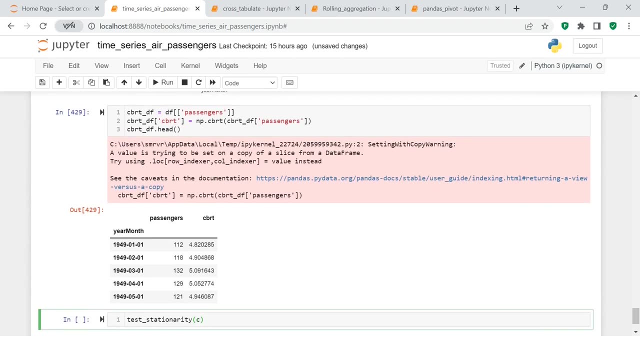 the next thing which comes is testing the stationarity. All right, Now let's just go ahead and test the stationarity. The data frame name we are going to use is cube root, underscore t, f, And the variable which we will be using is this: 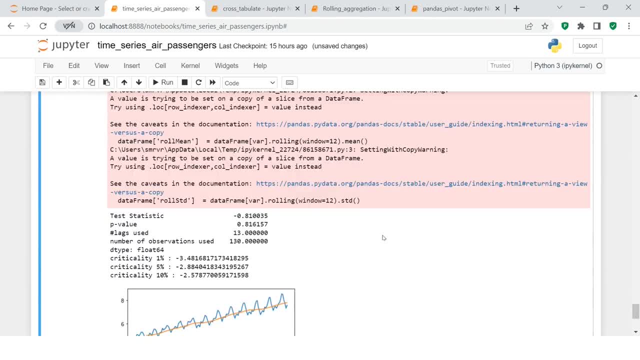 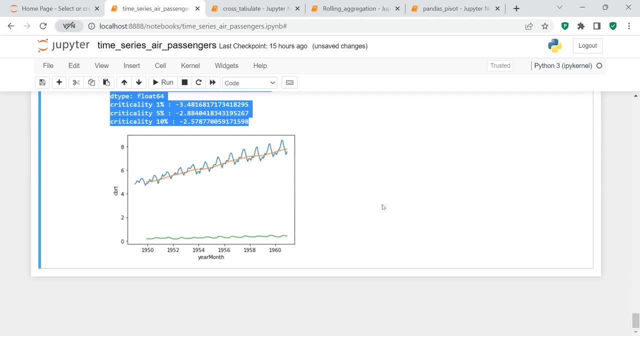 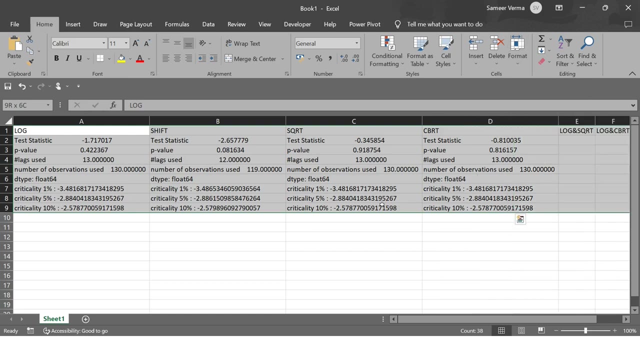 Now let's just see how our data looks like. Now. this is what we get over here. Let's by looking at the graph, it is not looking much different, But let's just see. how is it looking over here? All right, 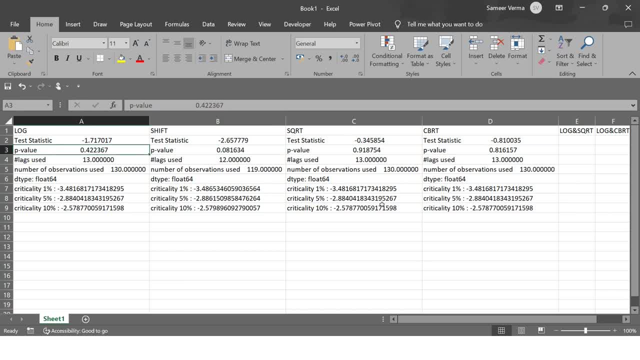 So if you see it has zero point eight, still the shift one is giving you the better result, isn't it? Shift shift method is giving you zero point zero eight p value, And this statistics also fairly close to it. Now let's just try to. 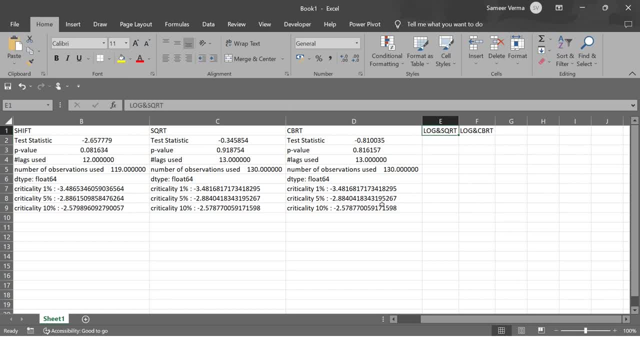 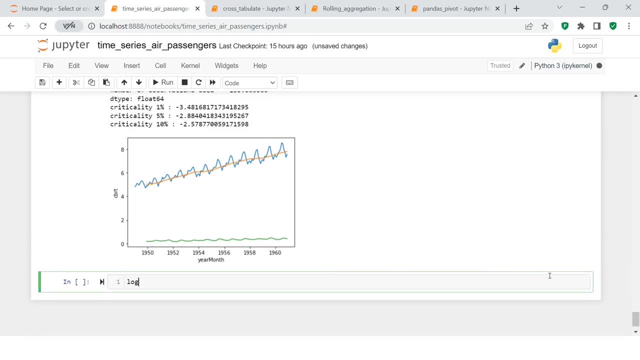 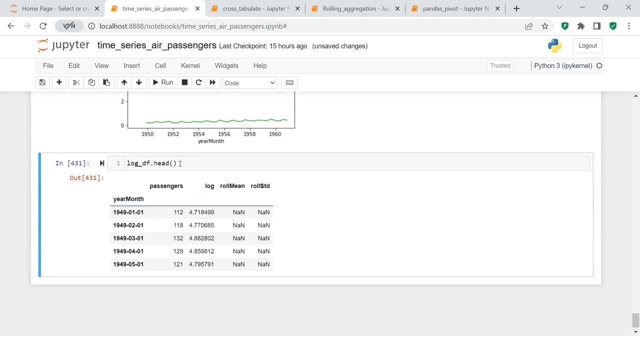 Combine log, square root, log and square root, both. So what I do is first I have the log df, log, underscore df, dot head. Here is what we have Now. let me make a subset and let's call it log df to log df, log, underscore df to. 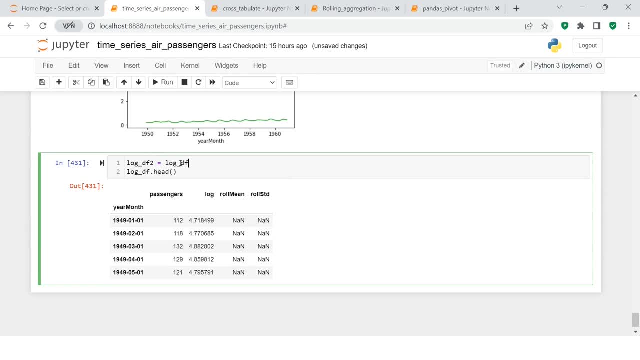 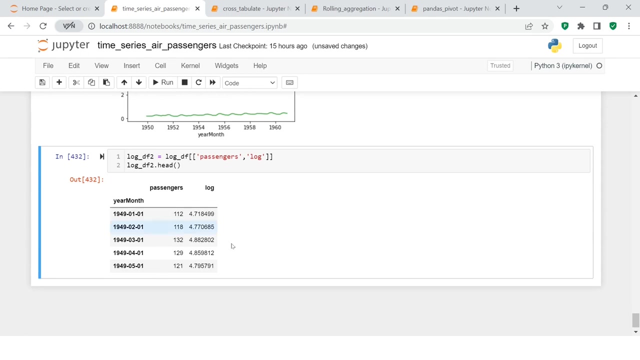 equals to log df, And out of that I will just take the Passengers And the log variable And let me show you the sample data. This is how our data looks like. Now we have to perform the square root on log variable. 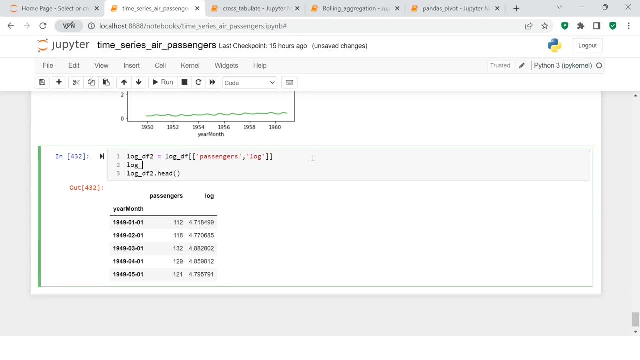 OK, so let's just say log underscore df to log square root. OK, and now we're here, Let's call it NP dot square root. inside that, what we're going to do is NP dot square root, and inside that I will use log df. 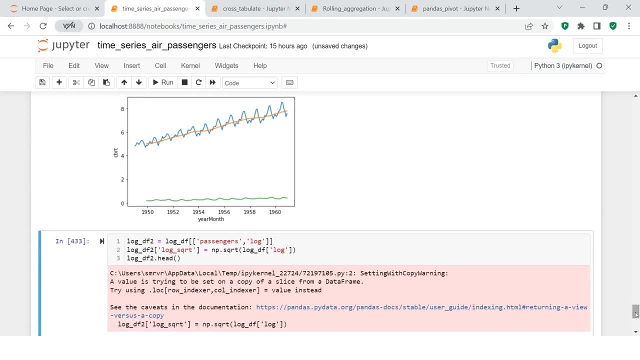 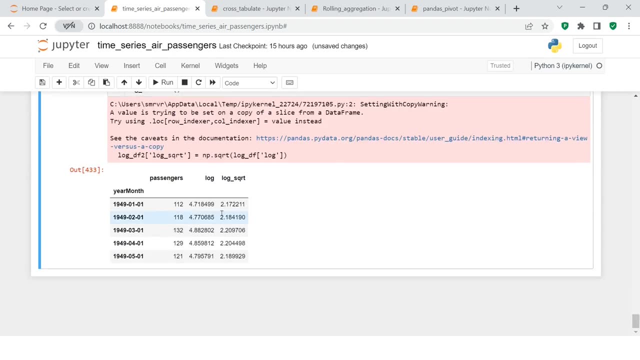 out of which I will take the log. So here we are, just trying to find the square root of this log data. Now the next thing, what you can do, is you can find the difference of these two, and then we can check the stationarity. 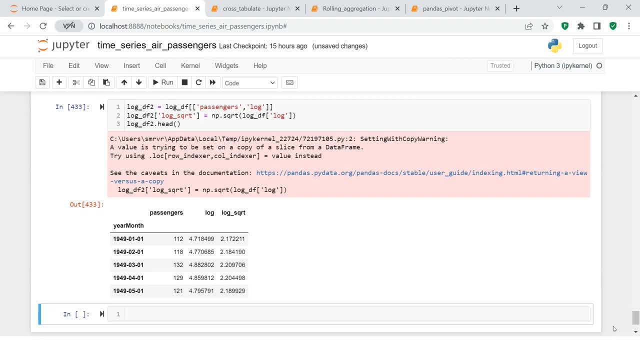 on top of, or maybe let's just try to figure out the stationarity on this variable itself. OK, because we have already combined two things Right. So let's just see how does it looks like? Test stationarity, And inside that I'm just going to put the. 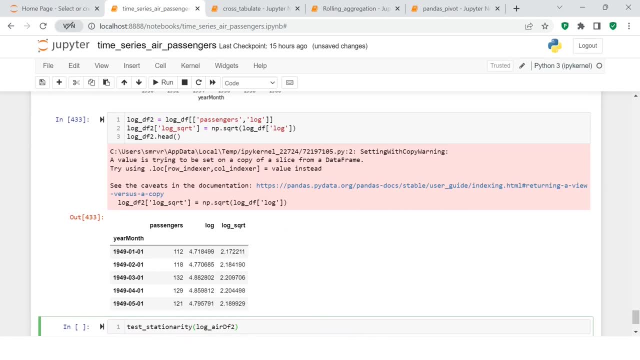 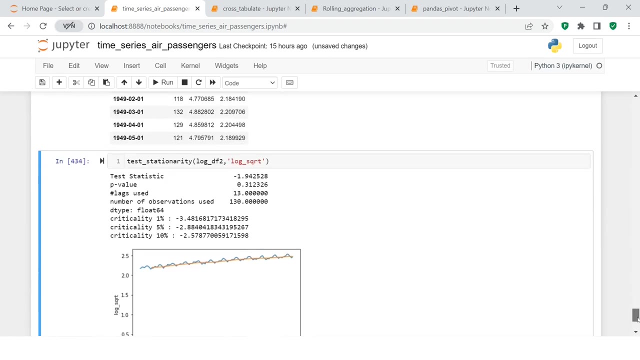 This particular data, which is nothing but log df two, sorry, log df two. And over here, the variable which I will be using is this: Let's just see how does it looks like now, OK, And what is the p-value? 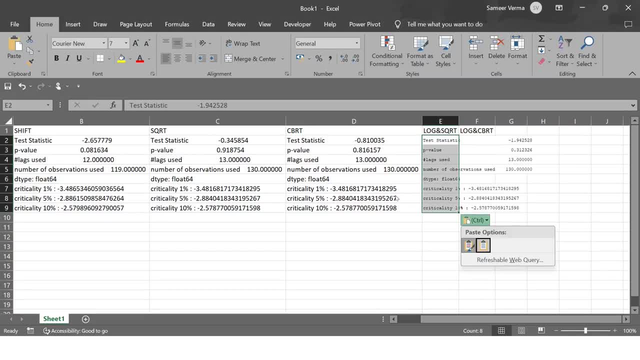 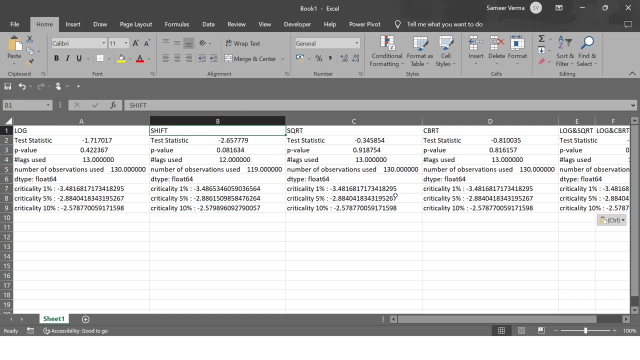 Here we just combined log and square root, OK. So p-value, It is giving us of zero, point three, which is still showing that shift method is doing better. Right, If you go by this, this test statistics: OK, And the test statistics also, you know. 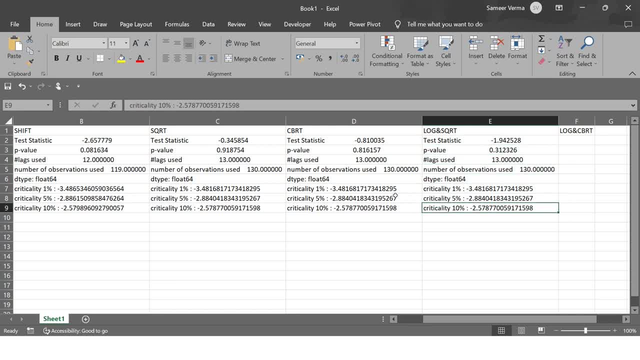 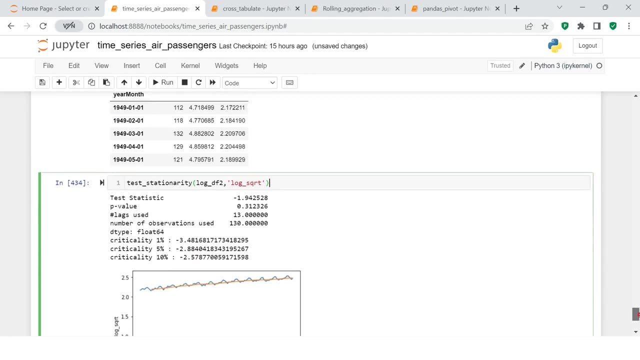 somewhere we can see it's close to this- criticalities. But p-value, you see, is still shift. one is much better. Now, what you can do over here is next thing You can try to, you know, shift this, this particular value. 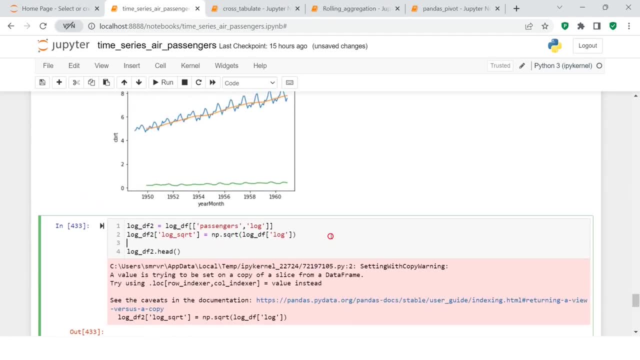 Let's just try this over here. What I'll do is log df two And let's call it log shift div, Log shift div, And over here they will say log square root. We are combining multiple things, So let's just see. 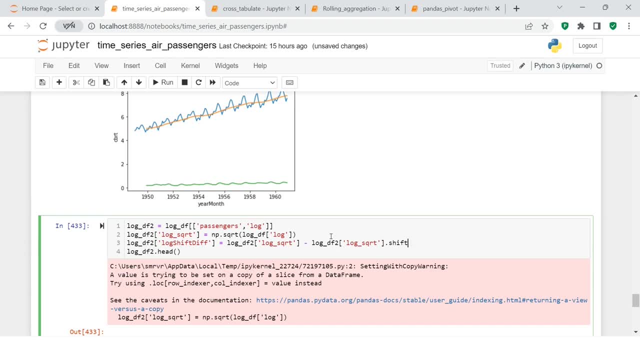 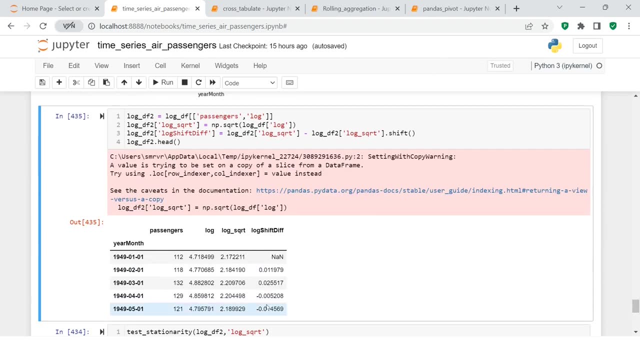 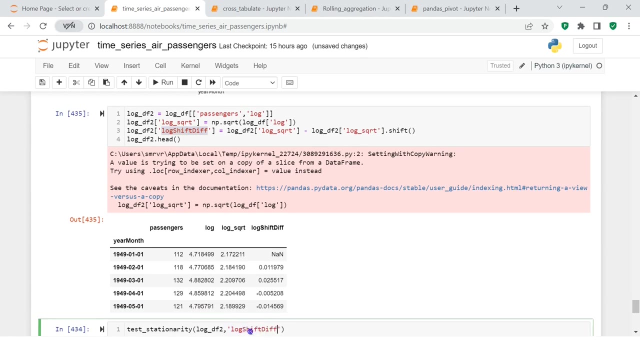 How does it looks like? Shift by one? OK, Now this is how the data is looking like. This is shifted. Let's see how does it behave over here. And we would have two variables already created inside it: Rolling, mean and all those things. 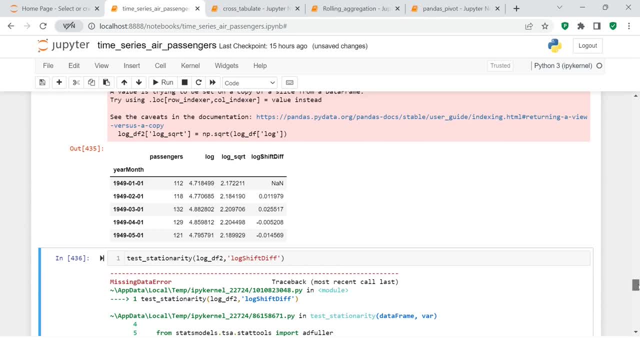 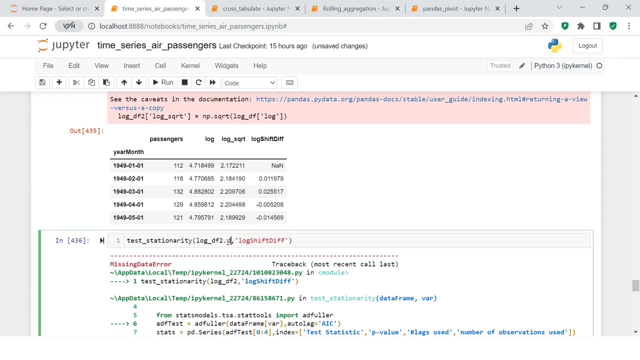 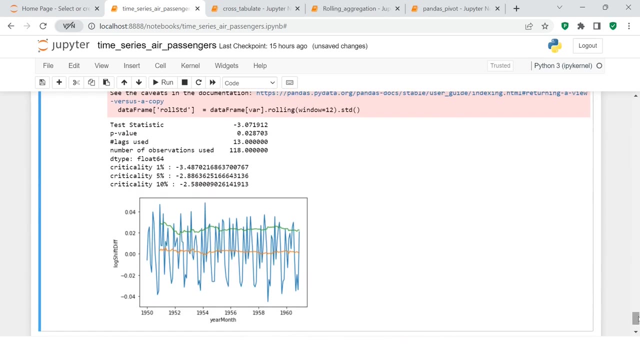 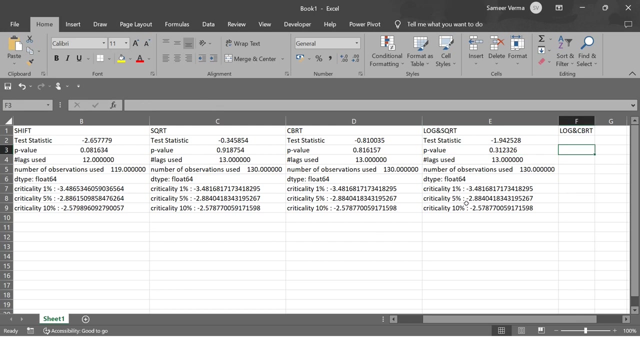 This is what happens. OK, It is saying something, And then problem. OK, because this shift value, Right. So here I would say: drop any. and this Is this working. Oh, it's pretty good, Isn't it? Now, if you take this, 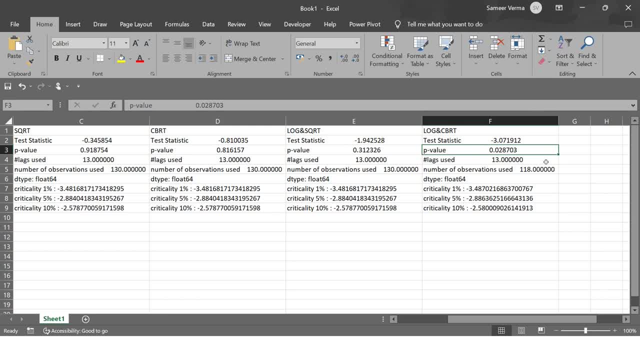 All right. So here the test statistics is three point zero seven, which is fairly close to criticality, one percent, and p value is zero point zero two, And the p value which we have for shift is zero point zero eight. So this is doing much better, which is log plus square root, log and square root. 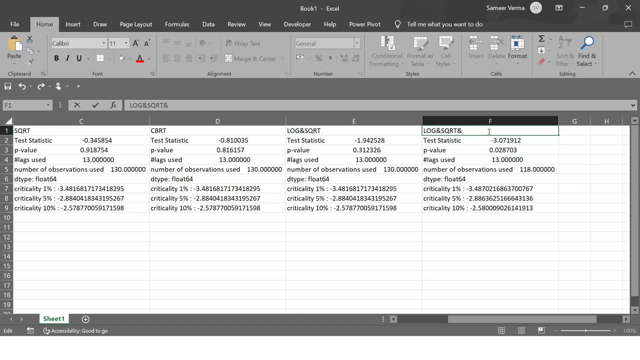 We combined three things over here: right, Square root, And then we combined shift as well, Right. So when we combined three things, we relatively got a much better result, Right. So this is how you can try different ways, Right. 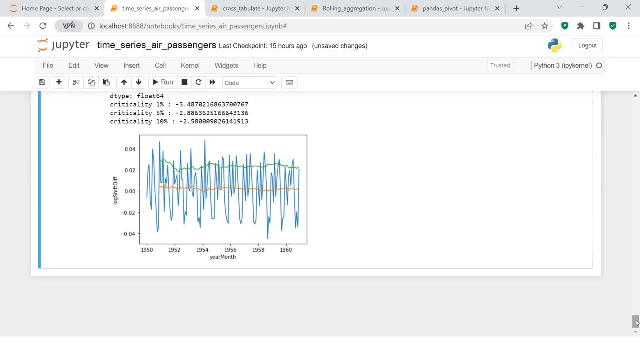 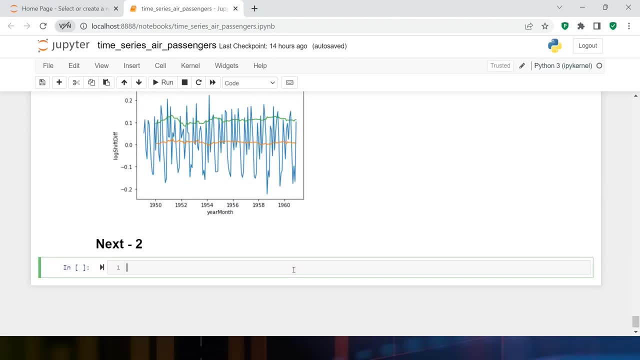 And then you will get, you make it a very good result And then, using that, you can move forward to build your model. to make the model, Arima is the best suited model for time series. to make the model, We can use either stationary data- the data which we transformed and made made it. 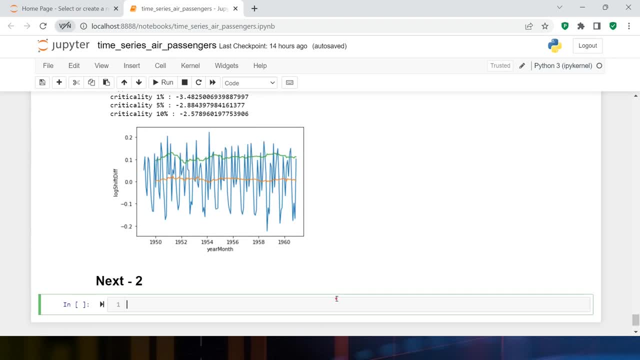 stationary or we can start with the original one. So I'm going to start with the original or base data. Once that we see, once we see that how to make the how to develop the Arima model, then we can try to build the same model on a stationary data or transform data. 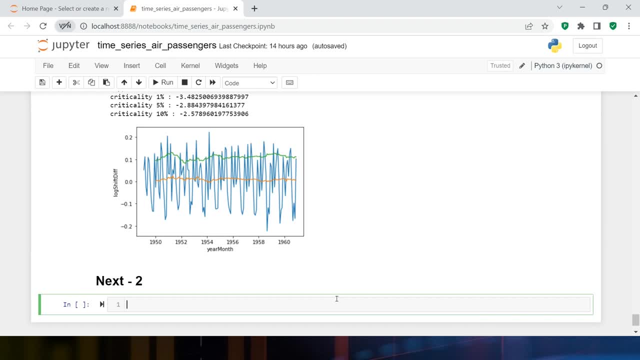 Why is that so? Because if you build the Arima model on a transform data, you'll have to again transform it back to the actual form, which will take some time. And, and just to avoid any kind of confusion, I'm going to start with the base data. 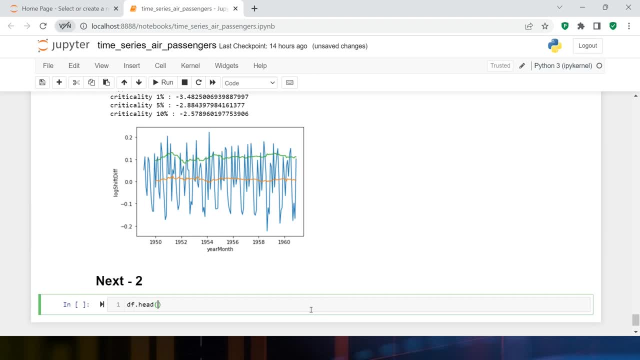 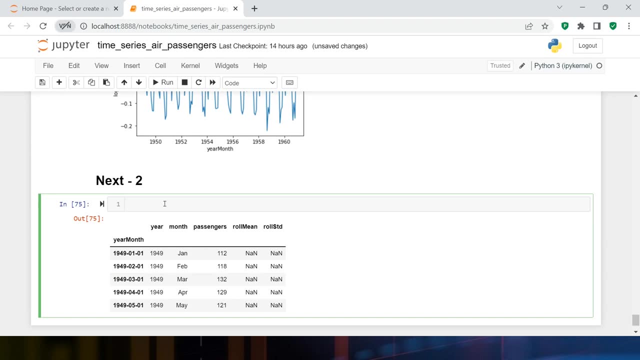 So, before we start, let's have a look on our original data. This is: this is how our data is looking like Right now. let me make a subset of it. subset, I will say: ARP data, ARP, ARP. Let's call it ARP. 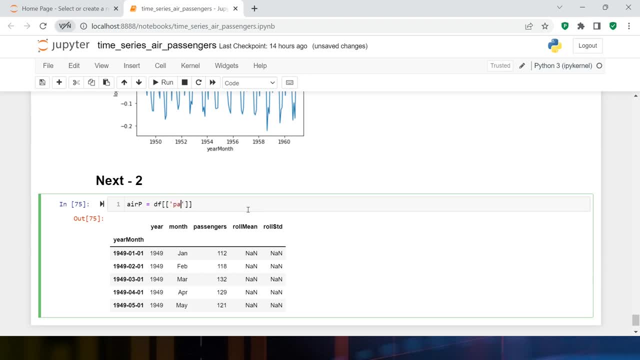 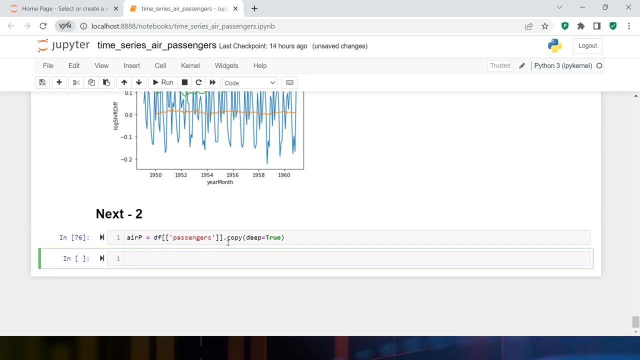 OK, And then out of DF. I am just trying to passengers, I will do copy, and here I would say deep equals to true, so that my original data remains unchanged. So I'm done with creating this data frame ARP dot head. This is it. 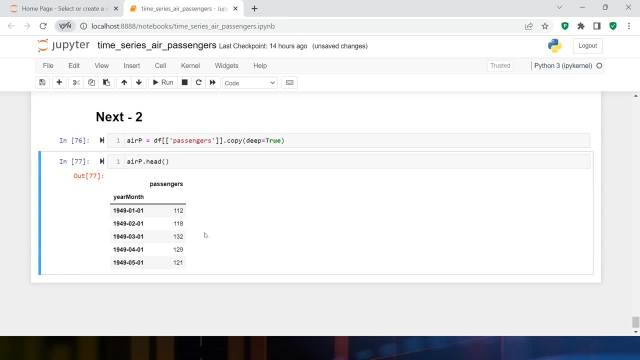 Now, once I'm done with this, I will create two more variables into it, where I would differentiate by one And I would differentiate by 12 as well. Why by 12? Because in the beginning, we saw that the data is having trained pattern as well. 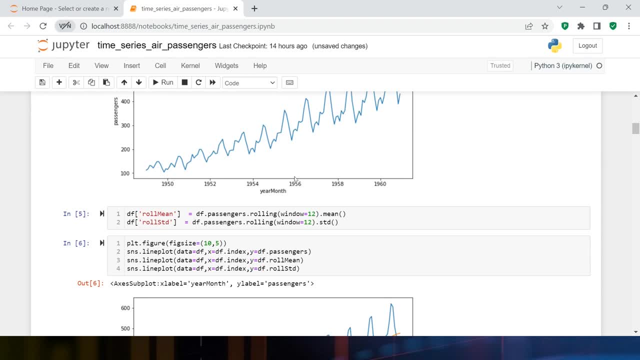 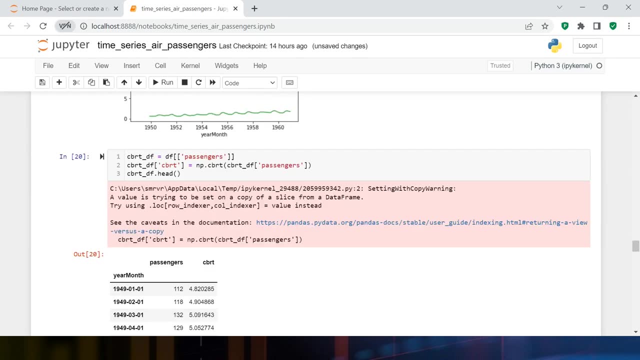 as seasonality right, and this seasonality is on 12 months. If we do it on, if we differentiate by 12, that will help in reducing the seasonality. OK, so that's why I will create both of those variables over here and as and when. 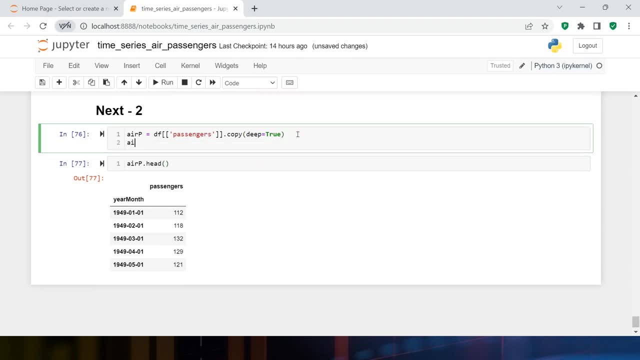 needed. we will use that. OK, now here let's call it ARP difference. One first difference. Let's call it first diff, And for that I will use ARP, ARP, dot passengers, And here I would just say diff. So in this you don't have to use the shift thing and minus thing, it does rest of the things. 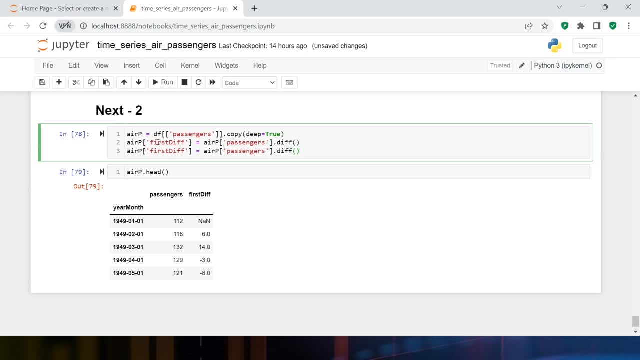 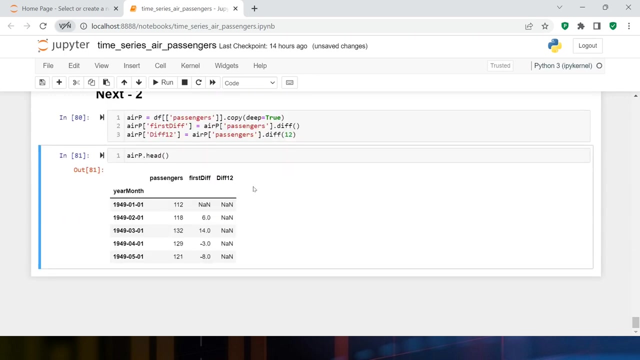 automatically. OK, now the next one which I'm going to create is diff 12, 12 diff, Let's call it, or maybe let's call it diff 12.. And in this I will put 12.. OK, now, here is what we got. 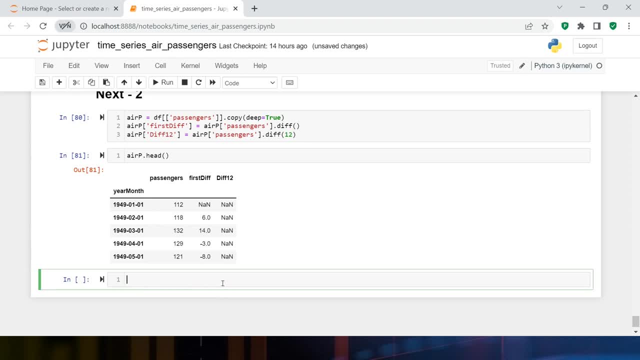 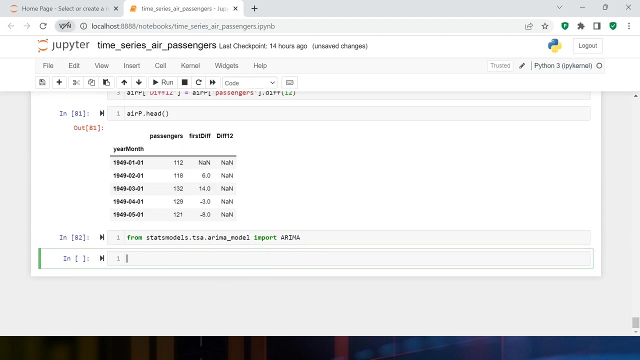 Next, we are going to start with building the ARIMA model. to build the ARIMA model First, we need to import this. So we're going to say from start: modelstsaarimamodel, import arima. OK, I'm done with importing this. 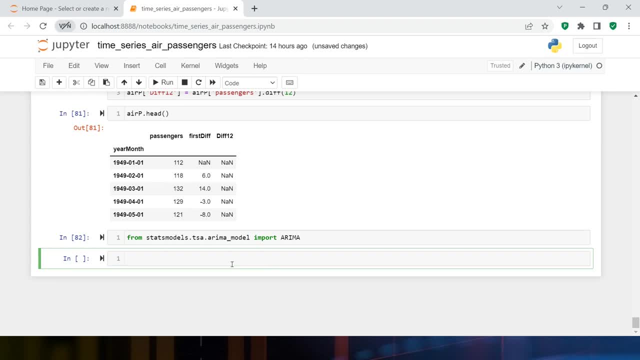 So I will not import all the libraries at once. I'll import them as and when it is needed so that you would have the context which library is needed for what purpose. OK, now, once I'm done with importing this, I'm going to build the model. 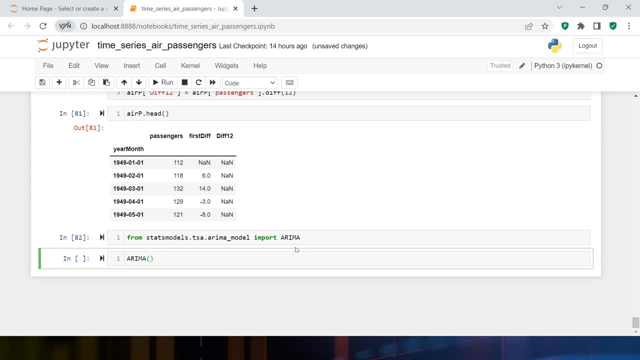 So, when you build the model, first thing which you need to provide is the data, And for data, we require the train and test data. right, Train and test data. Before I reach to that point, let me just show you a version. 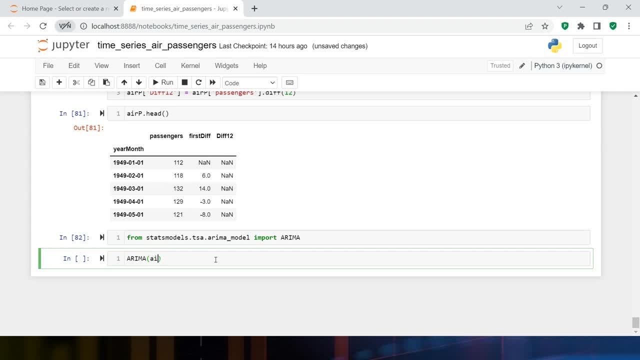 OK, so over here I'm just going to use let's, let's, for example, let's try to use this data, and after this, what we need to use is let's see all the parameters. So you see, here you have to supply data and then you have to supply the order. 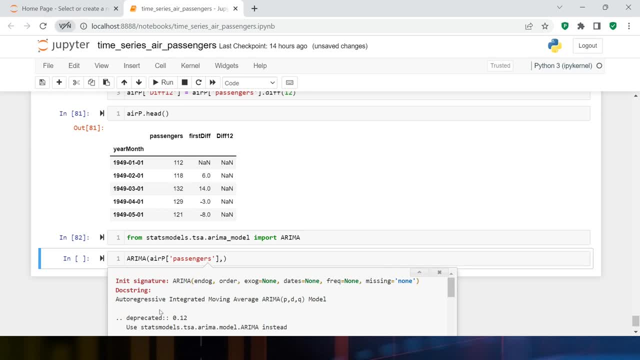 So for order, you see here it also says autoregressive integrated moving average. So this is the full form of your Arima model And that takes PDQ as order. If you come over here for order, we require PDQ. 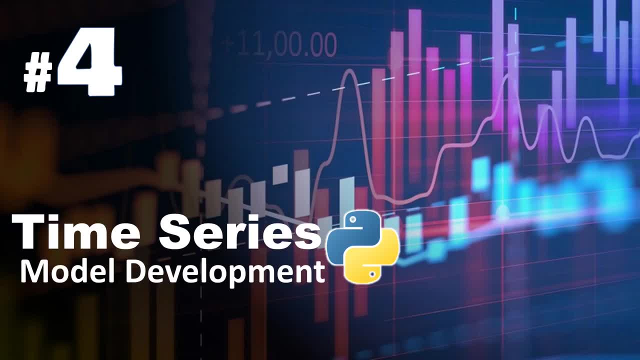 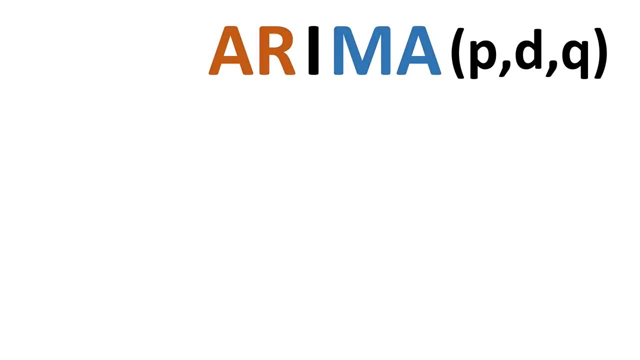 Now let's try to understand what exactly this is right. So for that I'll take you over here. Here, if you see, Arima itself is a combination of three models. One is AR, then I, then MA. Let's understand each of them. 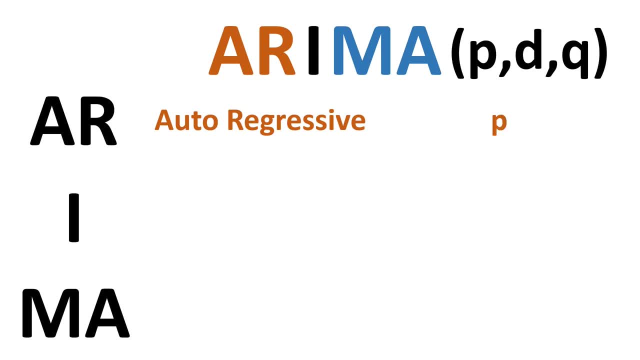 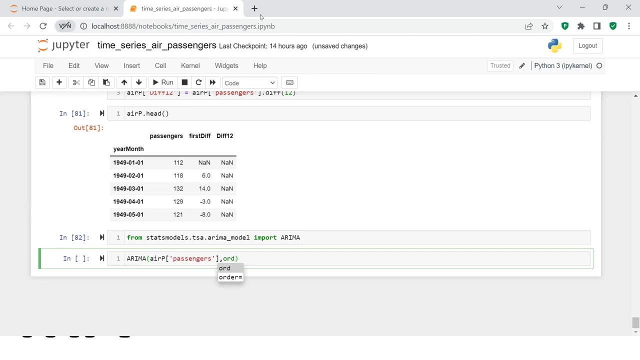 AR stands for autoregressive, and it is indicated by P. I stands for integrated, and that is indicated by D. MA stands for moving average, and that is indicated by Q. So this is how we call it: Arima model. Now let's try to understand how to get the value, because here in the model you need to supply. 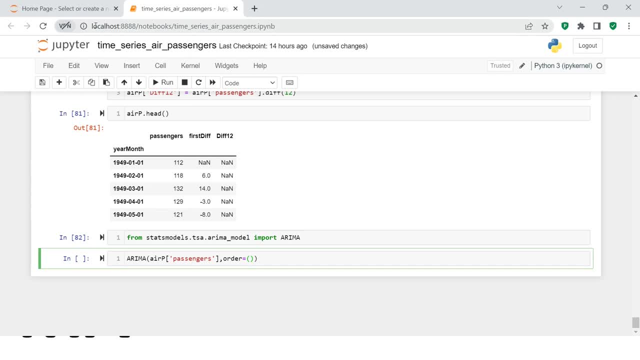 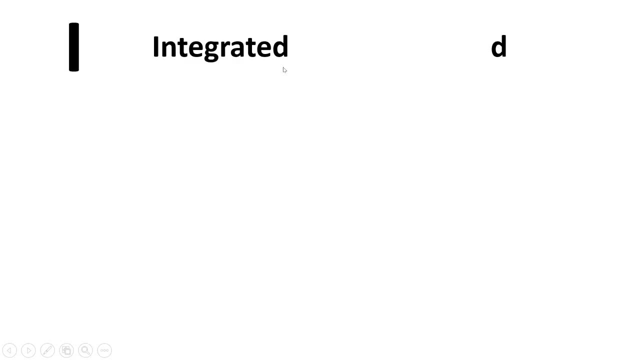 You would require to supply the value for order, So the value which you would be supplying, that will be for PD and Q. Now let's understand how to find its values. So, to find the value first, let's start with D. D is nothing but integration. 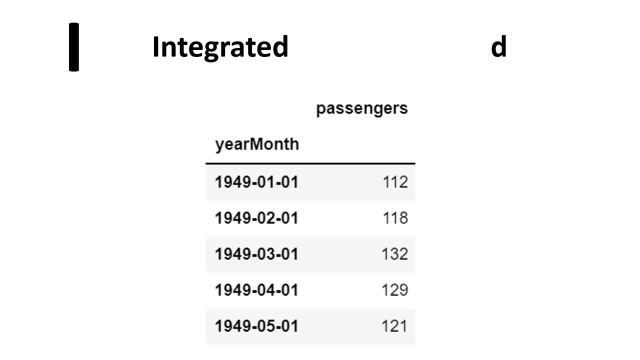 So what does it mean? You remember, this is the, this is how we have the data frame And when we differentiate it, this is how we get right. We just shift it by one and then we find the difference. So by how many steps? 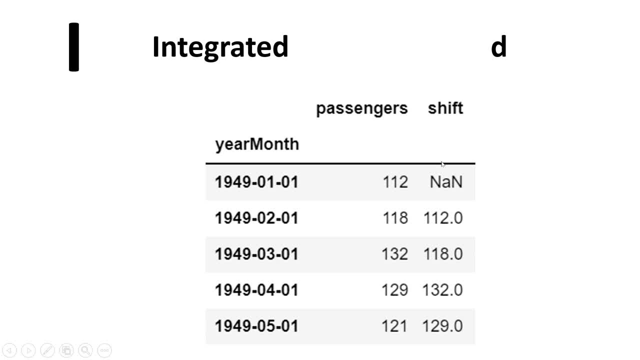 We are shifting it one, So here the value for D will be one. When you shift it for 12 months, the value for D will be 12.. What, by whatever interval you shift, the data that will go in D. Next comes is autoregressive model. 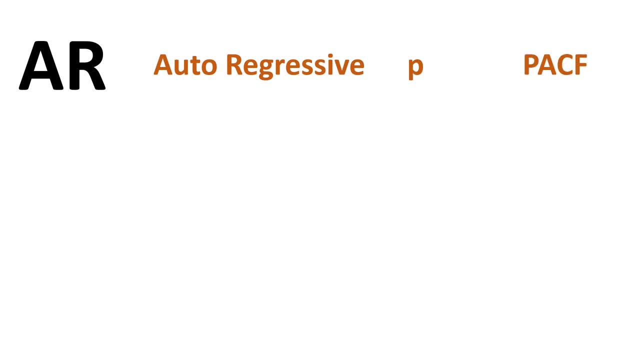 So to find AR value, we check the PACF. PACF is nothing but partial autocorrelation function. OK, then comes MA moving average, Which is indicated by Q, And to find that we use the ACF. Now I will not go in mathematics. how to find this mathematically? 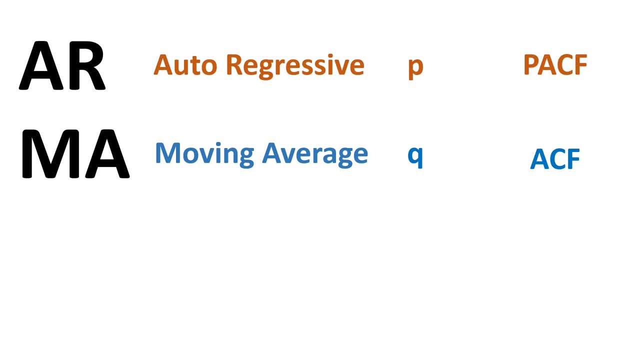 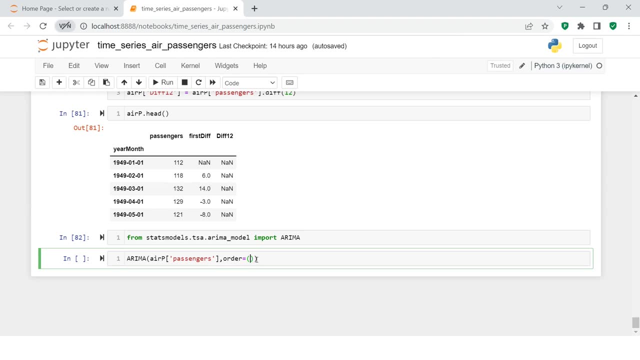 To keep it simple and specific. I'll try. I'll go and try to find it in Python itself. OK, now let's go back over here. So here we require the order values for that. What we need to import is from stats models. 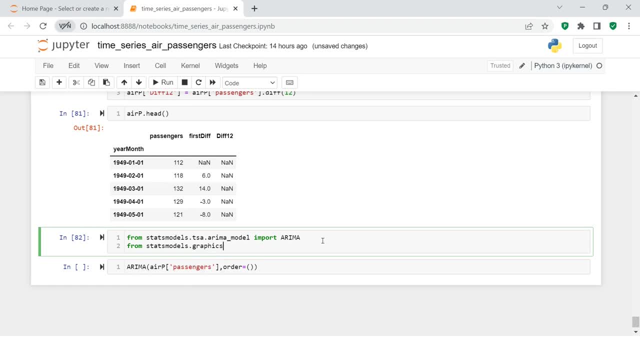 graphics, someplots, Plot tools, I guess. Import plot, Import graphics, Then it should be PSPlots, ImportPlotACF and PlotPSCF. Both of these two things I am importing. 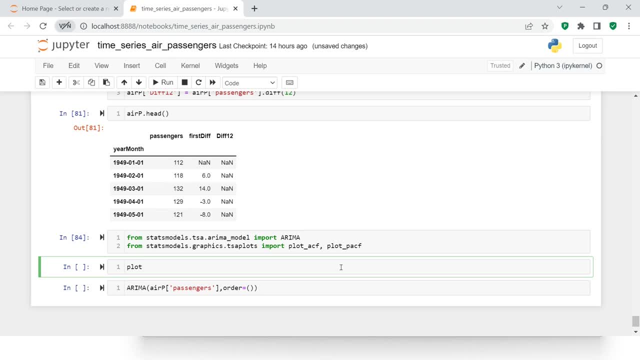 All right. Now, once we are done with importing this, let's try to plot the data. So first we are going to build our ARIMA model in context of first diff right. So here what I will do is I will use my data. 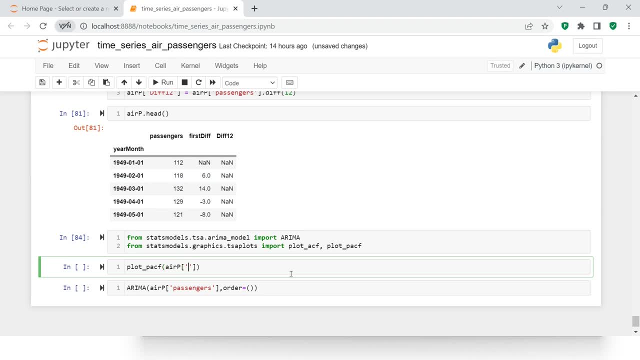 So let's call it ARP, and here the value which I'm going to take is passengers, Not passengers exactly. It will be first diff And because it has NA value, so I'm just going to say drop NA, Drop NA. I'm just waiting for it to complete. 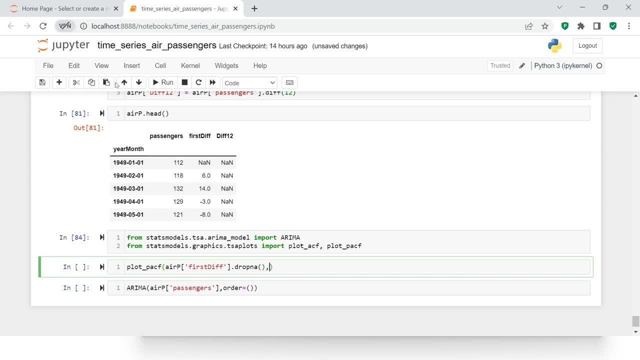 To do the auto complete, otherwise it will just give you the error And then it takes the value for lags. So I'm going to keep the value for lags is 20.. If you, if you want me to cover this thing in detail, let me know in the comments. 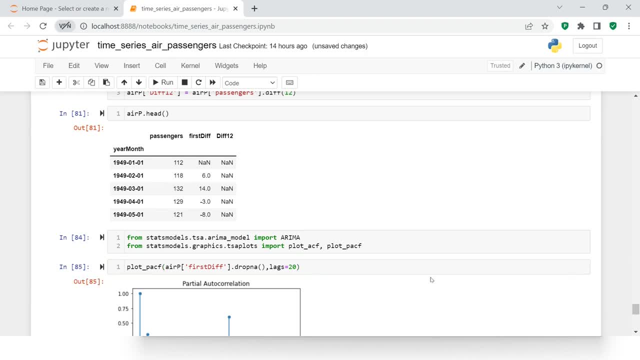 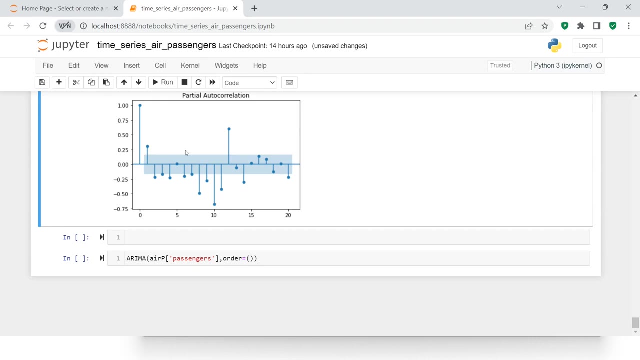 section. I'll try and cover that in detail, make a separate video for that. So here is what we got for PSCF. So let's see how to find the PSCF value. So you see this shaded area, That is insignificant area outside a area outside of this shaded one. 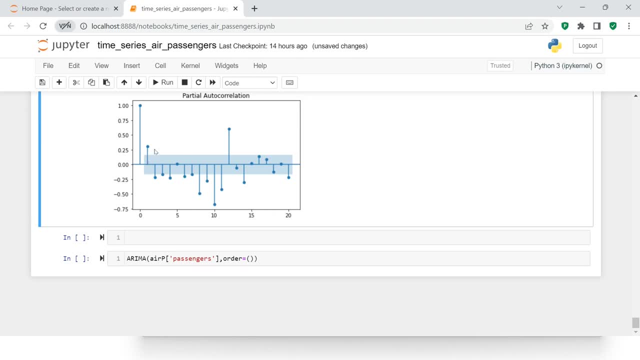 That is called the significant area. So the point where these lines are exceeding to this insignificant area, that that is something which we're going to consider Right. So this is zero. This is one. at first it is exceeding. Then here at downside, also here also it is exceeding. 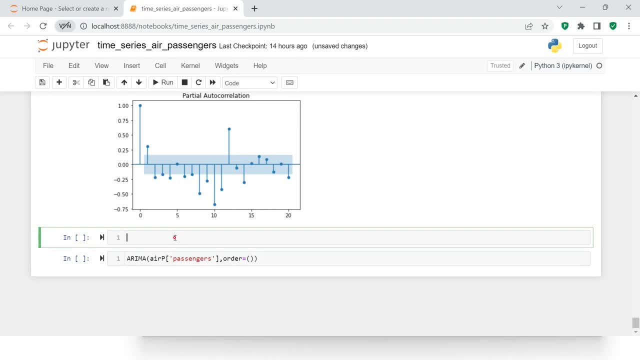 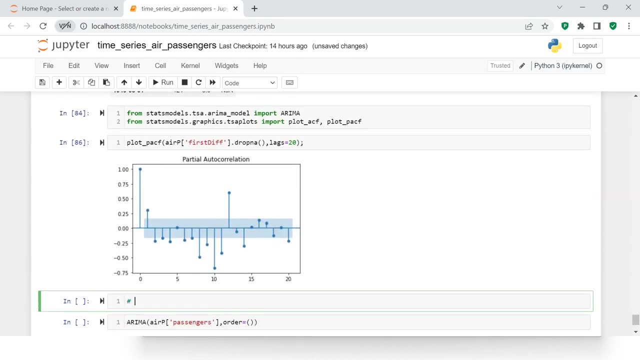 So we can try different combination of it. So first, P value which I'm going to take is: this is the value for P. All right, PSCF. So value for P I would have is I would have. value for P is one. 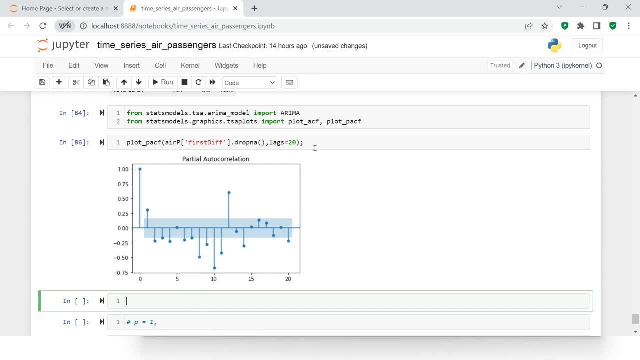 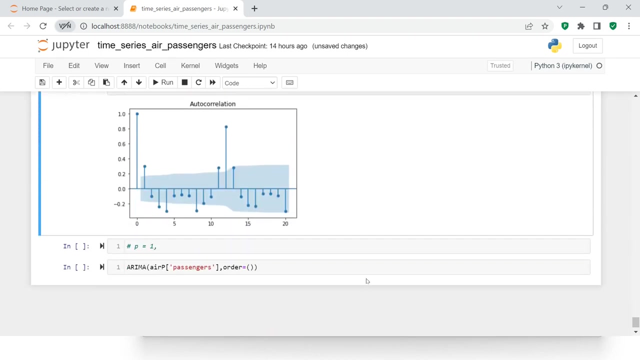 OK, now let's try to find the value for Q, because for D we already have the value. So to find it we're going to say plot ACF And the same thing. OK, rest of the things are going to be same. 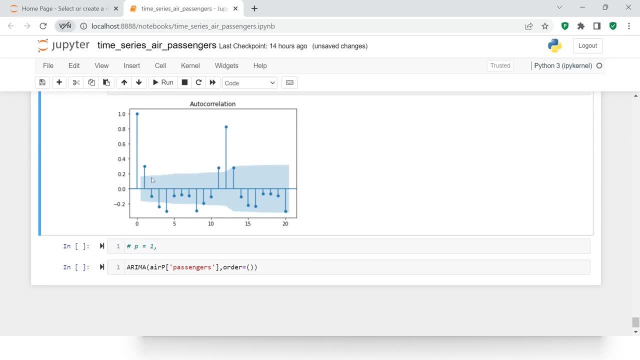 So here also it is saying the first one is out of the insignificant area, Then second is nothing and third Right. So I can try with first and or maybe third Right. First, second, third, I can take it third as well. 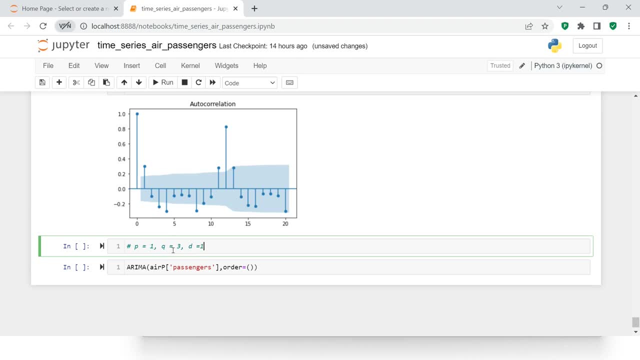 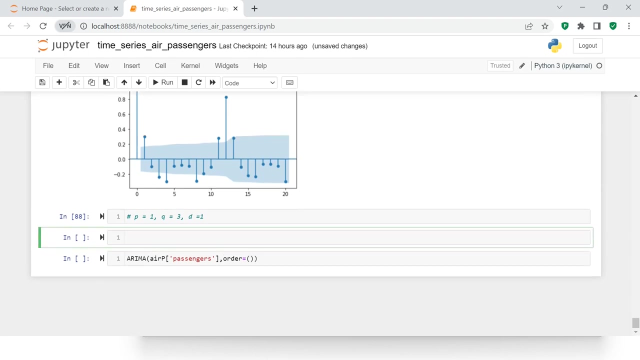 Q equals to three and D value for D we already have as one Right Now. this is The value which we got for the PQ and D or PDQ Right Now. next thing which we need to do is find the. I mean, make a trend test trend, do a trend test split so that, on trend data, 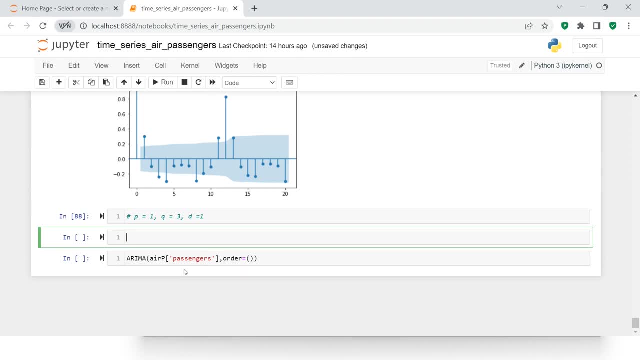 we will train the model and then, on the test data, we will test the model. Now let's start with making the trend test split. for that, The total length of data that I have is, that is, 144,, which is for 12 years, because we 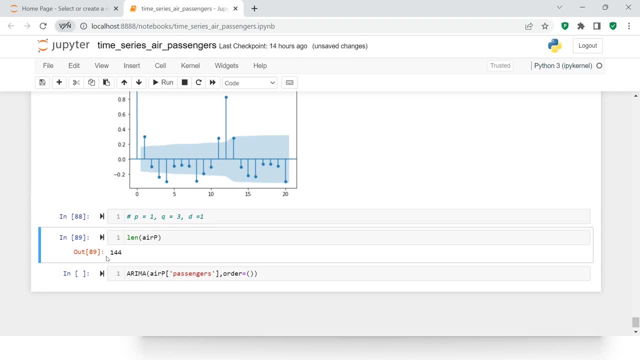 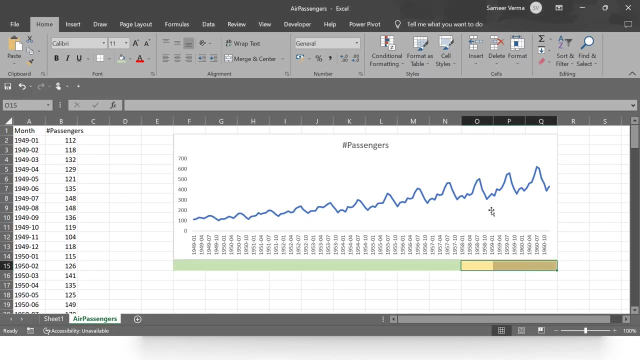 have the monthly data Right Now. I'm going to split 70 percent for training and 30 percent for test. How is that going to work? You see, over here this is the same data which I have plotted Now, if you see, starting from here till here. right, that I will. 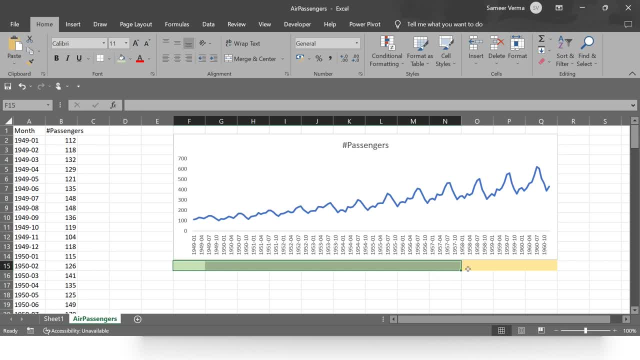 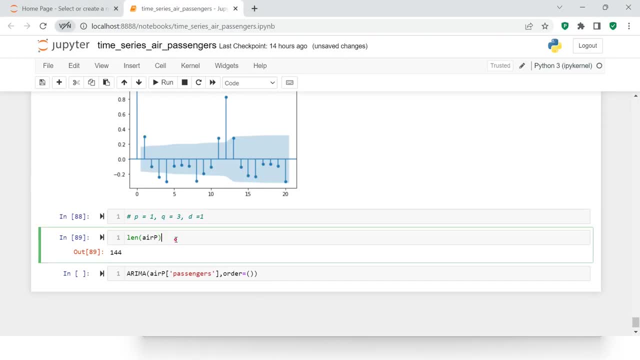 make as training data and the point where it ends. starting from there till the end, I will keep it as test right for testing data. Now let's just- I just hope that it was clear. Now let's find the 70 percent. 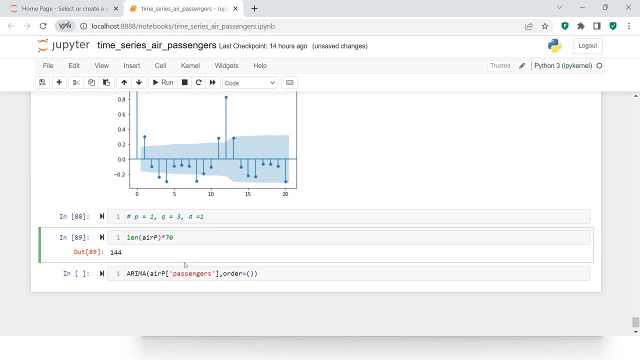 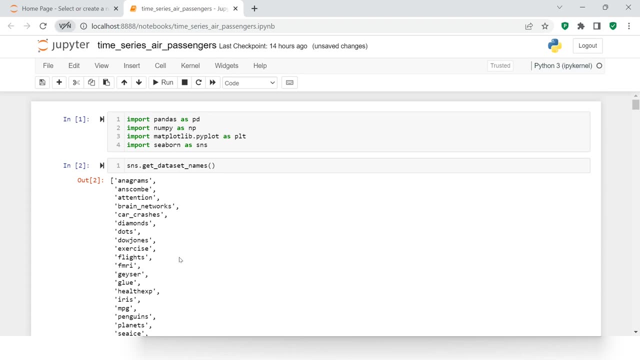 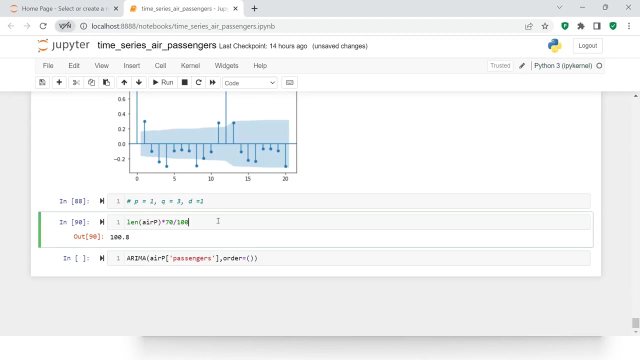 Of this data. So for that, what we're going to do is length of the data frame into 70 divided by 100.. Let's see what comes. It is coming one hundred. Sorry, It is coming one hundred. one hundred. point to eight. 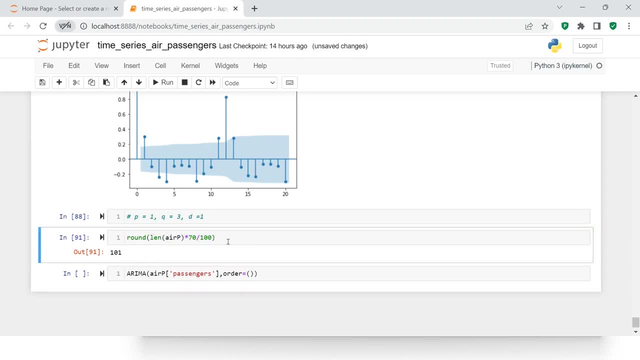 Now we need to make it round, Right. So this will be one hundred and one. Now the time comes when we should fetch the train, data Train, And for that I'm going to say air, air. be starting from beginning till till this point, Right? 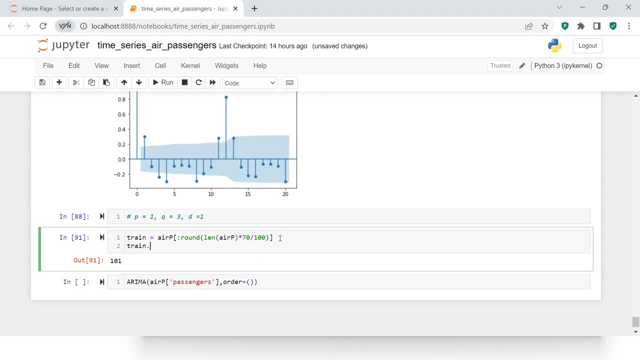 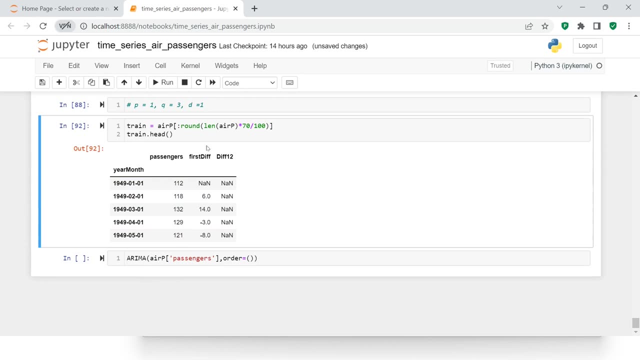 That will go in train data. Let's just see how does it look. Train dot head Right. So it is starting from this one hundred and twelve and will go till the end. Let's see where does it ends. Tell So here it is ending at May fifty seven. 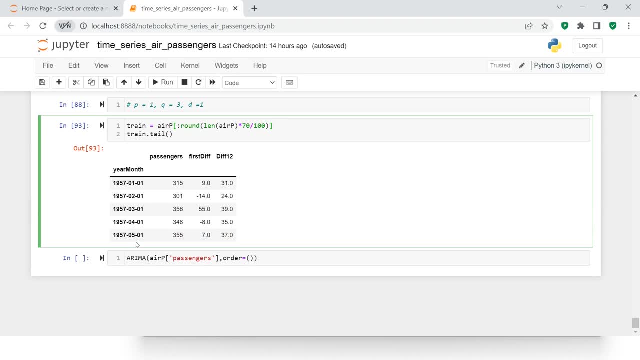 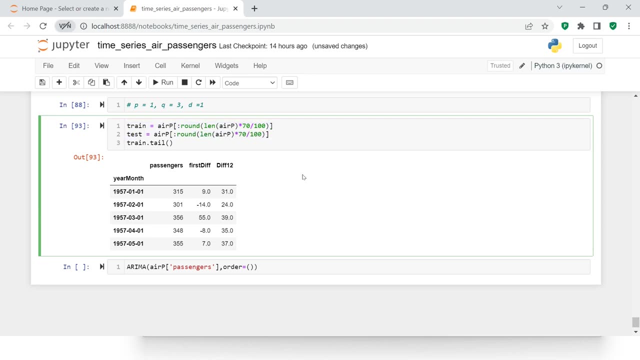 Now our test data should start from the month next to it, which is June nineteen, fifty seven- Let's make that here I would say test data, And in this this call on. I will start this call on from here and I'll just put it here. 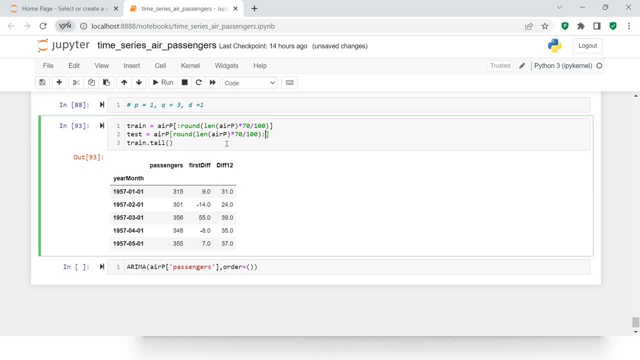 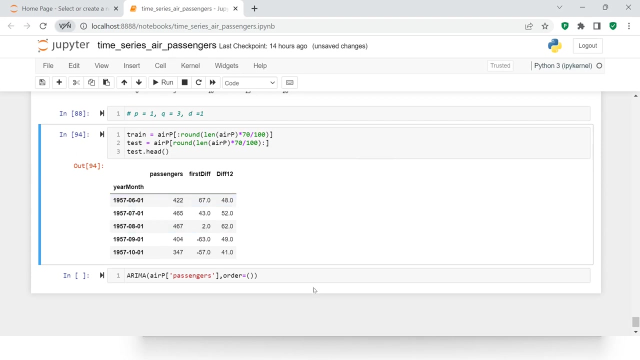 Here it says: start from this point where 70 percent is ending. from that point I want to start it, And here I will check Test dot head. All right, So we are good over here. Right? So here you see, we are getting the June. 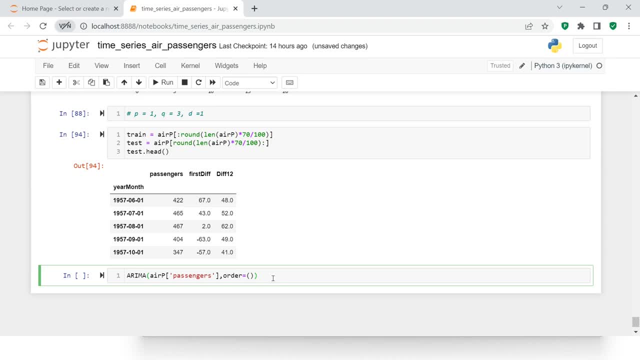 Now let's just start. now, Let's just start with the actual model bending. OK, now, here I would use train data instead of what is, I mean full data, And here we are taking the passengers. Please note, we are not to to train the model. 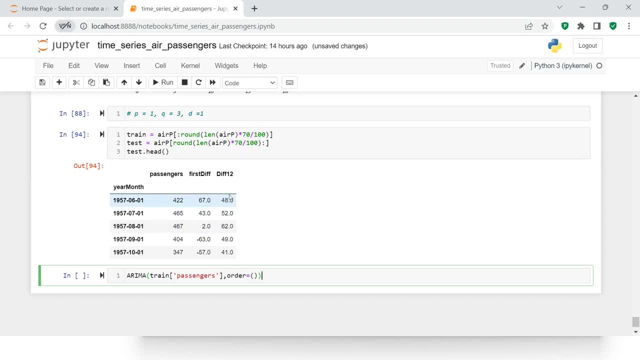 We are not taking this difference data, that. that is something which we just we use to find the value for P, D and Q. Now, for P, the value which we have is one, for D, We have it one, And for Q, we have it three. 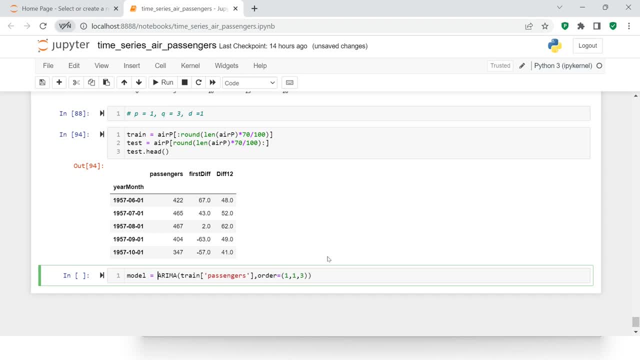 Let's try to fit the model. Let's try to have the model object created. After that I'm going to fit the model. So to that I would say: model dot fit. model is fitted. Let's see if it gives any error. 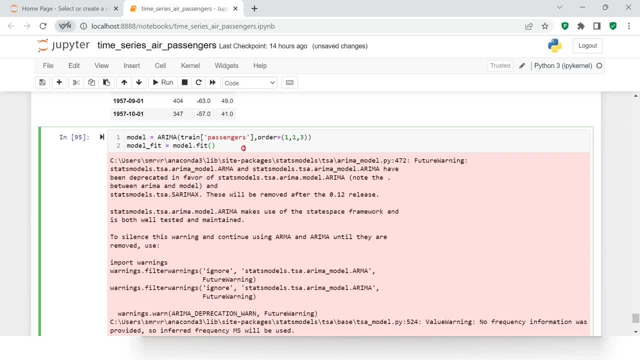 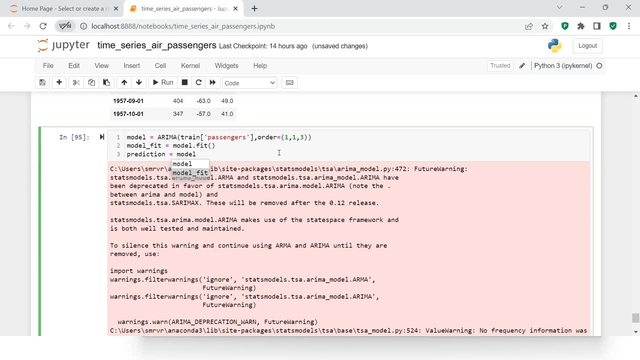 Looks good. Just ignore this warning, Don't need to worry about it. Now I will make the prediction, And for that I would say model dot, fit dot, Predict, Predict, And inside that I need to supply the data on which I want to make the prediction. 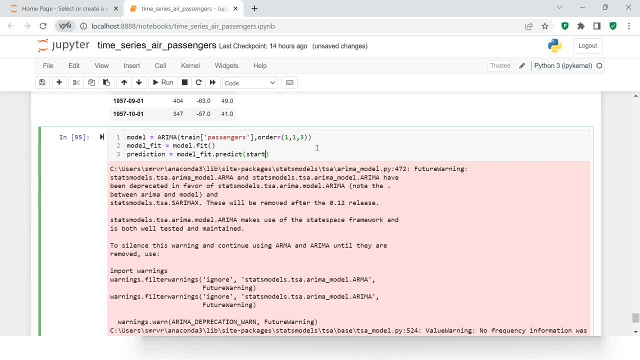 So for that there are two parameters. we need to provide the start point. Start point will be test Dot index zero, So we want to make the prediction on test data Right. And then we need to provide the end point, And for the end point I will use test. 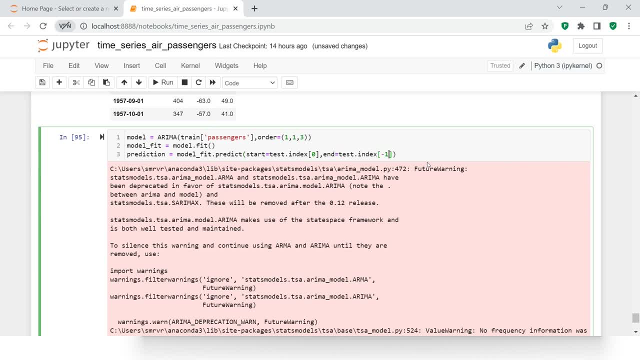 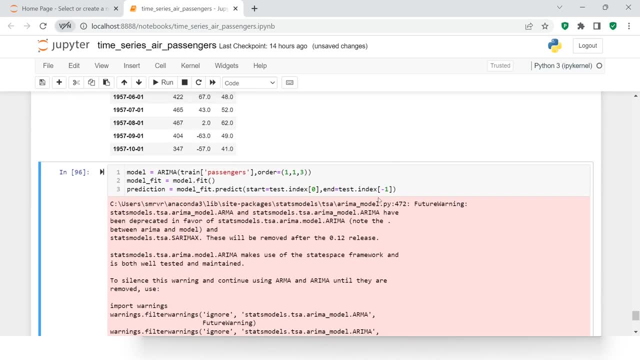 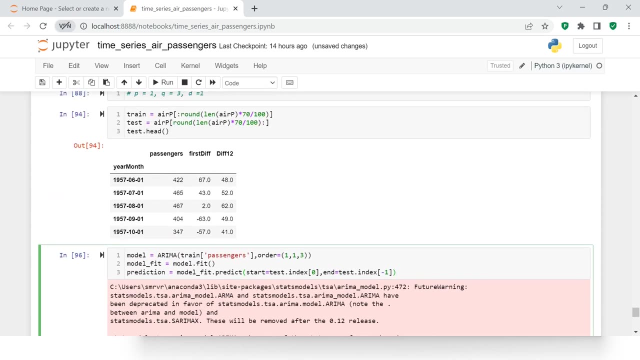 dot index minus one. Let's see if this gives any error or works well, Working well, OK, Now, this is the prediction which is created. Now, the next thing which comes is putting it in the data frame, the data frame which we have over here. 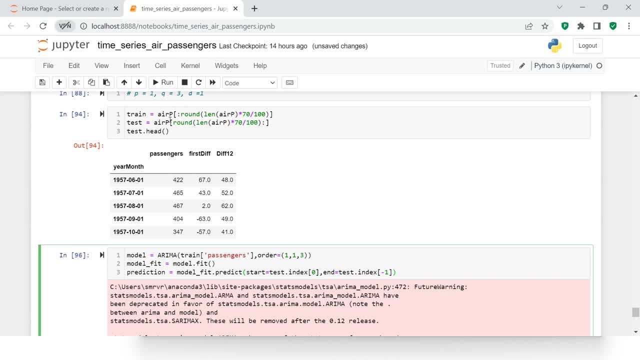 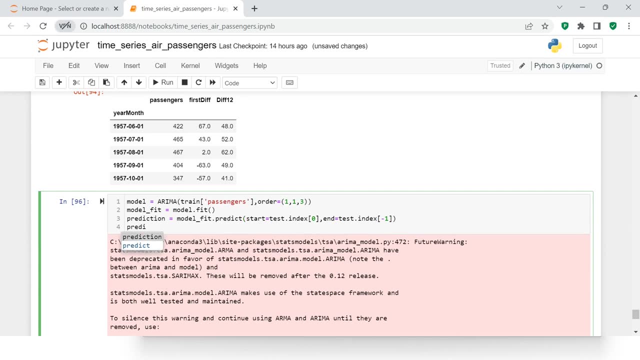 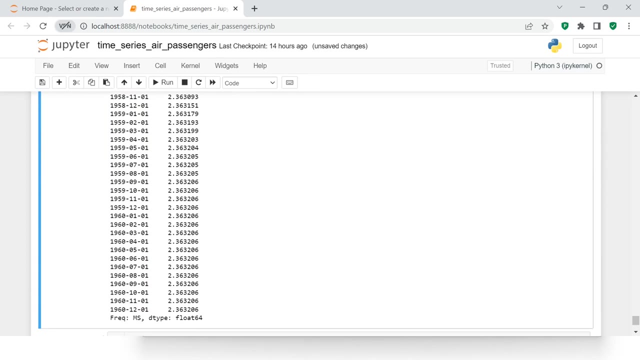 Right, The main data frame, ARP. OK, And then I'll try to plot that. So this is the prediction which is done. Let me just show you the prediction. How is that looking like? You see, these are the values. This is horrible. 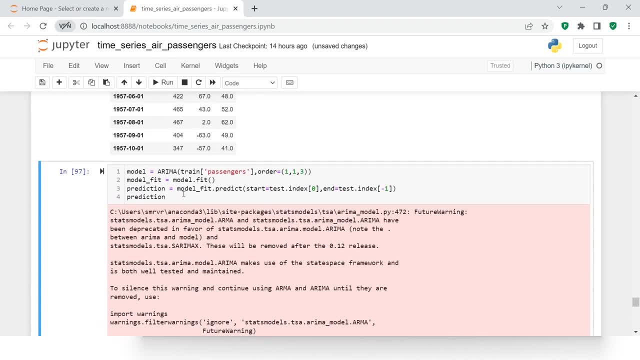 It's a Arima model is not working well on this, OK, but anyway, just let's just put it in the data frame. All right, To put it in the data frame. what we're going to do is, let's say, ARP. 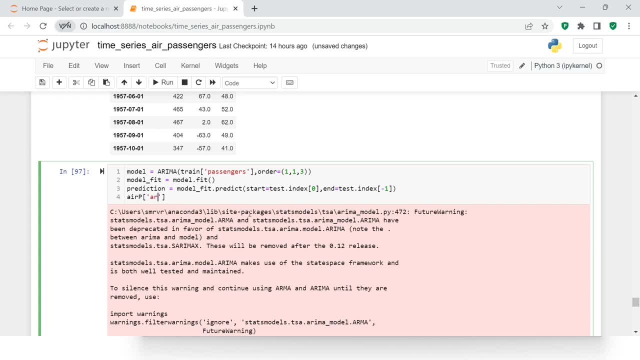 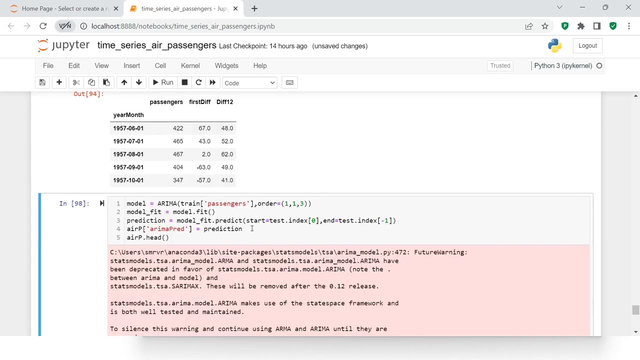 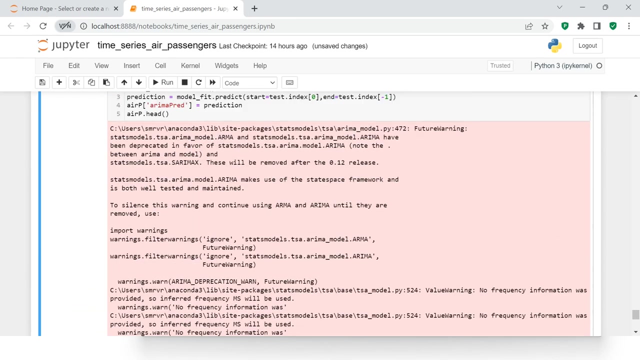 And here I would create a variable. I would say ArimaPred- OK. And here I'm just going to say prediction. Let's just put the prediction and then see ARPhead. Let's see: OK, because of the NAN, it is not showing you. 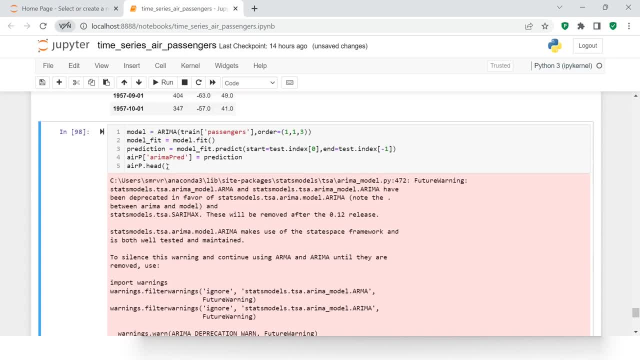 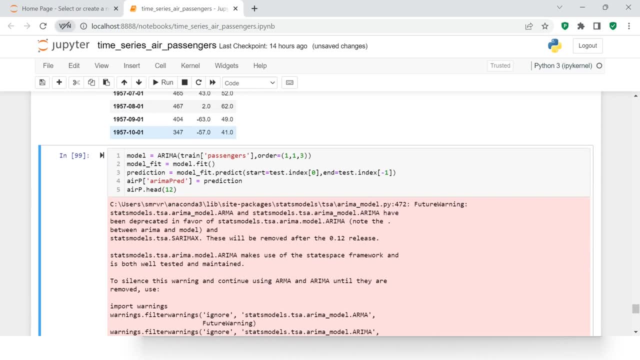 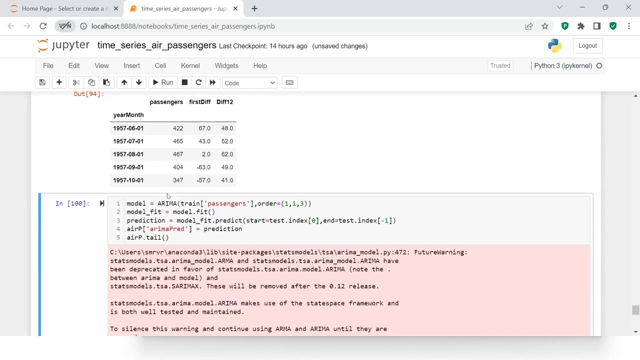 And for that reason let me just say head 12.. OK, OK, So this is the tell data, test data. so that will be at the end. Let me say tell, All right, so here is what we got. OK, now let's just try to plot this data. 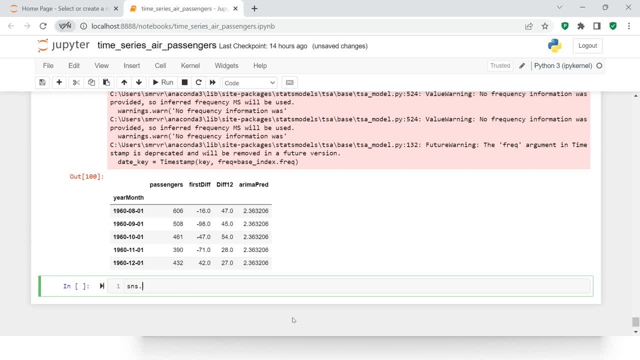 So SNS dot, SNS dot. We had created it on top of train data, Right? So let's, let's call it SNS dot line plot. And here I'm just going to say train data Data equals to data equals to train X, equals to X, equals to train dot index. 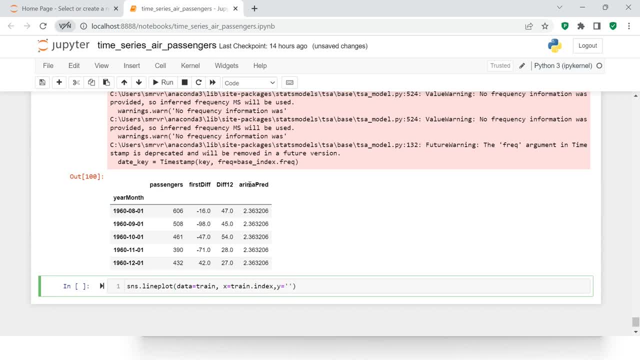 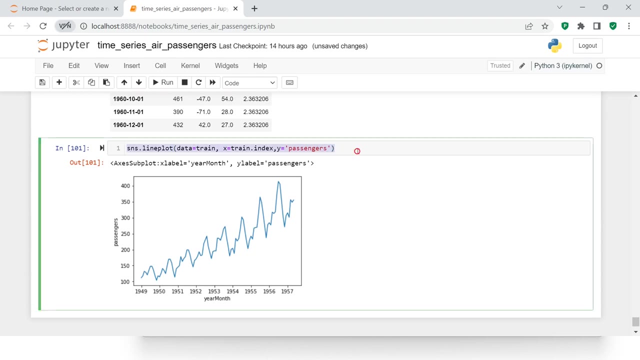 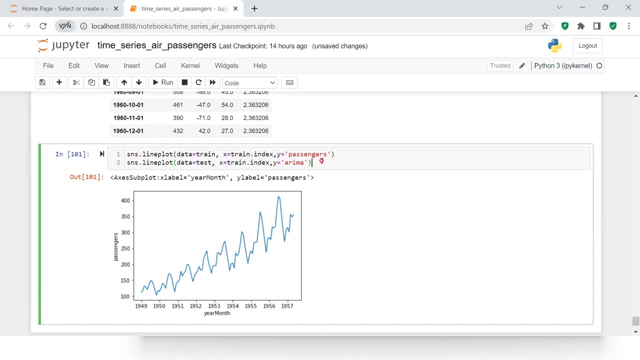 And Y equals to ArimaPred. Let's just take this. This is your training data now, because you build it on test data. So here I would say: test, here Let's call it Arima Arima. OK, To build the model. sorry, to plot the graph. what we need to do is: let's take: 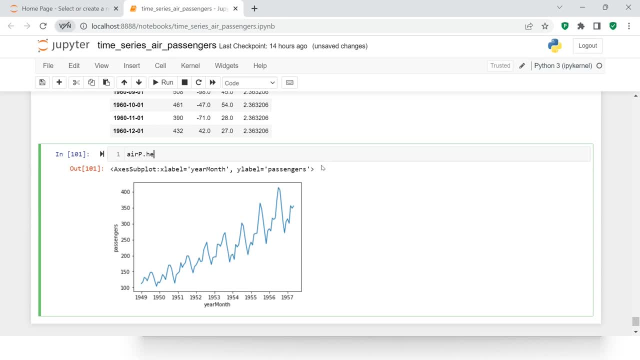 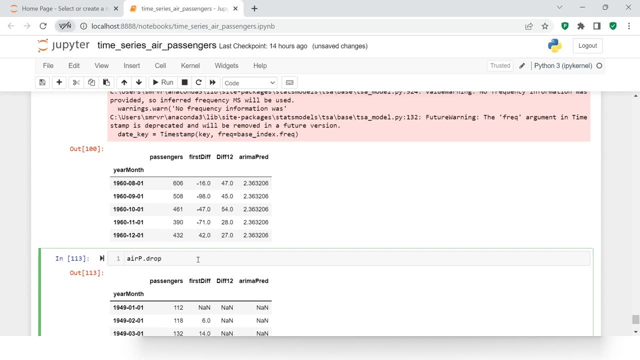 the original data frame, because in our original data frame we have everything Right And, if you see, it has any values. So what I will do is I'll just drop them. drop any, Remember this is not permanent. drop, OK, ARP. 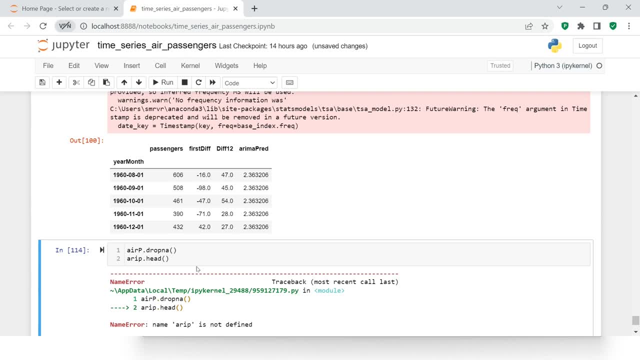 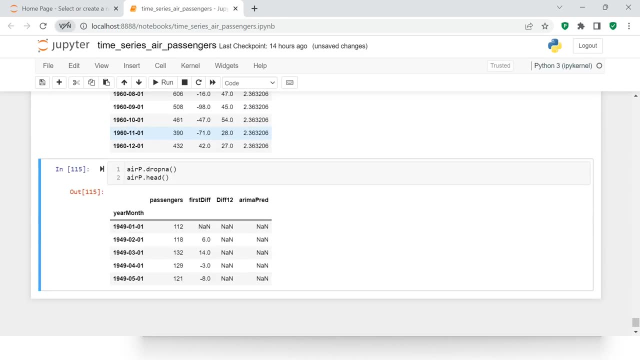 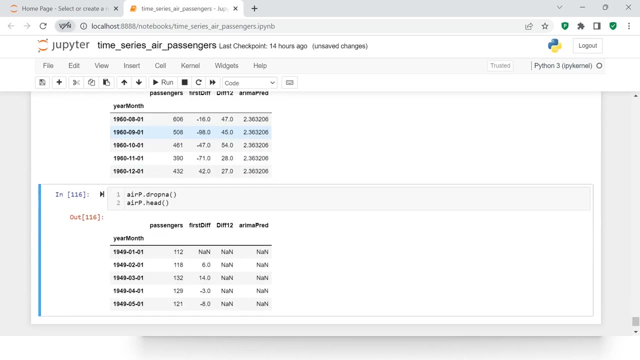 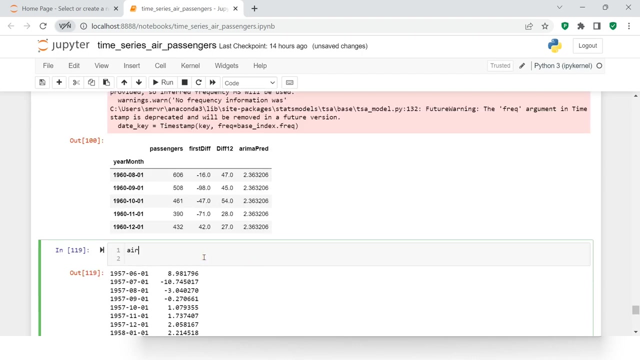 Now if you see ARP dot head- So it is going to- Sorry for the spelling mistake- Drop any. So here I will say ARP dot, drop any. And if you say in place equals true, that will be permanently removed. But at this point I don't want to do that. 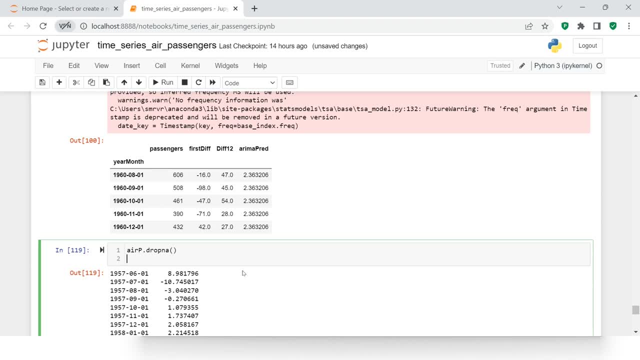 So for that, what I'll do is I'll keep it to this Right. Then I would say: SNS dot line plot data equals to ARP, X equals to ARP dot index, Then Y equals to ARIMA, this variable where we have stored our values. 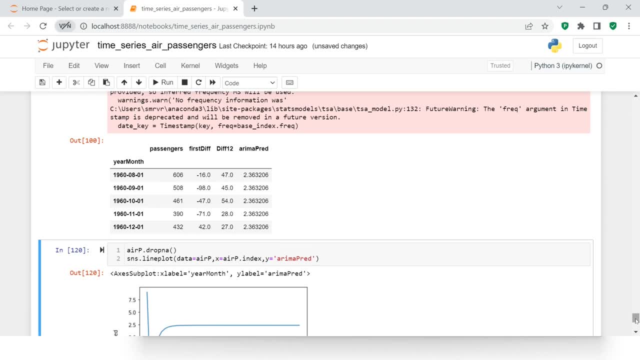 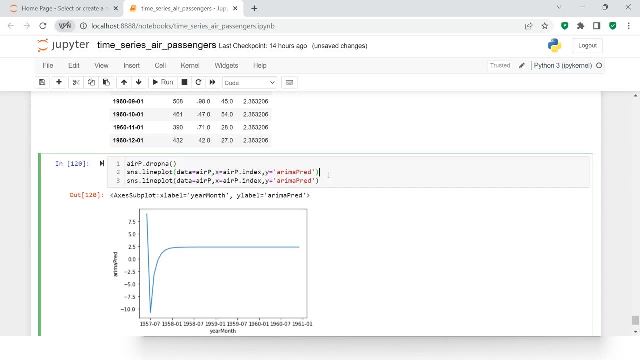 So this is what it looks like. Now let's just see how does it looks like. This is how it is looking like, But it is hard to interpret how it is doing against the actual value. So, for that, what I'm going to do is, instead of ARIMA, parade here: 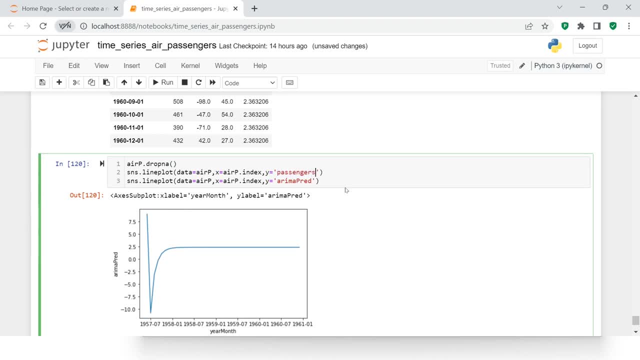 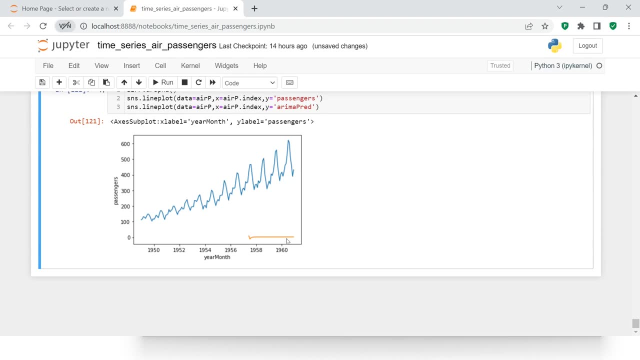 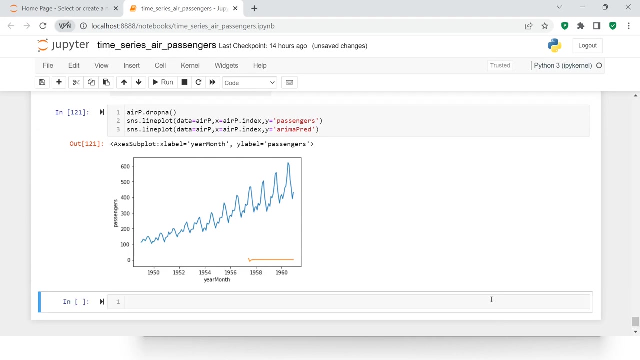 I'm taking passengers. This is what our real value is Right Now. you see the difference. You see over here it is coming. So this is the reason, because the ARIMA model is not fitting on it Right. So let's try to check the mean. 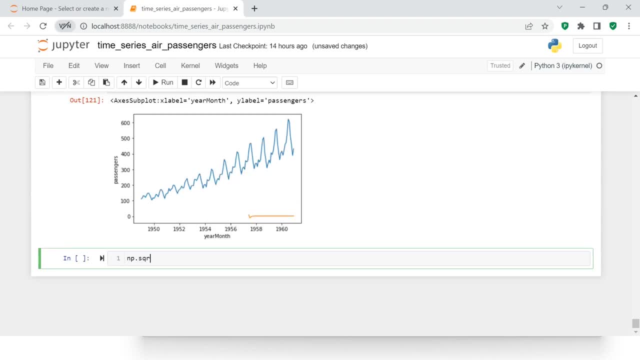 MSE. What is the error Right? So for that I would say, and the square root into this mean is error. for that You would require to import it first from a scalar dot matrix: import mean: Squared route. Mean: squared error. 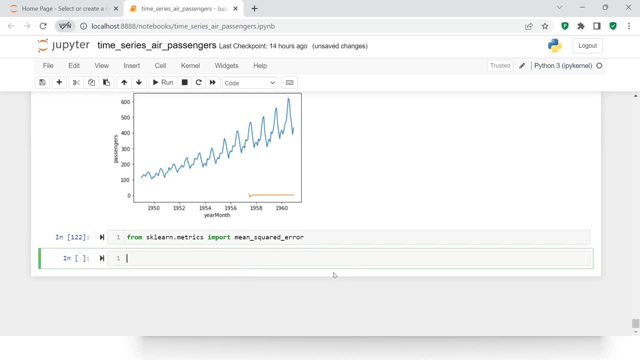 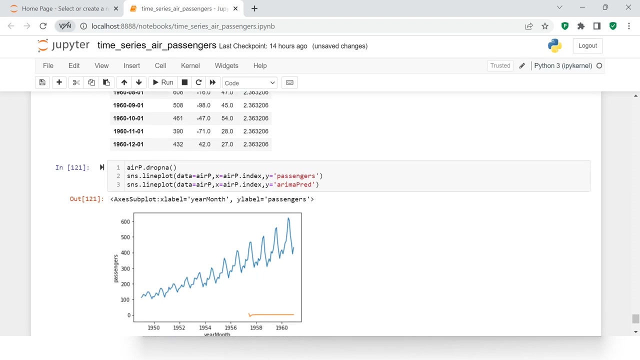 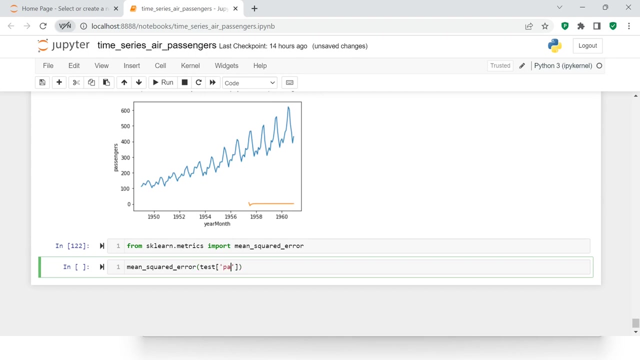 OK, this is the module which will help us to find it: Mean, squared error, And inside that I would put the value, These two values right: ARIMA parade and the passengers. OK, test data, Let's say test passengers. 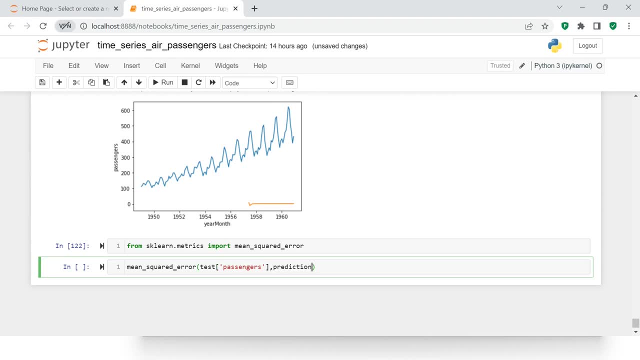 And I guess that we have created this value right Now. this is the mean squared error you are getting Now. if I do a square root for this, this is what we are getting: Four hundred and twenty seven, So this is absolutely not a good model. 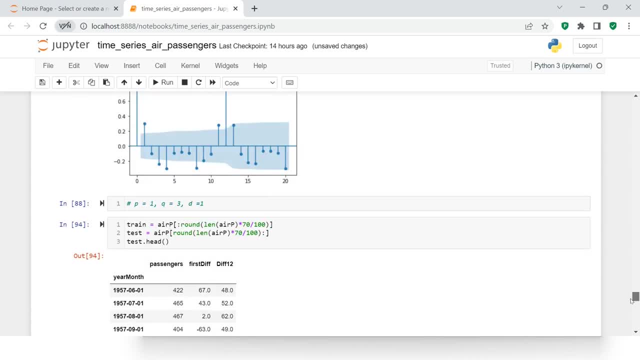 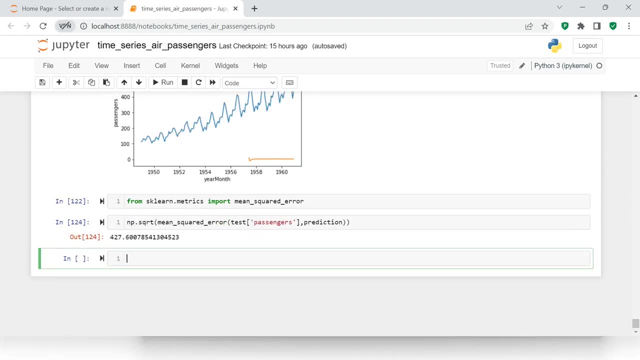 OK, so now the next step which we're going to do is we're going to see how to make it, how to make a seasonal ARIMA model. OK, All right, Now let's just start With building the S-ARIMA Max model. 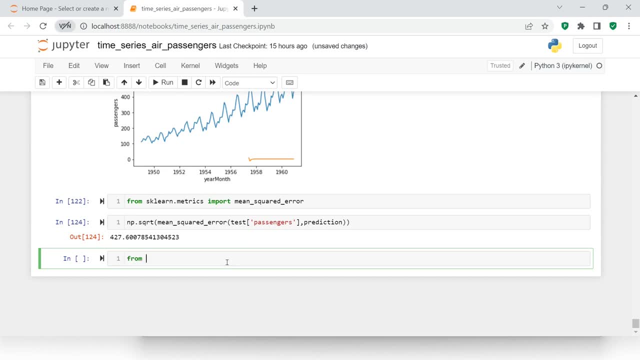 OK, so how can we import? first, We need to import that. So from statsmodelstsats space- Or maybe it should be std space- S-ARIMA Max, import S-ARIMA Max. OK, So this is done. next thing which we need to, if you, if you observe, 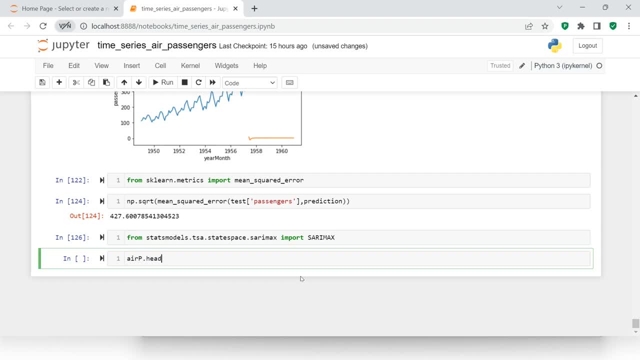 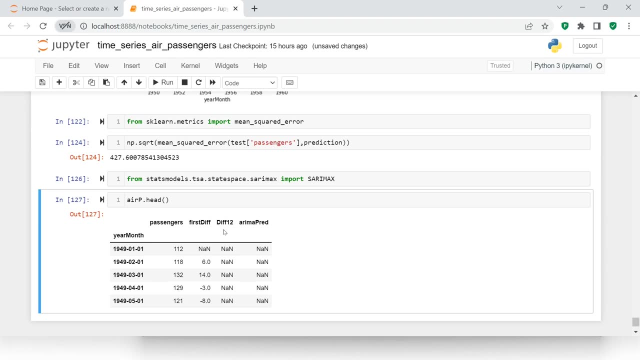 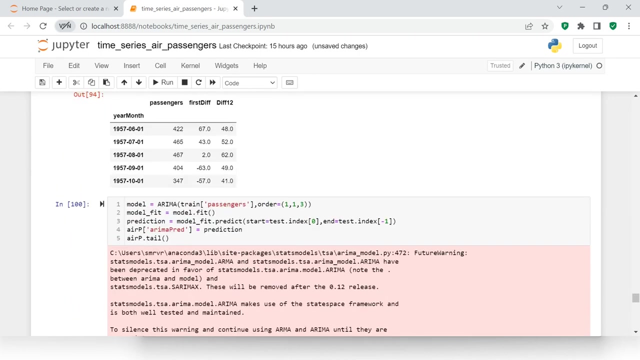 there was one more variable which we had created. If you remember that, that was diff twelve. Right now is the time when we need to use this particular one Again. we are going to find the ACF and PCF so that it will give us the value. 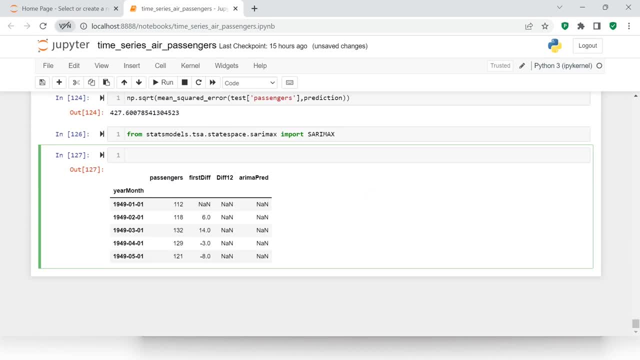 for this twelve difference, and then we will start with it. OK Now. First we need to find the value for PD and Q. OK, now, let's just do that. The value for PDQ. So first thing which we need to do is find the plot, PSCF, and in that, the data which 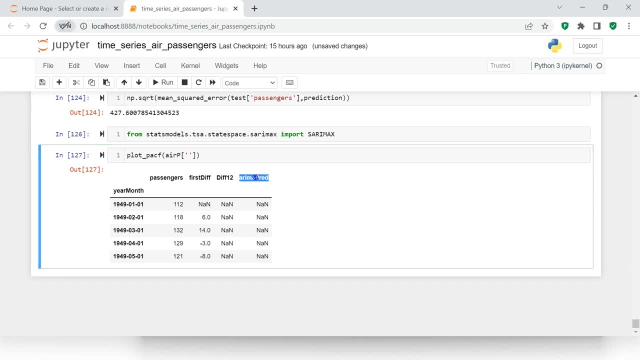 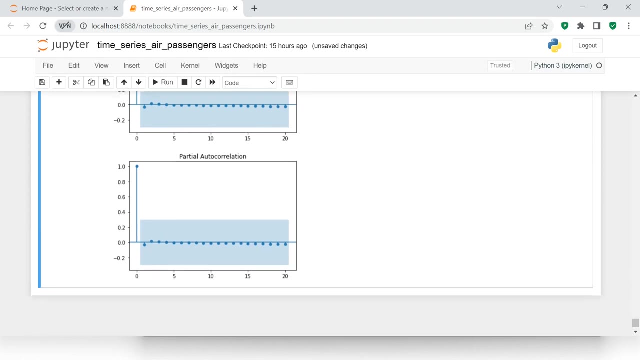 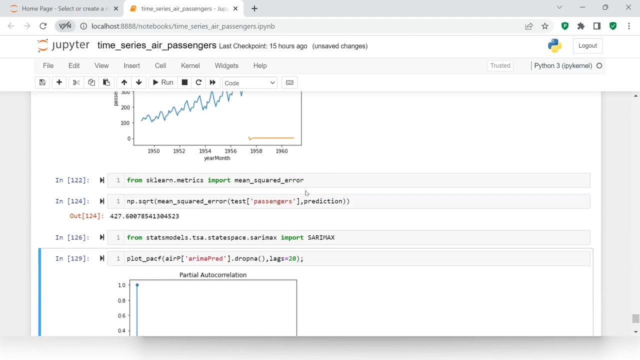 we need to supply is this, and into this we are just going to use this particular variable over here, say, drop NA and lag equals to lags equals to twenty. Let's just see All right In this. Let me just do this. 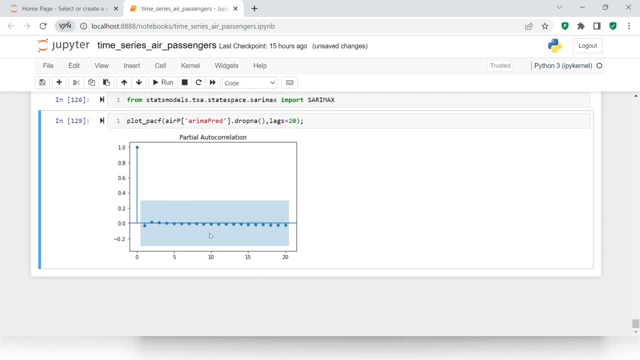 OK, so here we don't have anything going significant right, Going in significant area. So what we can do is for S-ARIMA we can keep the value for PDQ same as we keep We took it for, You know, ARIMA model right. 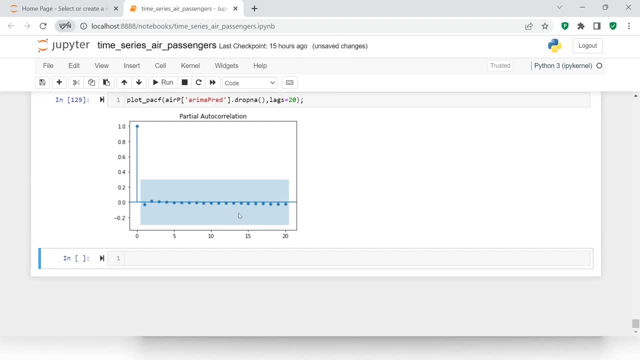 And here seasonality we can provide for twelve months. Let's start with this, Let's do that: S-ARIMA, S-ARIMAX, And here I will just say train data, Train, and then here we need to provide train passengers. 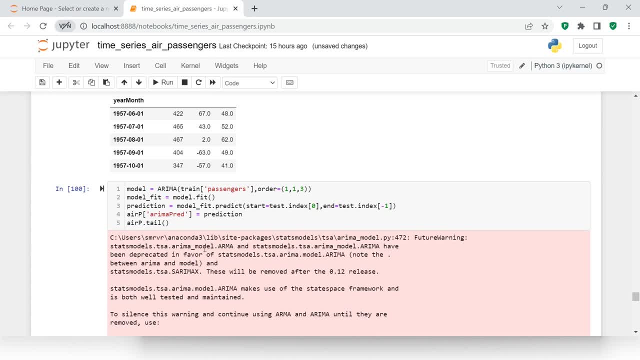 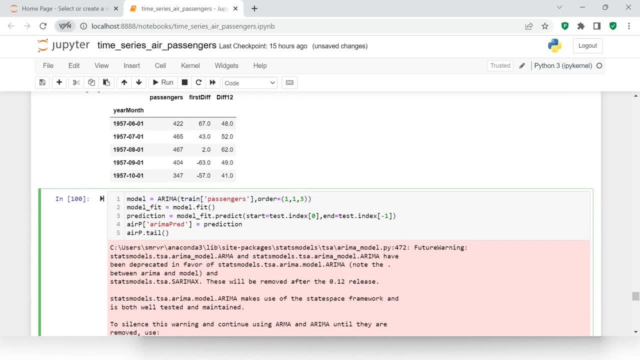 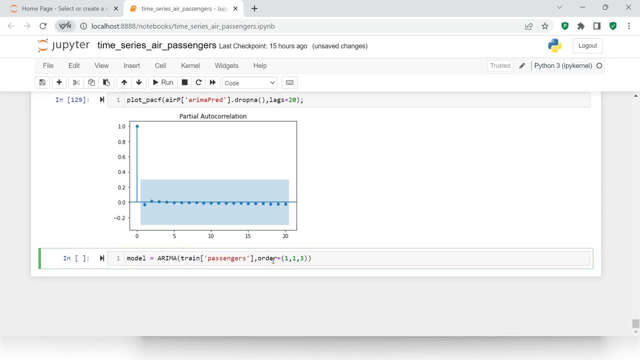 OK, let me just copy it from here itself. Whatever we had We did, I'll just take it from here only and I'll just put right away, just to save the time, and we will call it as ARIMA. Here it takes one more parameter and that is called: 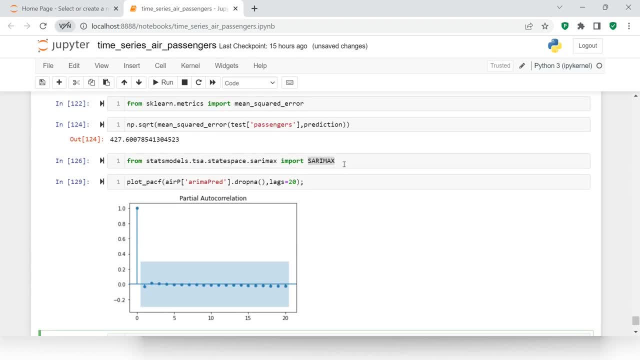 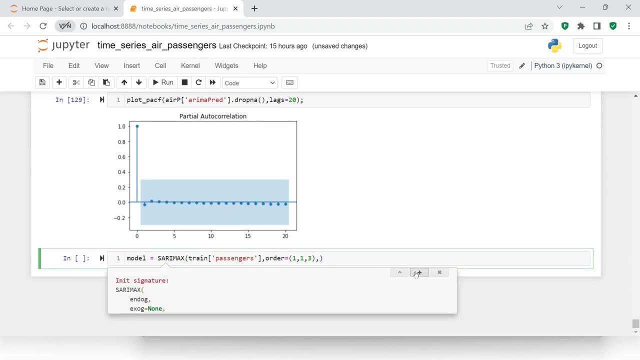 I'm sorry, here there is one mistake. instead of S-ARIMA, We need to take S-ARIMAX. OK, this is what we need to take over here. Now, if you see, the parameters which it is taking is along with the order. 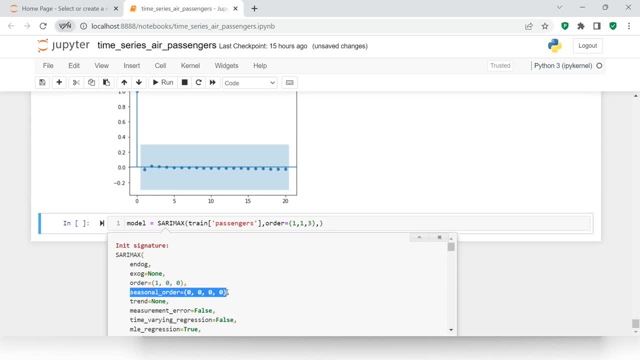 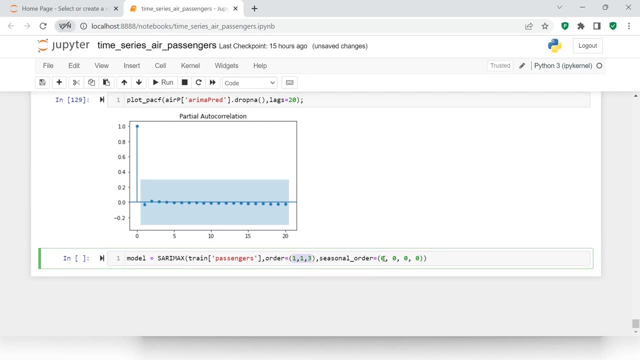 it is, it also require the seasonal order, right? So let's just apply that as well over here. So in seasonal order, these three things: it comes PDQ, in seasonal order, It takes PDQ, and over here it takes the seasonal number. 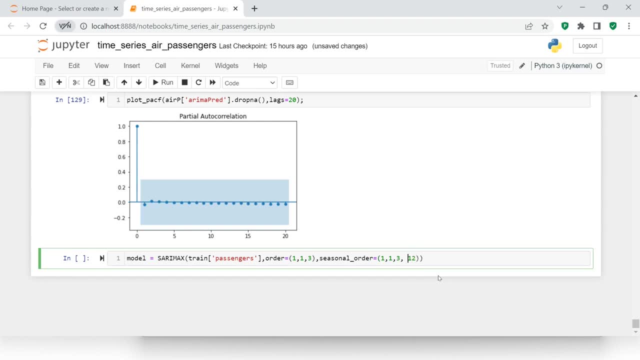 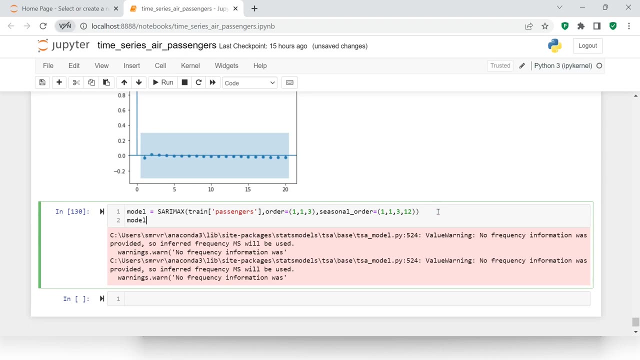 OK, so we have 12 months seasonality. So that's what I'm going to put over here. OK, now this is done. It's not giving any error. Now let's just fit the model Model underscore fit, And over here we say model dot fit. 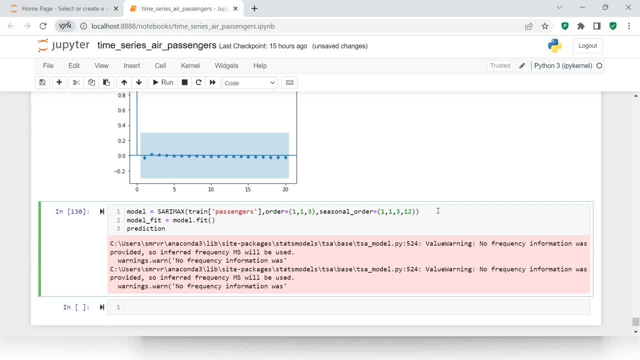 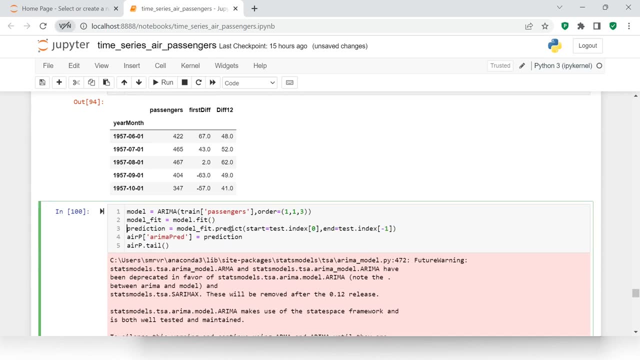 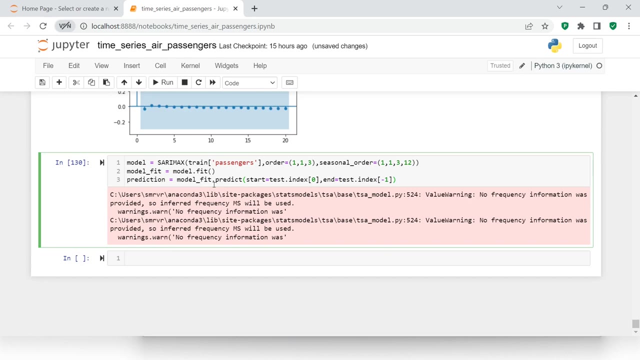 And now the time comes when we have to make the prediction, And for that again, what I'll do is I'll copy paste the things. Oops, sorry, Let me just copy Paste it So that it will save time. OK, now this is done. next, in the data frame itself: 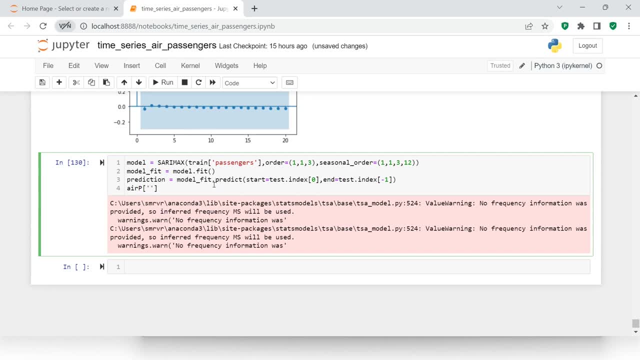 We will put this particular value and I would say 12 months, 12 months difference. If 12 months or let's call S-ARIMAX spread, OK, that was ARIMAX spread and this is S-ARIMAX. 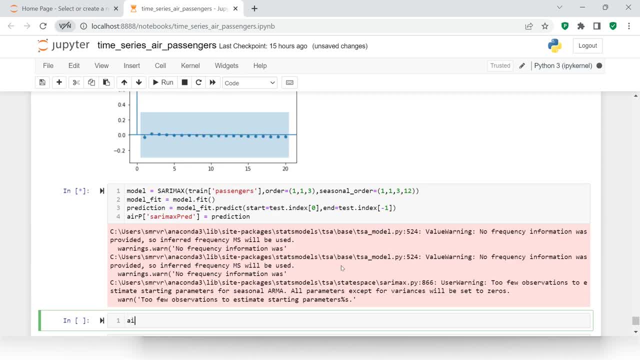 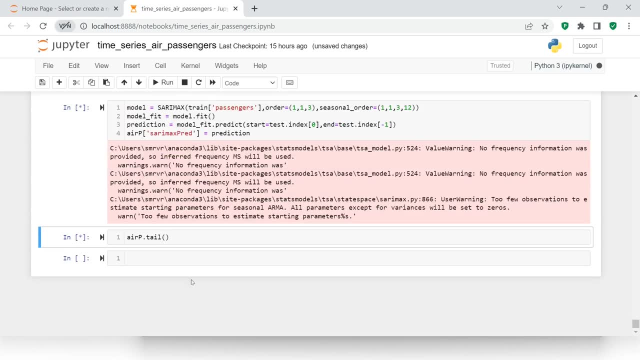 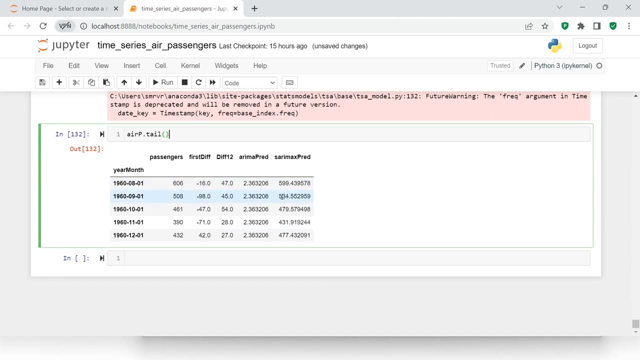 OK, this is done. Let's just have a look at the data P dot del, because that's where you're going to get the actual view right Now. here is what we have. This looks a little better right Now. let's just try to plot this. 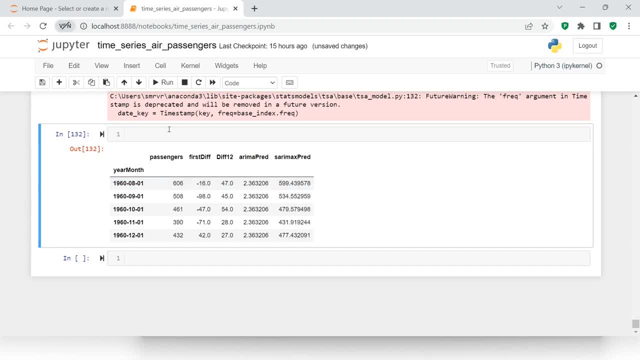 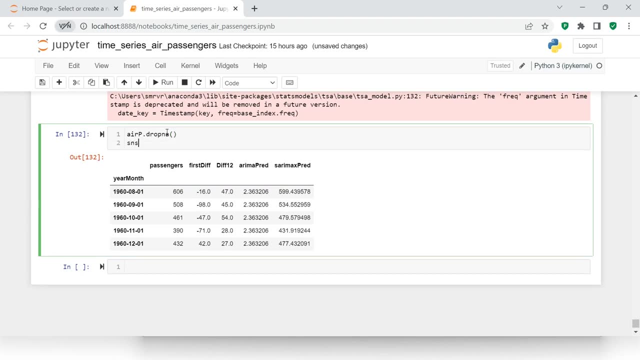 So plot there. to plot this again, I'm going to do the same thing. I would say here: P dot drop, Drop any. This will drop the data as an S dot line plot And inside that data equals to air P And from here I will just take passengers. 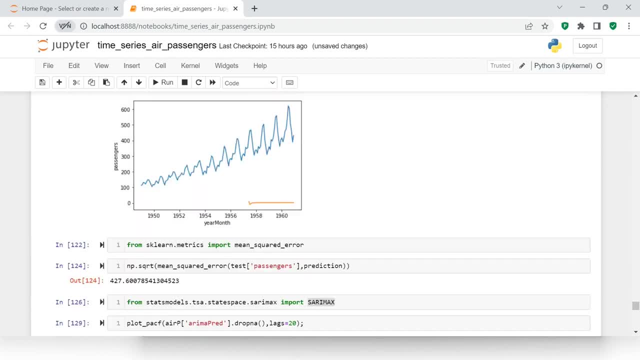 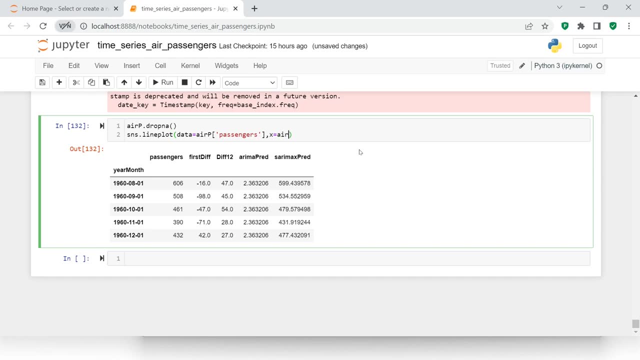 or maybe, if I can do a copy paste, let it be just passengers, OK, and over here I can use air P dot index. Next, on the Y axis, I'm going to plot this S-ARIMAX. Now, how is that going to look like? 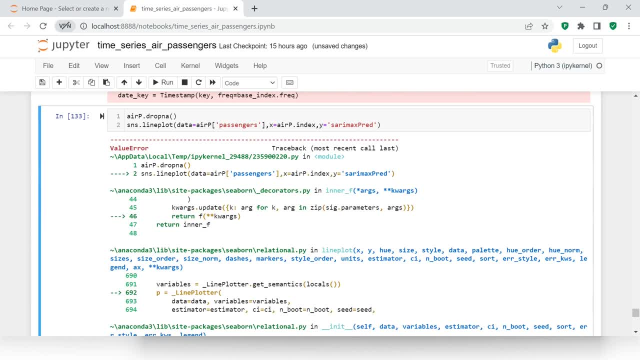 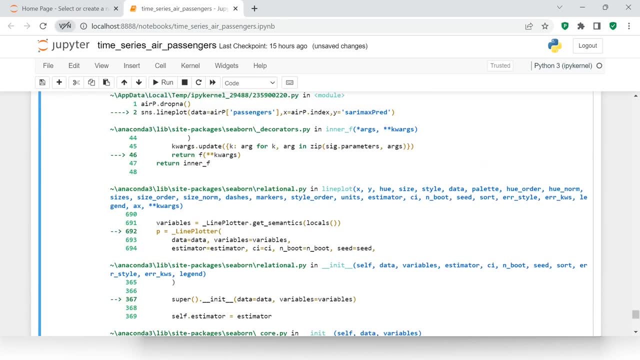 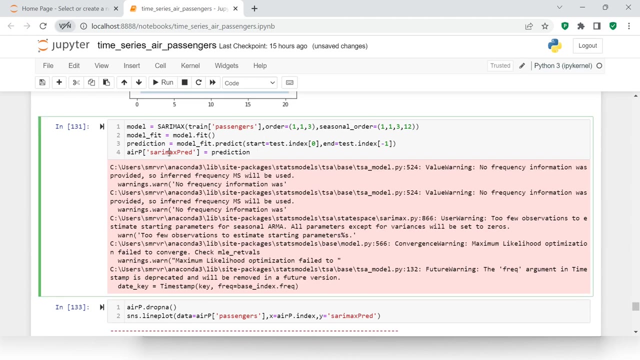 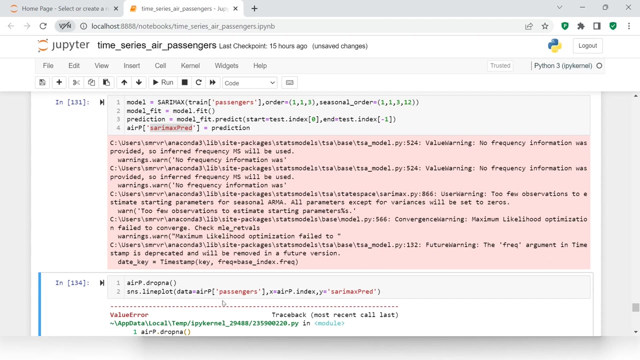 Is it giving some error? Yes, What is the error that we have? Could not interpret value S-ARIMAX spread. Why it is not able to interpret that S-ARIMAX spread. it still says there is some problem. 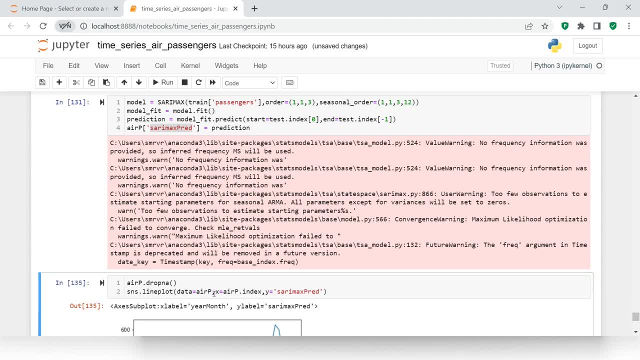 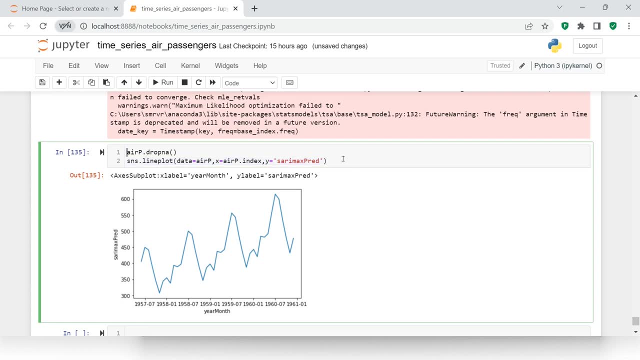 OK, so here I don't have to keep it specific. OK, I got the error right. So this is our S-ARIMAX output. Looks pretty well because it also shows the seasonality. Now, here, instead of this, I need to use passengers. 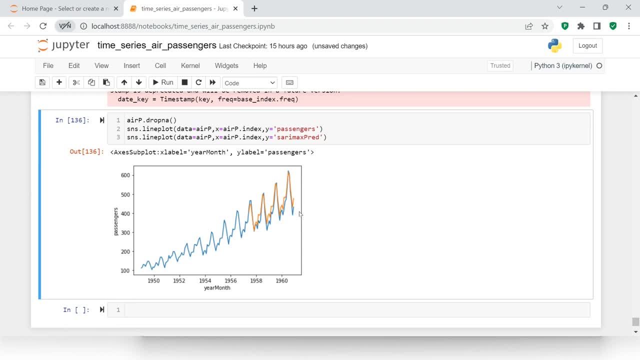 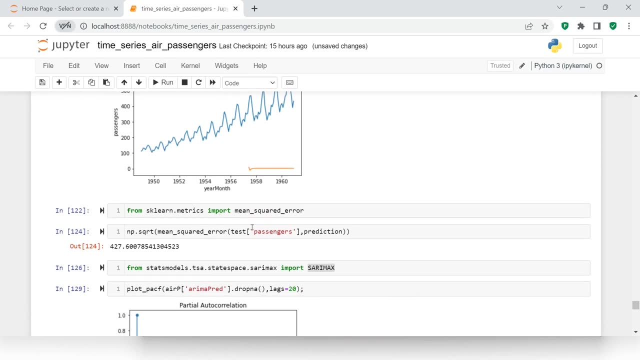 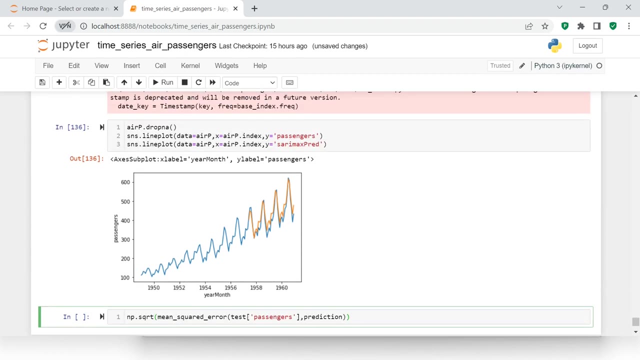 And if you see over here, this is looking following The pattern, this looks like following the pattern. Now let's find the error over here. Here we already have the function and let's just do this over here And I will put this particular variable over here. 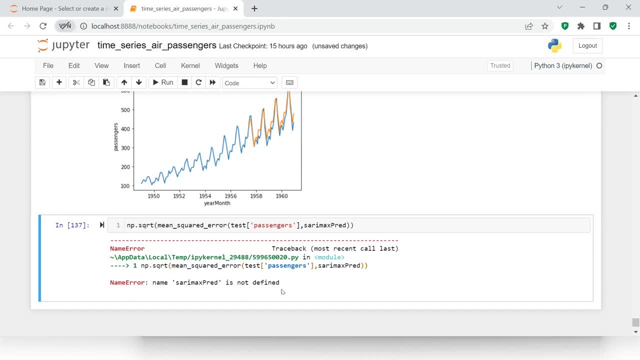 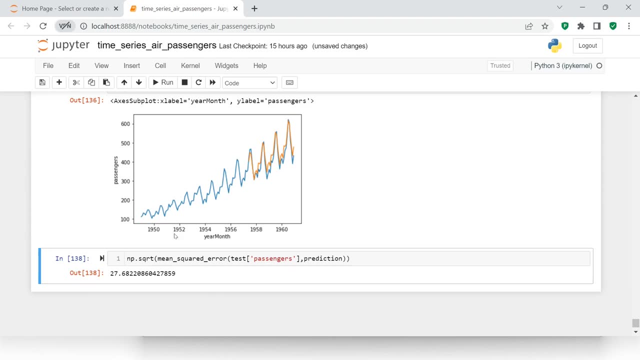 OK, again got. the error Is not defined. I have to use prediction. So here we are getting: error is 27,, which is pretty well compared to the previous one. Now this is done with S-ARIMAX seasonal ARIMAX model, which looks pretty well. 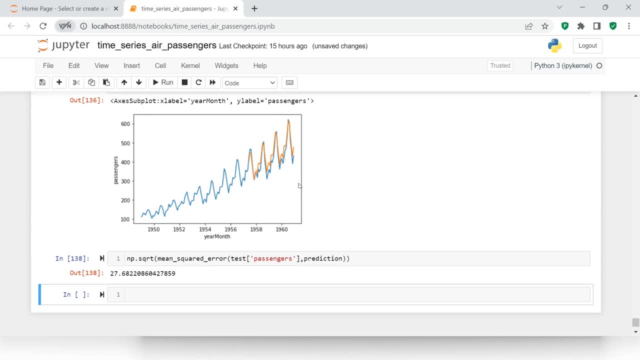 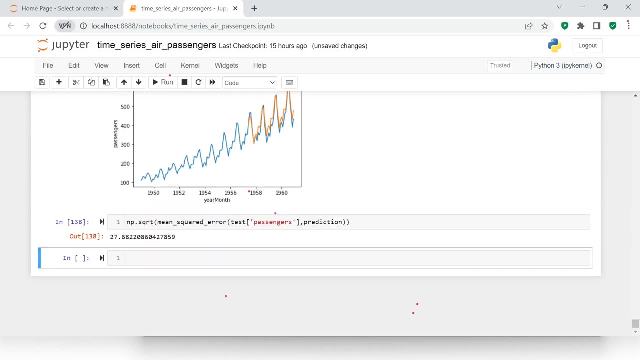 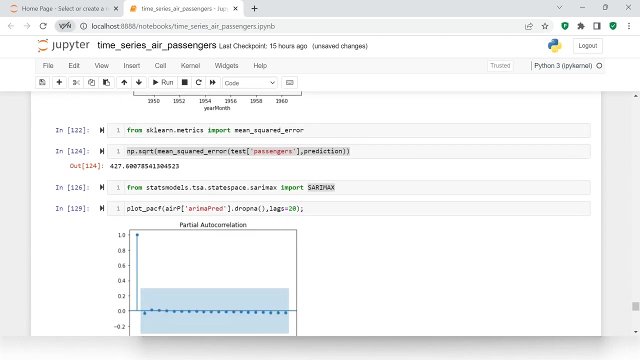 Next thing: we need to find this thing for future data right. How can we interpret this for future data which we have not seen, which is not available? Before we move forward to predict it for the future, let me have a look over here. 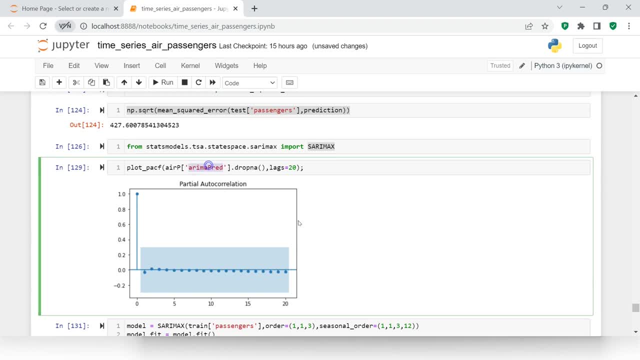 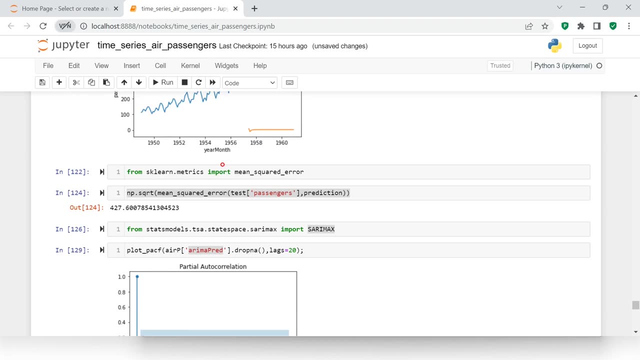 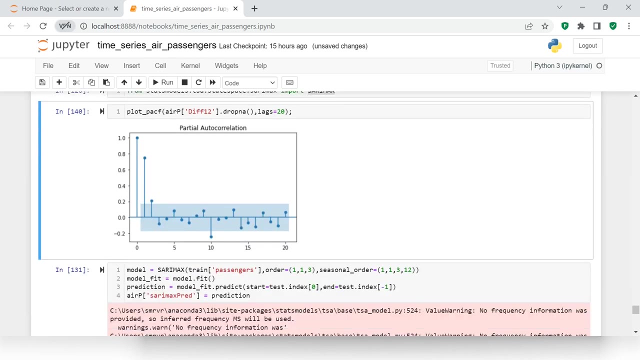 Here looks like I made a mistake here. I should ideally use the 12 month differencing variable. this variable, right? I use a wrong variable over here to find the PSEF, And so still we are not getting a bad result, right? 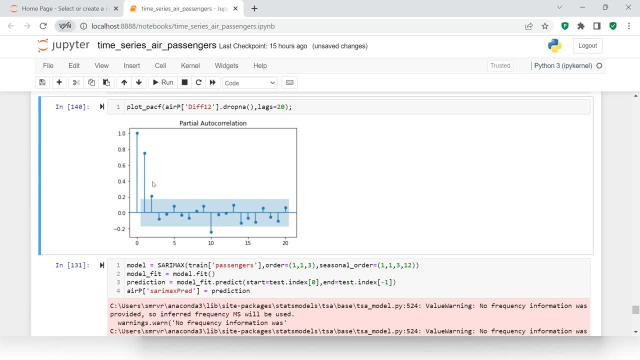 So if you see over here, here we have one and two- Both of these two are exceeding- and then 10th. one, two and 10th. So if we can, you know, use combination of both of these two. So this is for P value. 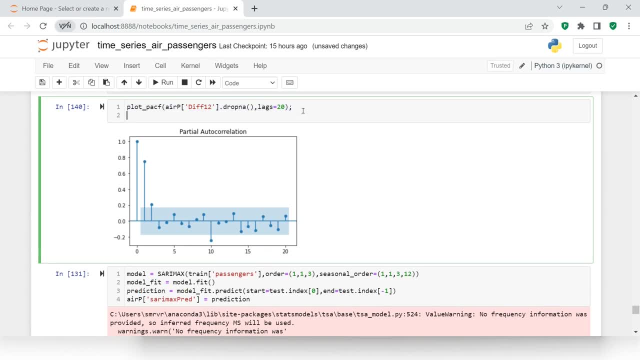 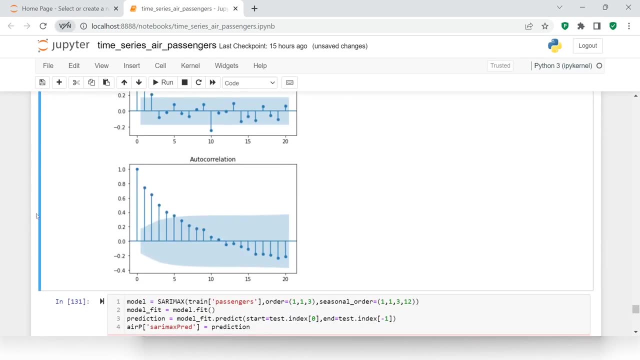 And for Q we can find. for Q what we can do is: let's make it ACF, All right. So this is looking pretty well, right? So here what we can do is zero, one, two, three, four. 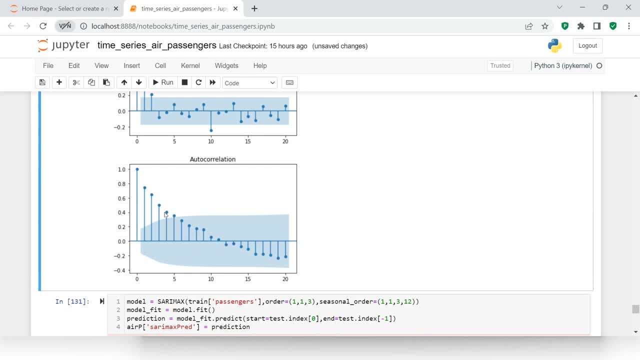 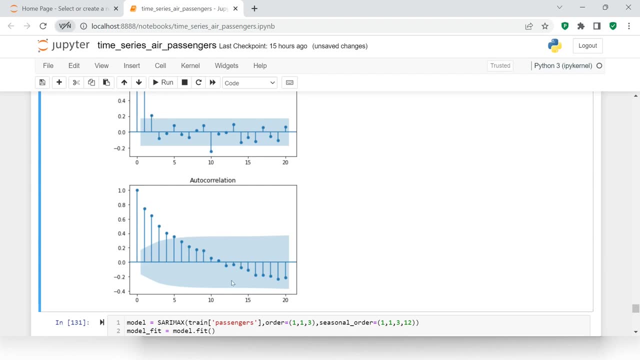 We can use all this combination to, you know, train our model in S-ARIMAX. OK, so let's just start with here. I will. I will take two, And for D it will of course be one. 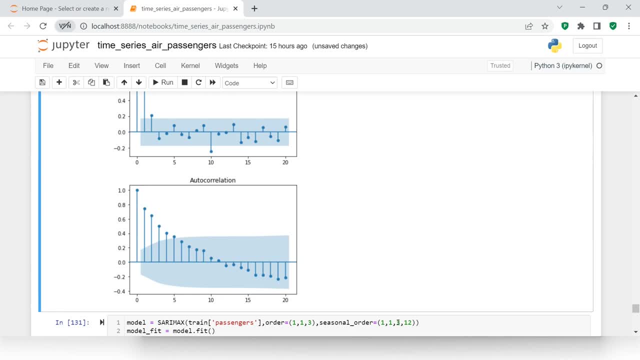 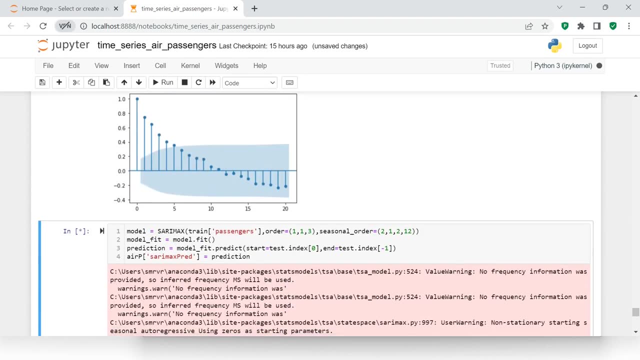 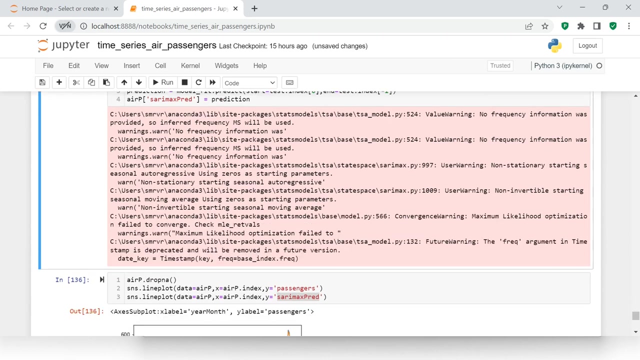 And for Q also, I would try with two. Let's try two. one, two. OK, now let's just see how the data looks like. It's taking some time to train the model Done. Then let's just see. 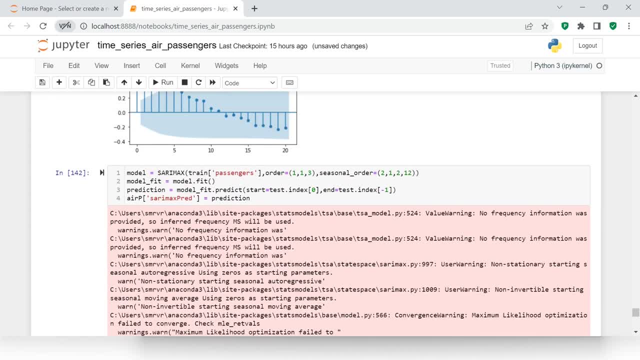 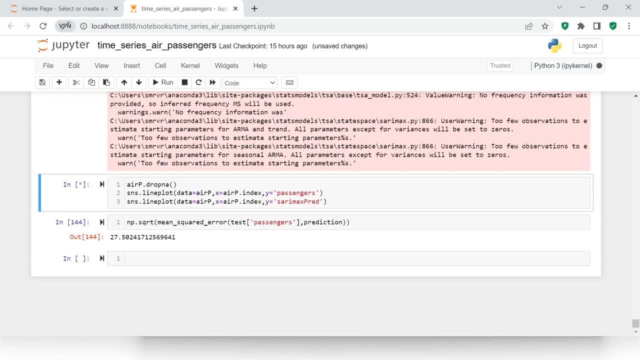 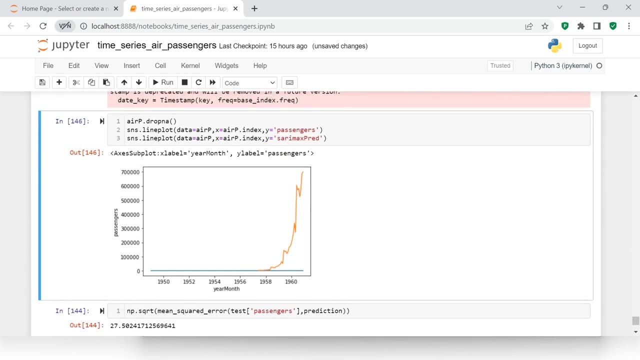 It barely puts any difference. so we are good. We are good with that. Or maybe, if you are thinking, if we can try, D equals to 12 and let's see what happens, Is there a change in the model? Oh, this is terrific, right. 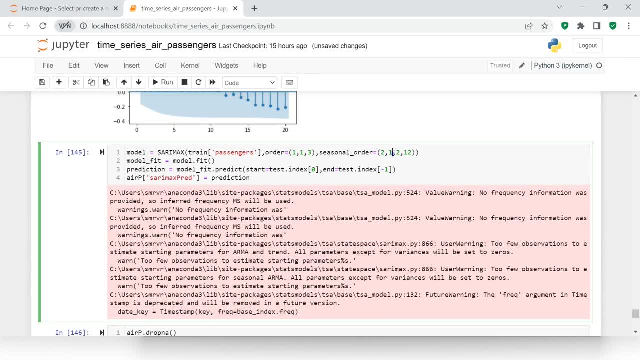 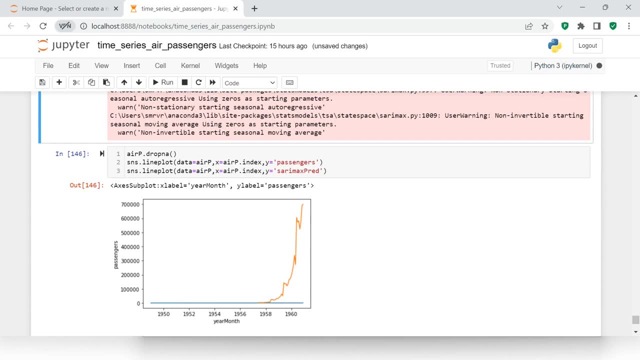 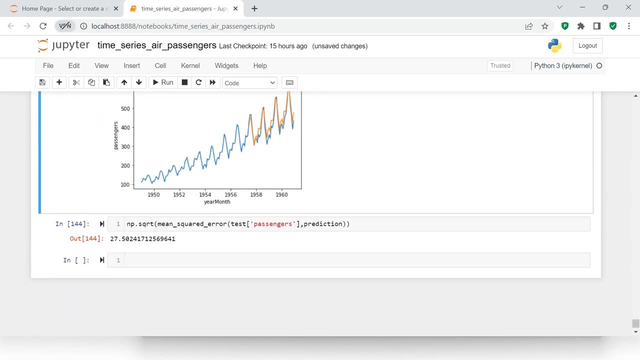 So it could. it can never be 12,, right, So it will be one. Let's keep that to one, And then over here We can try this. Now let's try to combine the ARIMA PRAD as well, right? 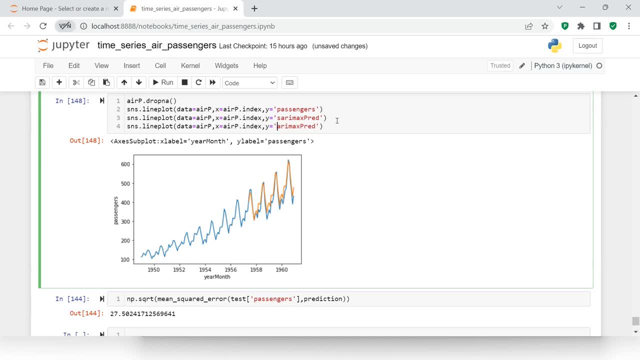 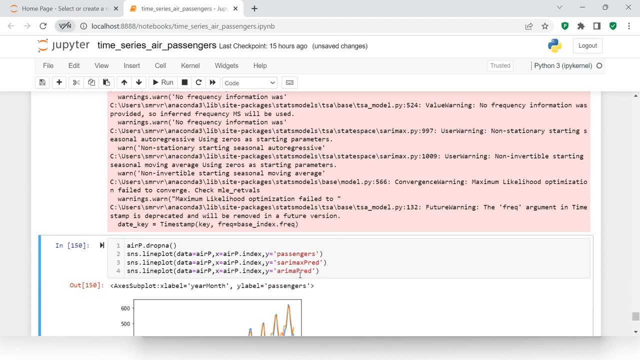 Let's try and combine ARIMA PRAD. I think this should. no, not ARIMAX, ARIMA PRAD, All right. So you see, over here, this ARIMA PRAD is looking. ARIMA PRAD is right over here. 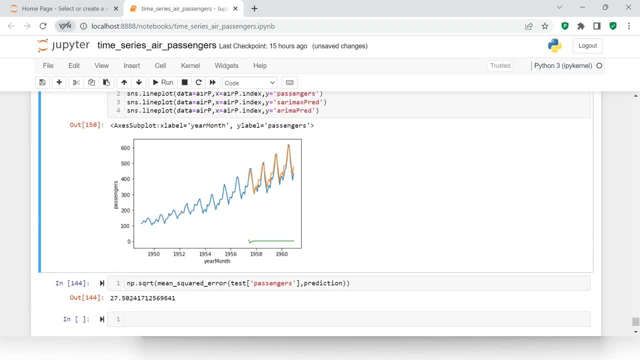 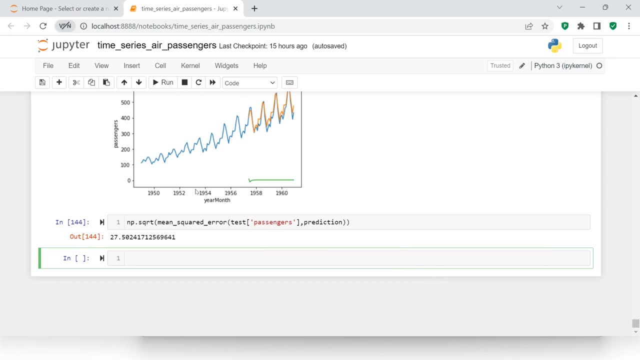 And this is how it is looking like right now. Now, to do the prediction for future, first thing which we require is to have the future dates, the data frame which we have, that has the data for which we have already done the prediction. 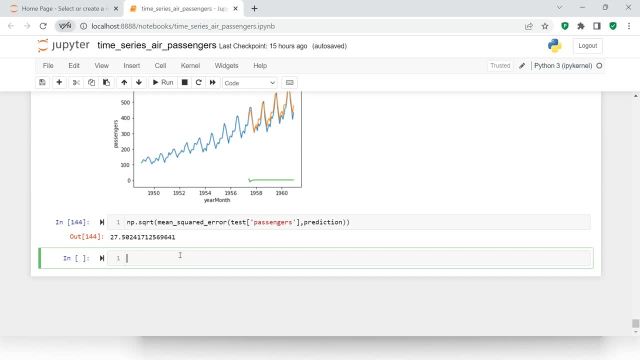 Now to do this for future, let's generate the data for future dates. OK, so before that, let's just have a look at the last date in our data, So in our data. this is our data And I will say: tell into this. 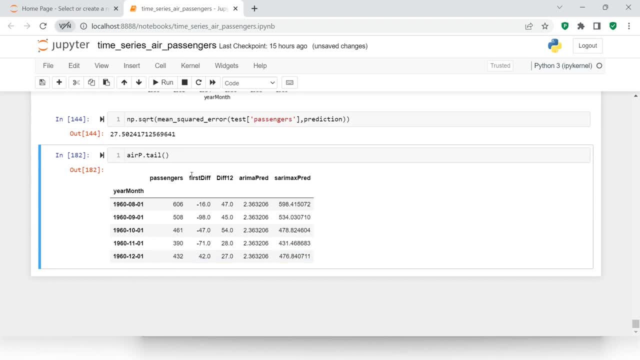 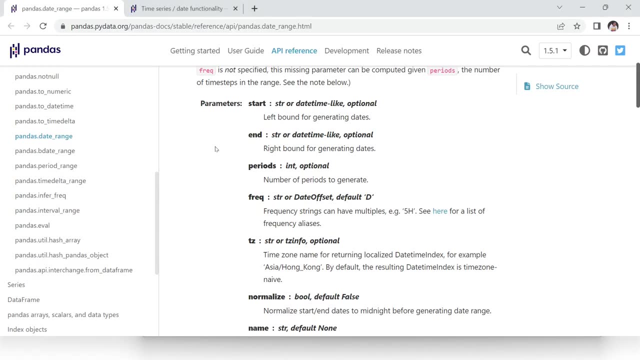 The last month which we have is December 1960. So we need to generate the date after December 1960.. How do you generate the date for future? For that, in Pandas you have one function that is called PDDateRange. 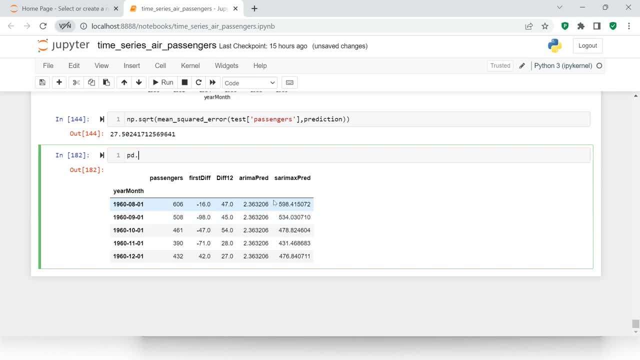 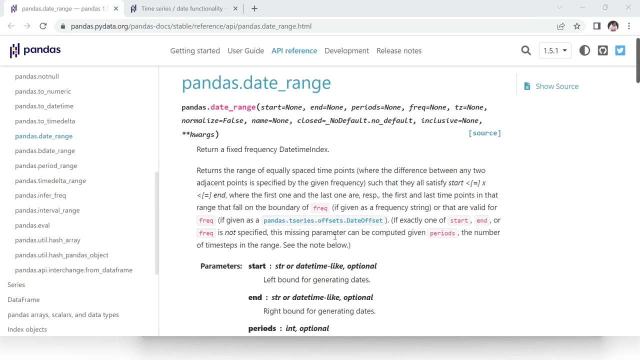 So you can use this. How can we do this? PDDateRange, Let's call it PDDateRange, And into this you need to put the start date and end date. Start will be, let's say, we will just copy this and paste it so that it will be quick. 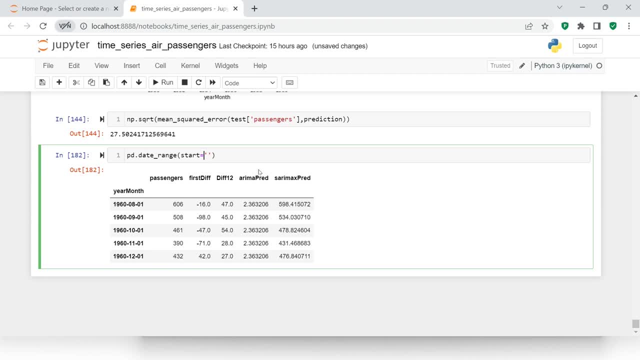 OK, let's just take this, and in this we will just change our values. So our values should be starting from January 1961.. Let's make it. I will just try to copy this, if I can. Yes, I can do this- and let's just put it over here. 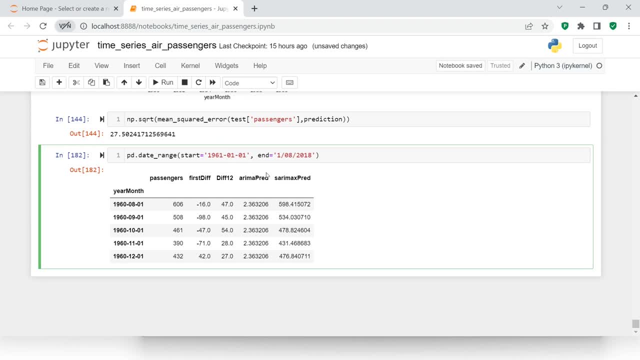 Let's just make it 0-1-1-1961.. OK, now I will make it for 24 month. OK, let's just try for 24 month, and here let's make it 12.. And this is third. 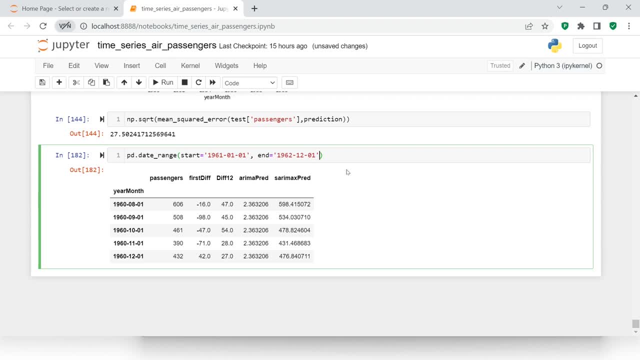 Let's just keep it till December. OK, now, at the end, If you don't give, the next parameter which you need to give is frequency. If you don't give frequency, then it is going to give you the daily dates, OK, but we require the monthly one. 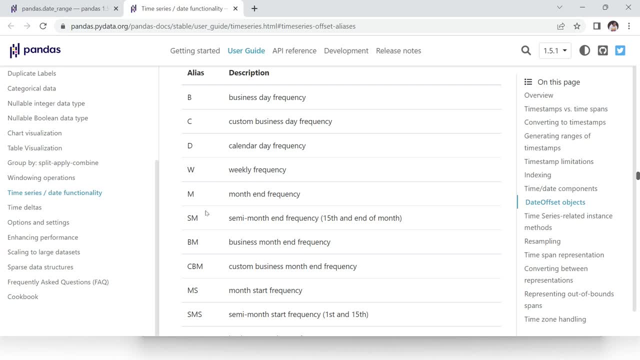 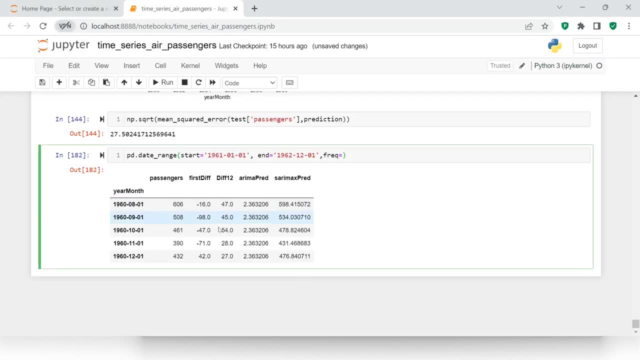 So for frequency, in here you have one frequency key which is called MS, That is, month start frequency. OK, because we have the starting date of each of the month. So here I'm going to say MS. Now let's just see. how does it looks like? 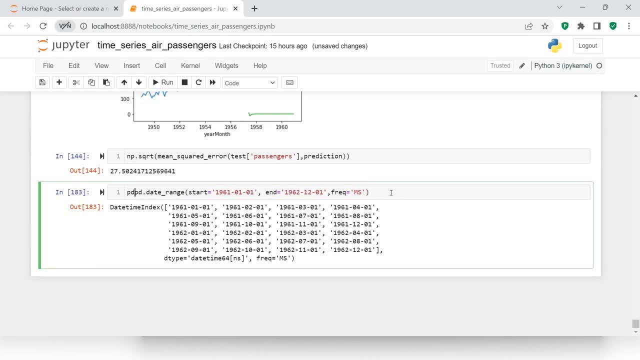 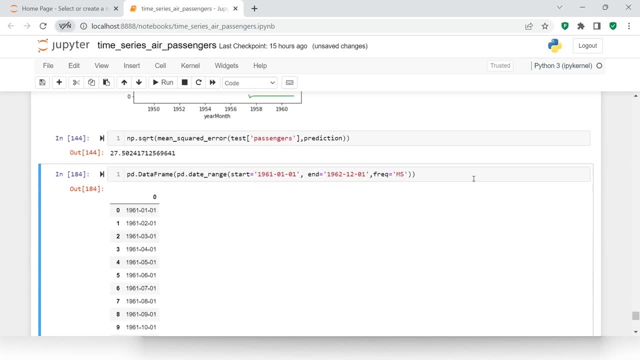 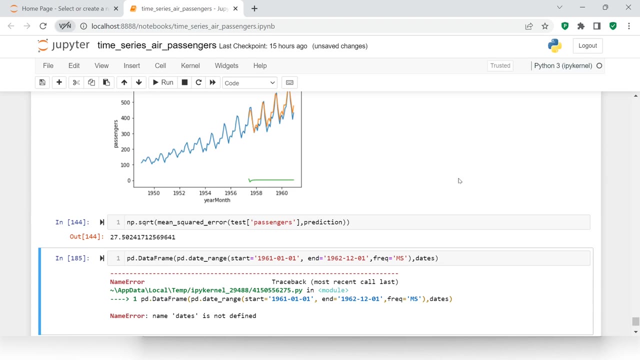 OK, we got it. OK, now let's just try to convert it to Pandas data frame, PD data frame. And here we go. Here we got it. Now let's just make it. let's call it dates, OK, column name. 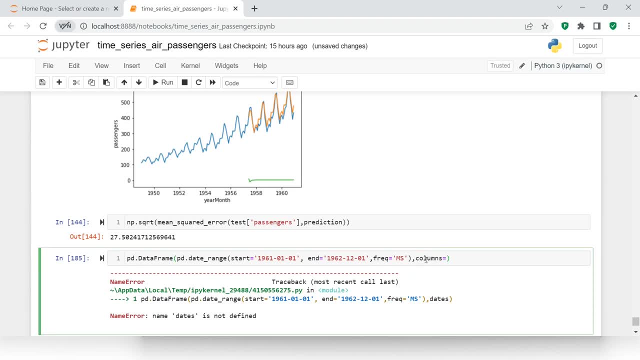 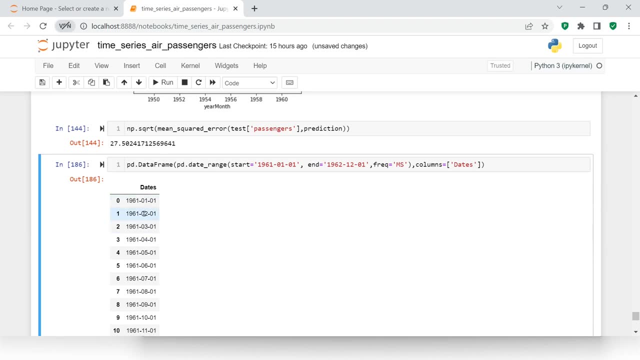 Sorry, I need to say columns, And over here let's call it dates. Now we got this. next thing which we need to do is I will just set it as index, OK, To make it simple. OK, first let's put it inside a data frame which is future date. 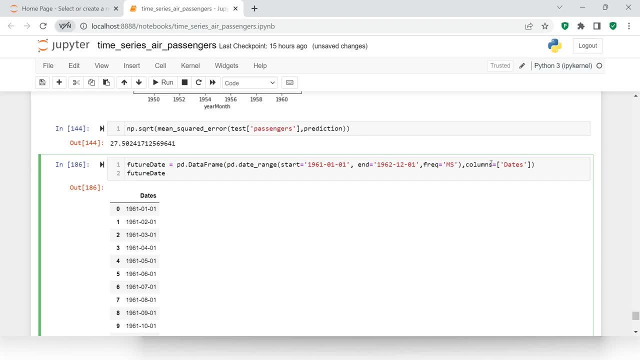 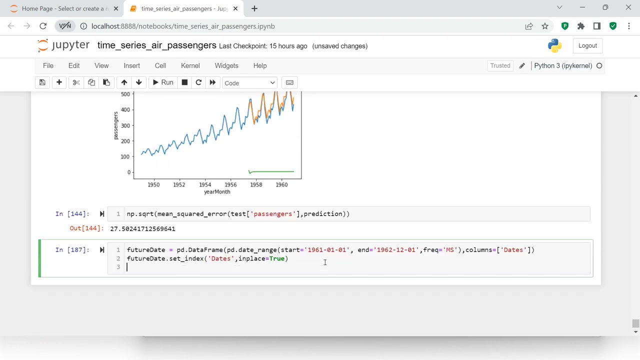 Let's call it this future date. And then I would say: dot set index, set index. inside that, the variable which I want to set as index is this: and in place equals to true. Now let's just see. how does it looks like: Future date, dot head. 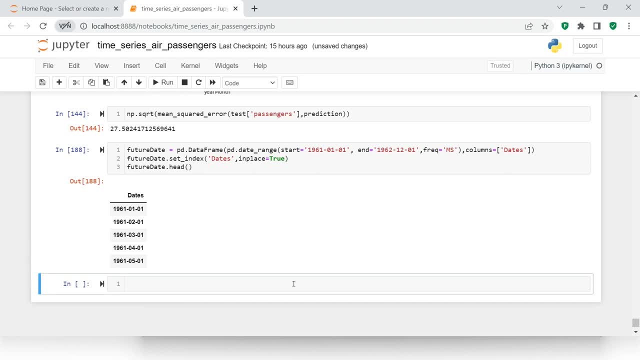 All right, so we are done with this. Now let's try to do the prediction on this. OK, so for prediction we have our model created, dot predict, and in this we need to provide this start, which will be start equals to, we can say, future date, dot index. 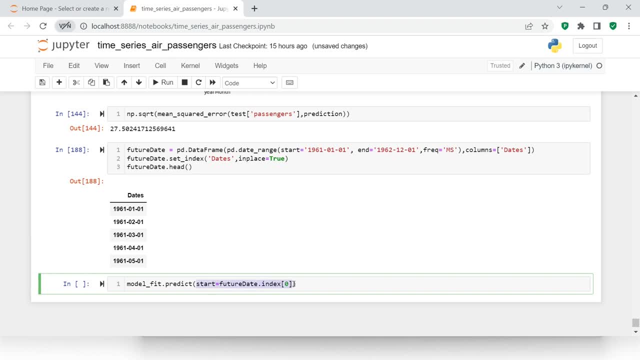 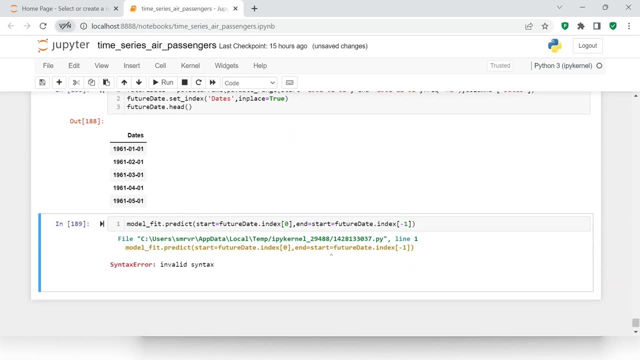 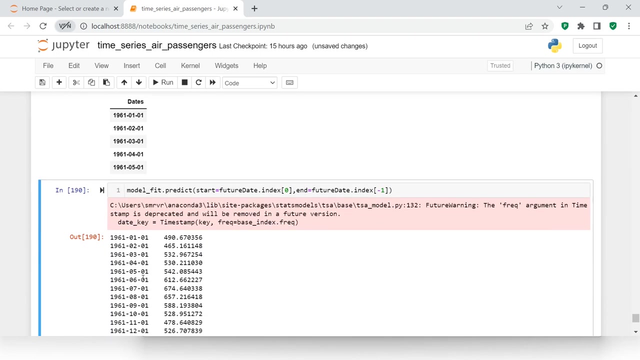 And the zeroth value, that is the start date, And then for end we're going to say negative one, And it says invalid syntax. Here is the problem. Now, here we got our values predicted. OK, this is the predicted value. 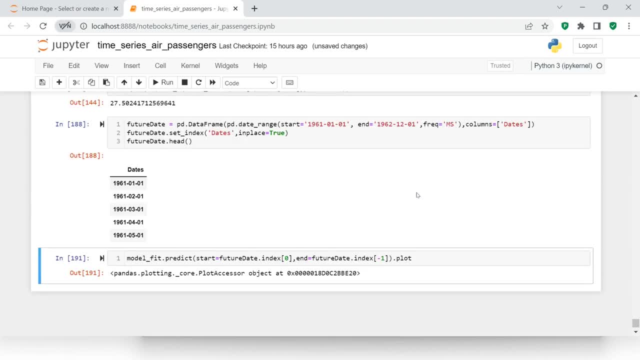 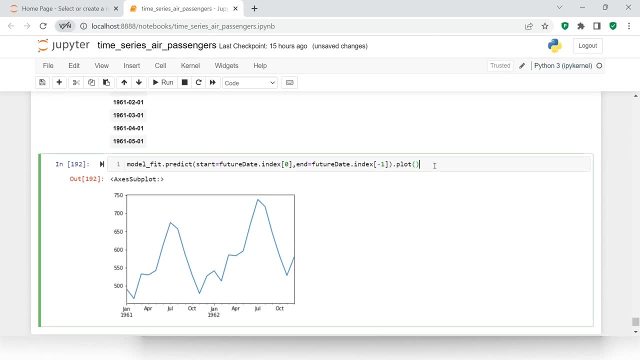 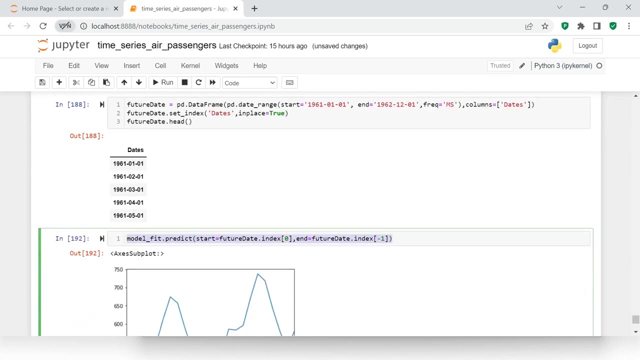 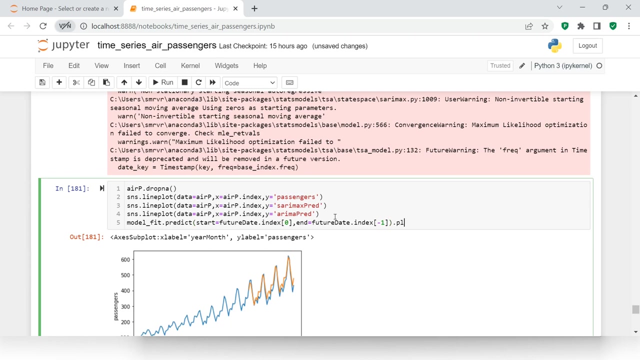 Let's try to plot this dot plot. All right, so this is how it looks like. Now, what I'll do is I'll store this value. OK, let me take this from here and here. we already have this created just along with this. I'm trying to put this: how does it looks like? 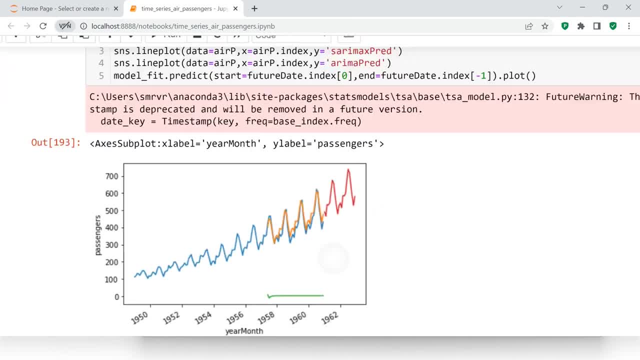 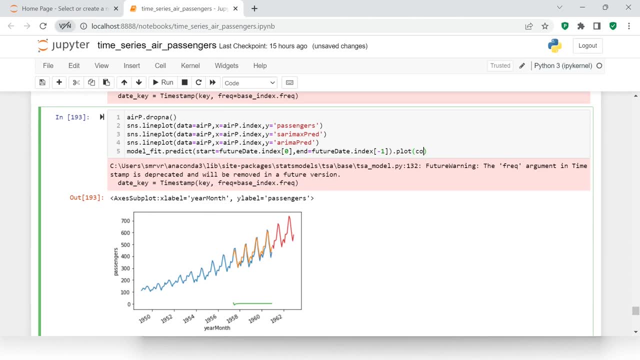 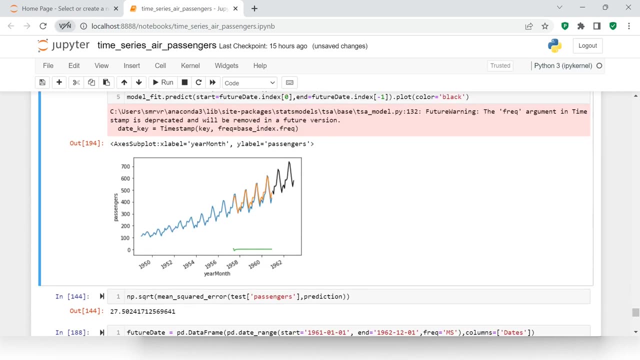 All right, so here we got that. So you see the red line. OK, if it is not looking pretty clear, So let me change the color. color Equals to black. And now let's run this. So you see, this is absolutely in sync, right? 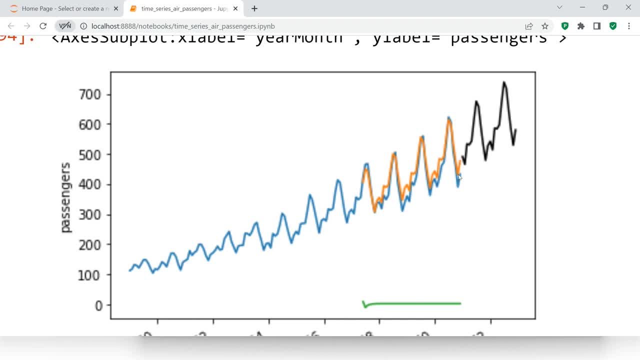 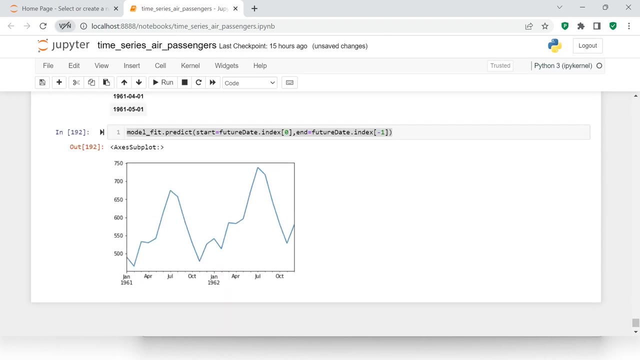 This is absolutely in sync. Till here, our data, our actual data, ends this orange line which you see. that is the prediction on test data and this is the prediction on future. So this is how you can play around with the models. You can try different values for PD. 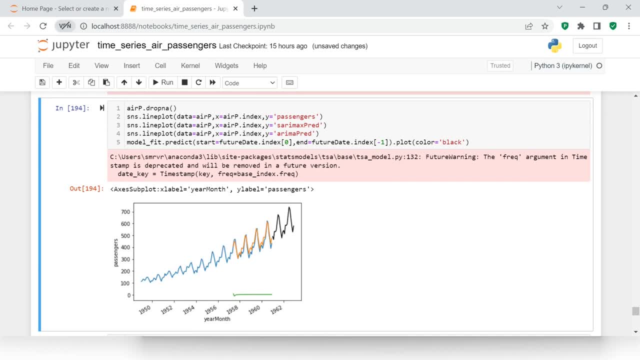 Q while training the model and you can have a very good model. All right, So this is it in this video. Moving forward, we will try to build the model on. you know, transform data, the data which we transfer to make it stationary. 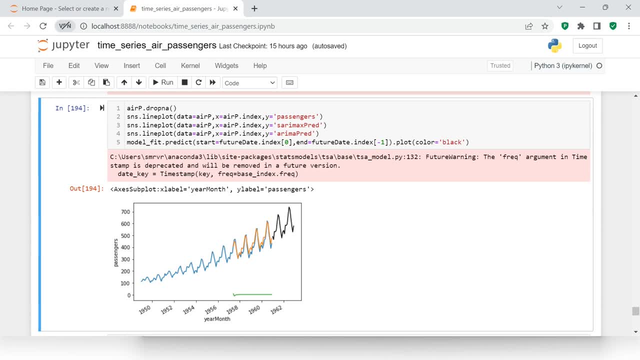 We will try to use that and make the model on top of that. Let me know in case of any confusion. try to put that into the comments section and then we will see it further.